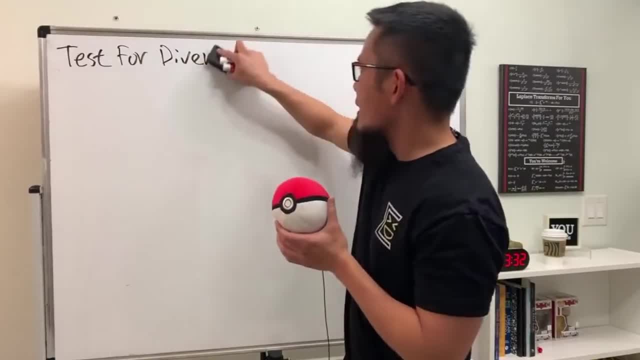 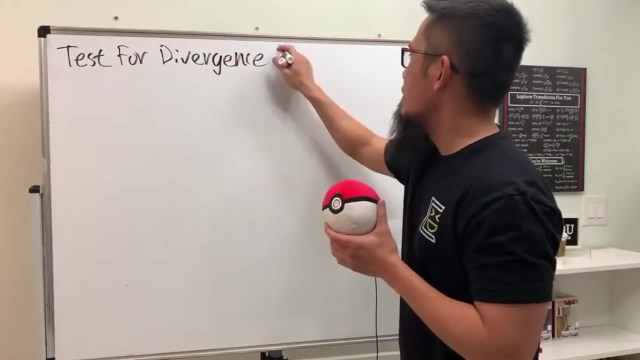 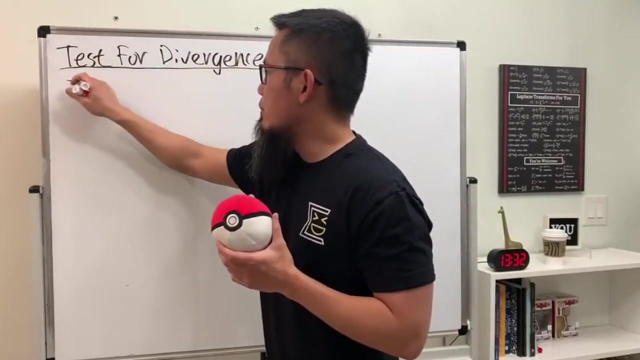 between convergence. We are going to compare the difference between the convergence between a sequence and a series. right, So this right here, a brief idea, is TFD and it says the following: all right, This right here is really useful. It says: if today you take the limit as n goes to. 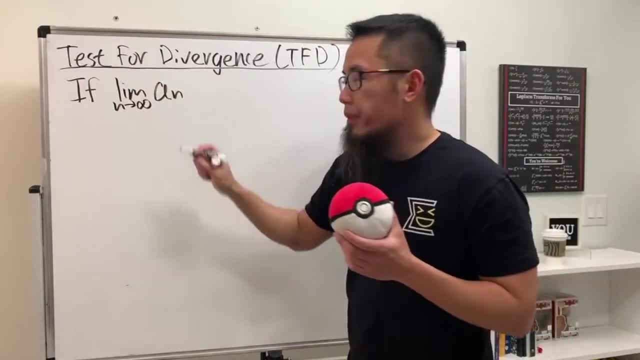 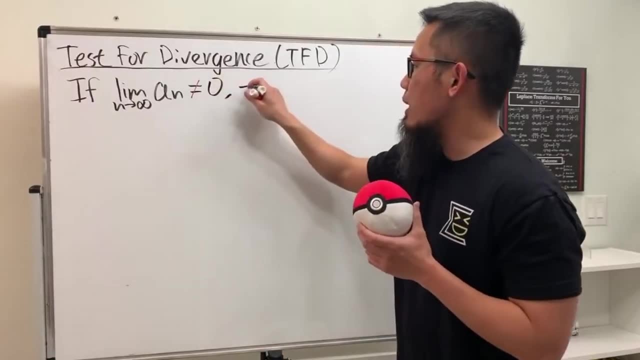 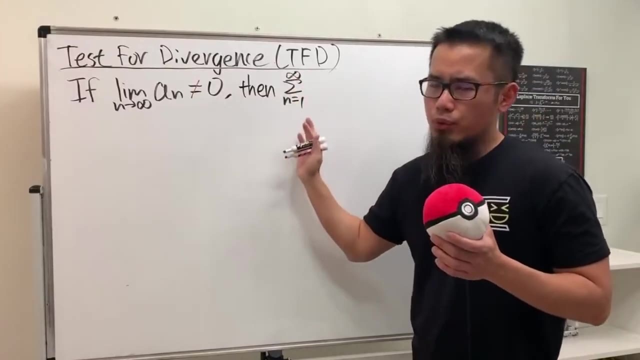 infinity of the sequence a, n. well, if this right here is not equal to 0, then you can be super happy, because you get to compute that the series as n goes from 1 to infinity, And in fact the starting n value usually doesn't really matter, but as long as you go to infinity, and then right. 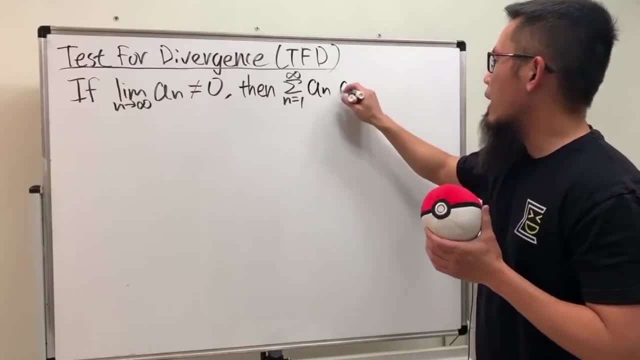 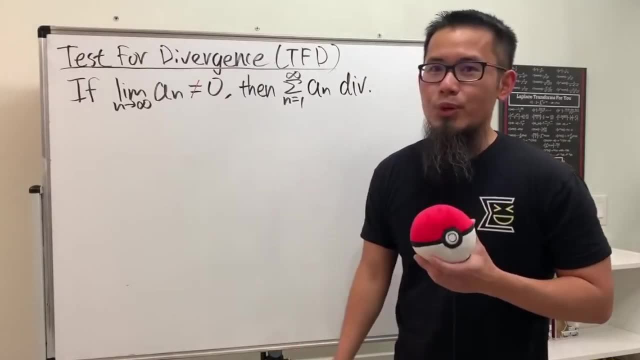 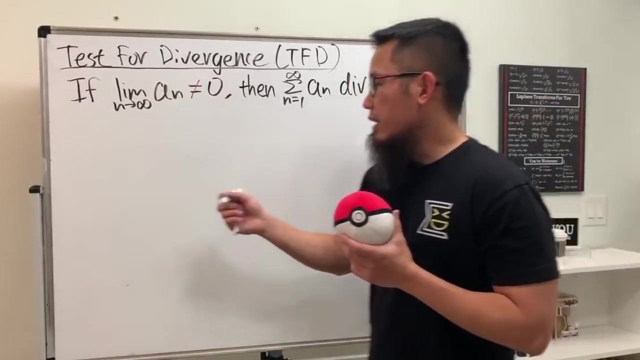 here a n, This series will diverge right. So this right here is really useful and you should always check that, and you will also have to be good with taking the limit of any kind of expressions that you have done so far right, So keep this in mind. Next, we'll also need to know the geometry. 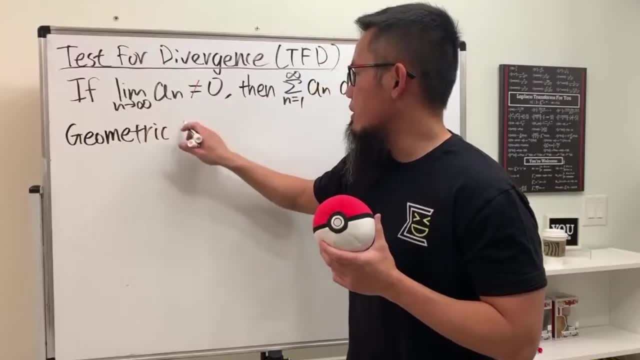 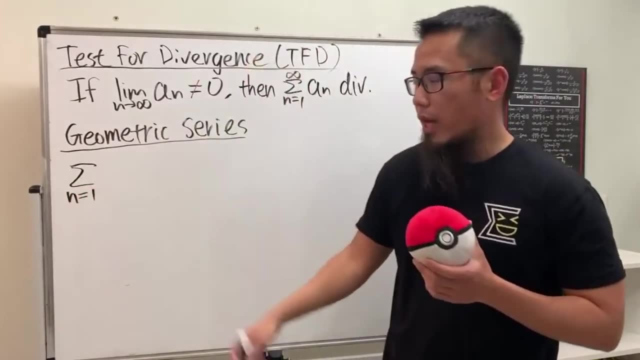 series. So let me just write this down here for you guys: Geometric series, And this right here has a special form. This is the series, and usually it's written when n is starting with 1, right, So it going to have a form. So it goes from 0 to infinity, right, So it goes from one to粽, and 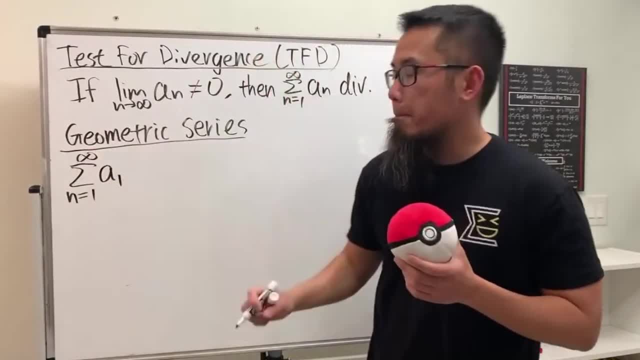 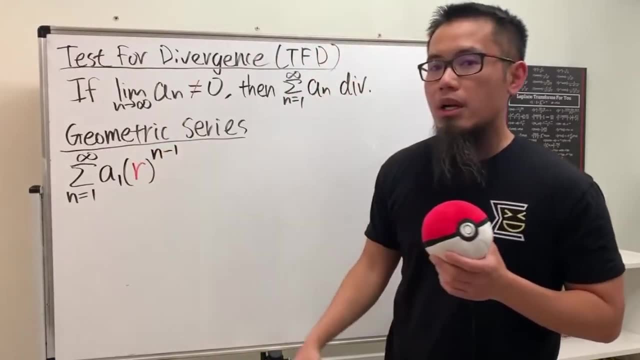 th and back. So now it's time for Geometry察, solemnga, and this is the initial term right. So it to infinity. and we have the first term, a1, and then we will have a common ratio, namely r, and then we are going to raise that to the n minus 1 power. again, this is the usual form for it, and once you 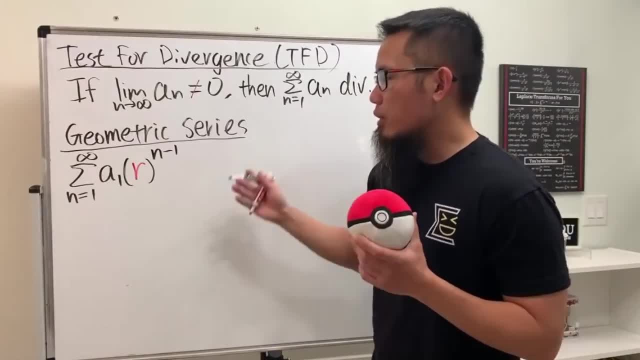 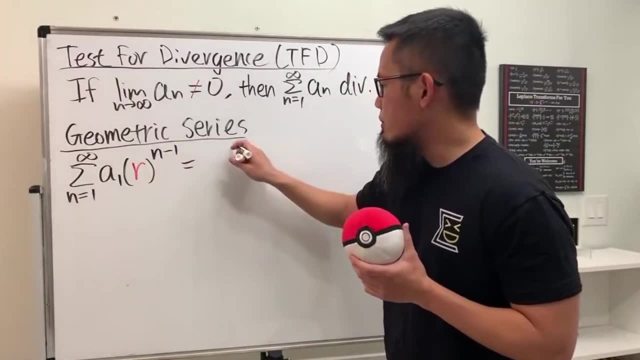 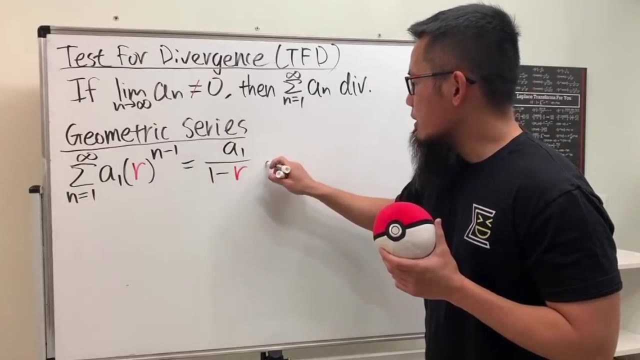 have this right here, let me tell you, you actually get to know if it converges or not. well, better yet, if this right here converges, you will know that this right here will converges to. it will converge to a1 over 1 minus r. all right. however, though, this only works if the absolute value of r 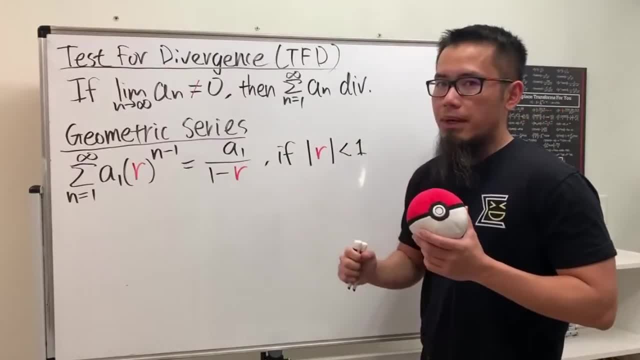 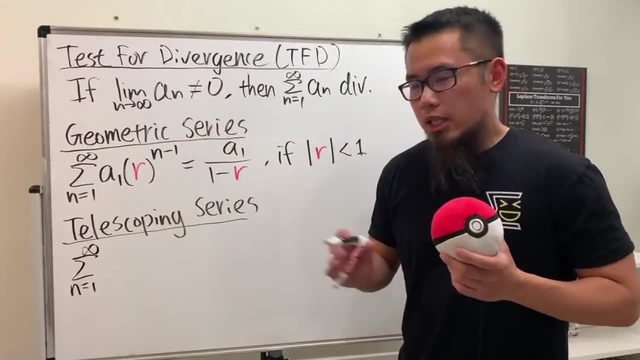 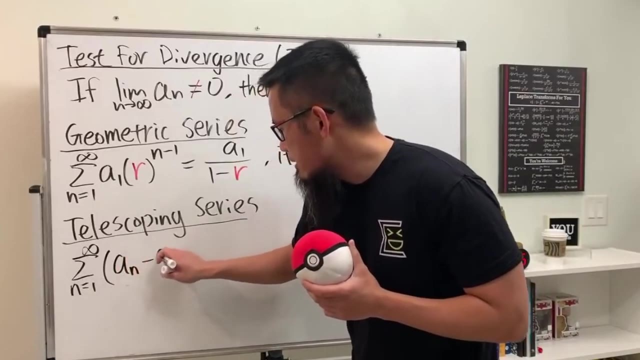 is less than 1.. so keep this in mind as well. but this right here it also has a special form. this is, when n is equal to 1, to infinity. keep this in mind, if you can somehow simplify the expression right here, and if you can make it into a n minus a, n plus k. 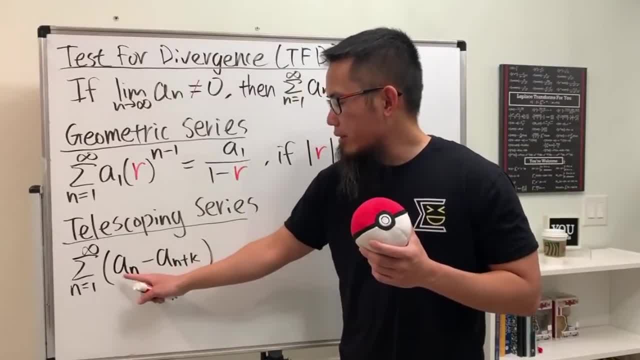 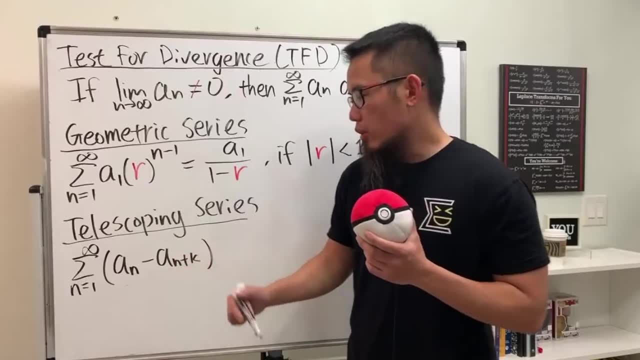 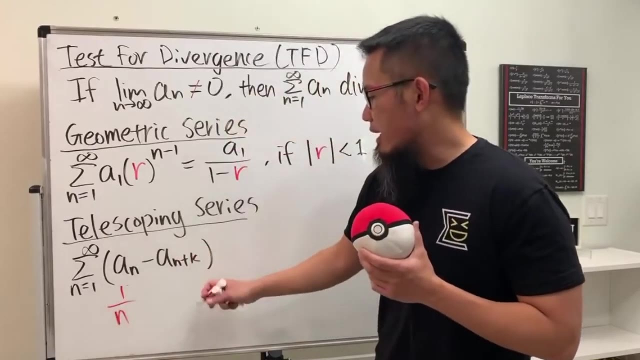 and what i mean by this is that, well, you have one term minus the other, and they are of the same kind, but they are just off by some terms. so usually you will see things like, for example, a n is equal to 1 over uh n, and then a n plus k. if k is equal to 3, then you are talking about 1 over m plus 3, and in. 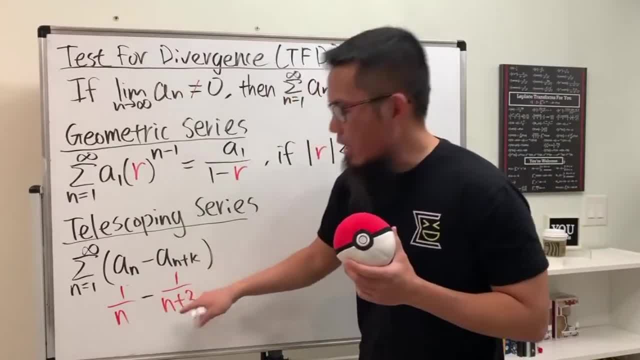 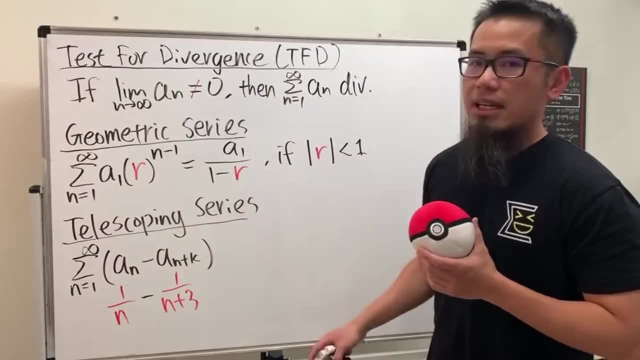 the middle is subtract, so, as you can see, they are the same kind, but they are just off by three terms, and sometimes expression can be slightly crazier. but this is the idea. now, once you have this, you're just going to write down a few terms and then just cancel things out, so perhaps i'll just write it. 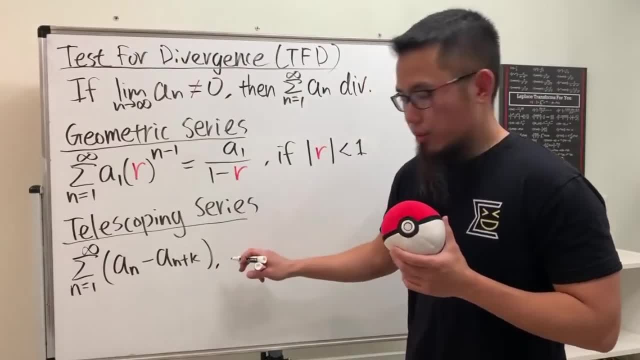 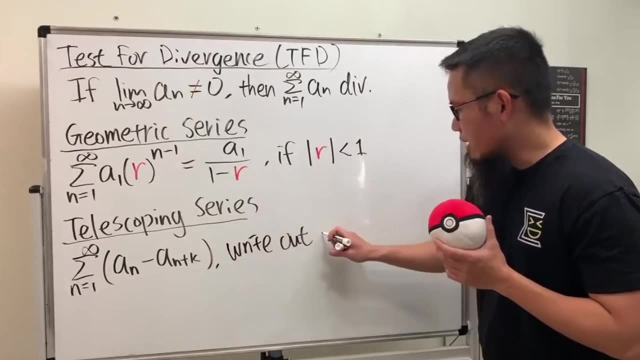 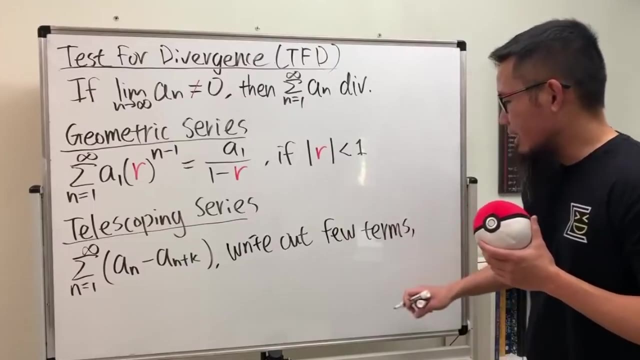 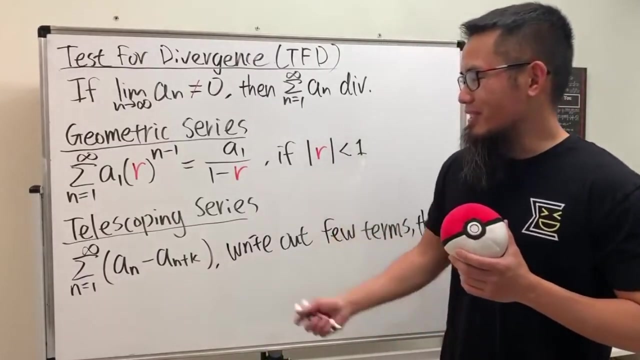 down right here for you guys, uh, write down a few terms. and so just write out a few terms and cancel it out. right now i have to say you've heard a few times- then cancel. yeah, then just work it out all right, because for this one right here, once you see, you will know what to. 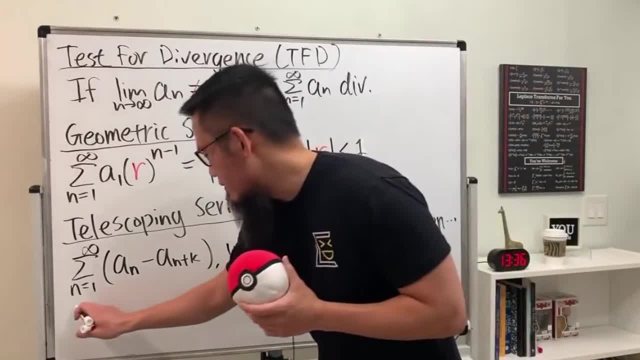 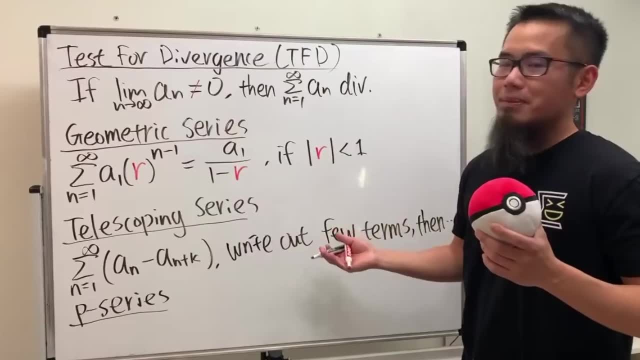 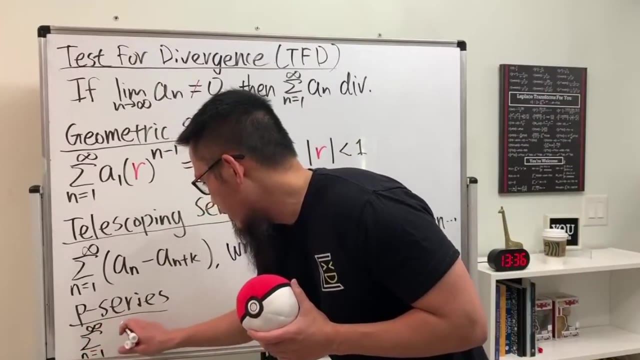 do right. and then last one, right here, this is everybody's favorite, namely the p series. why? because this right here is perhaps the easiest to see. well, i'll go, i will write this down here for you guys, right here. this is the series when n goes from 1 to infinity, 1 over n to the p's power. 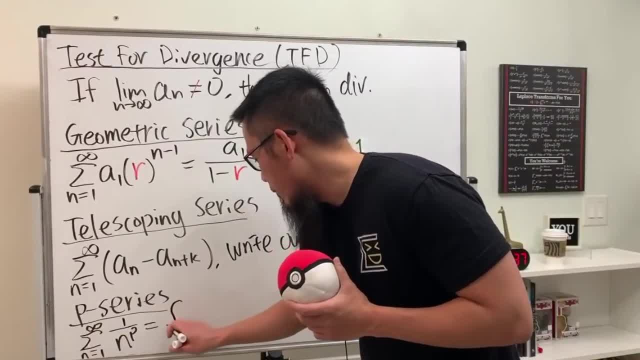 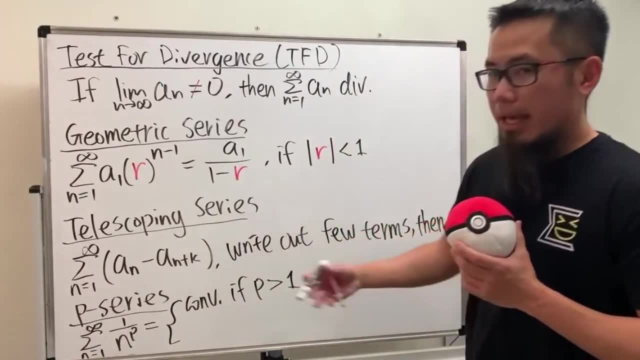 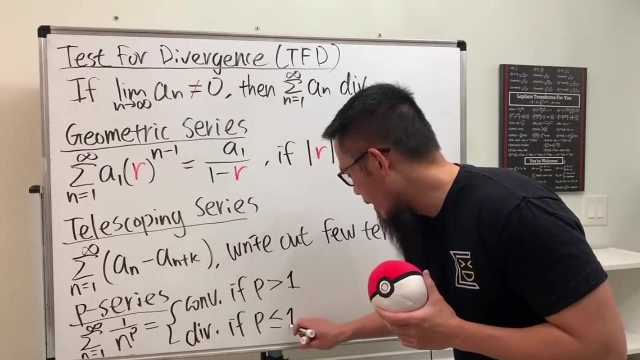 this right here. you actually know if it converges or not right away, so i'll write it down. this right here: converges if p is greater than 1, and that right there. diverges if p is less than or equal to 1. all right and for this. 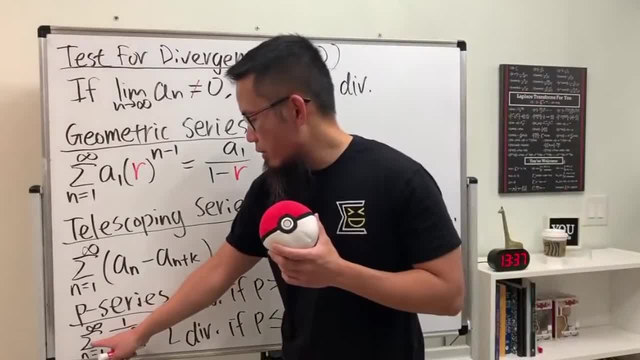 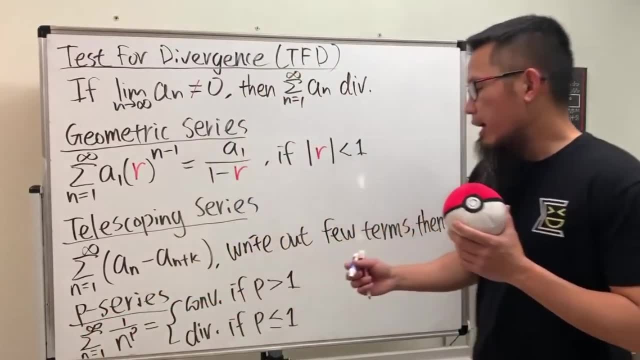 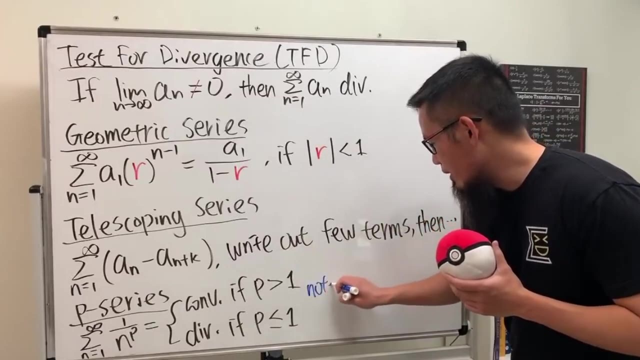 this is almost everybody's favorite. and again, sometimes you may see, okay, the series goes from 1 to infinity, but maybe you will see n goes from like 3 to infinity, but the statement holds and i want to just do some special mentions. all right, only for mention of special mentions, right? so just put down the note, right. 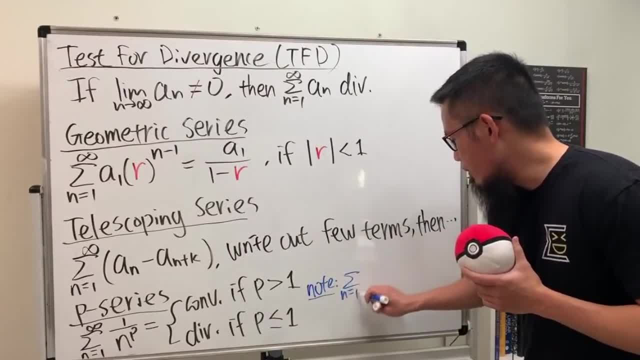 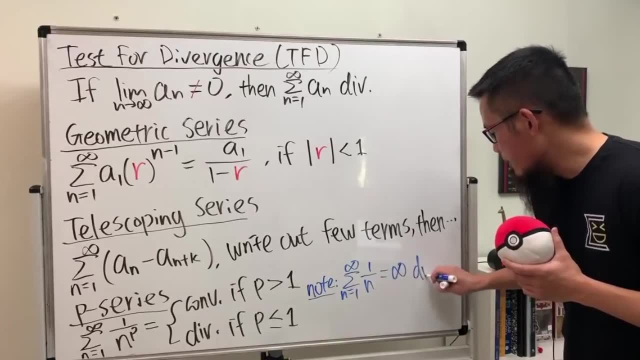 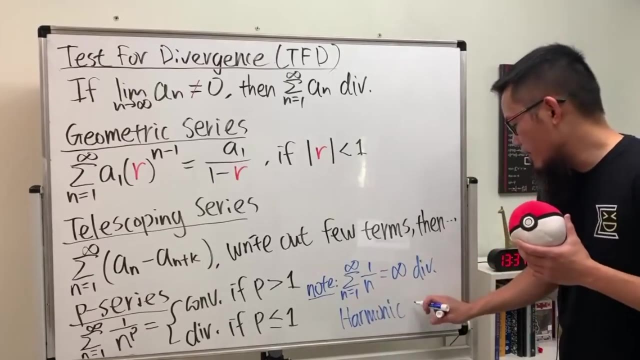 here, if you have the series as n goes from 1 to infinity, 1 over n to the first power, this right here actually diverges right and actually goes to infinity, and this right here is called the harmonic series, so it's just like a fancy name that you would like to use. 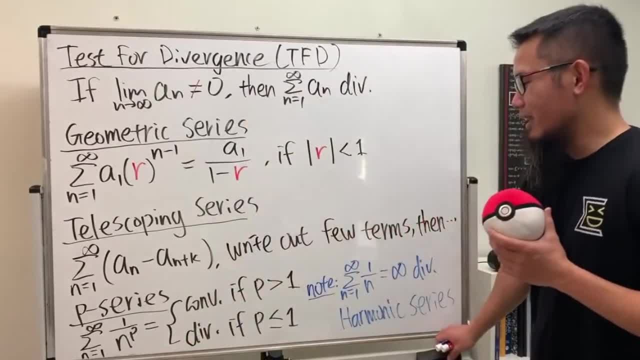 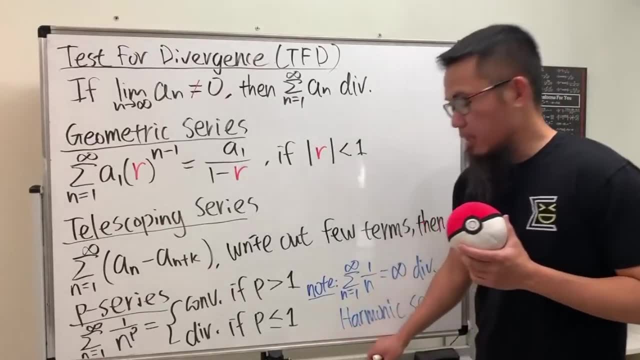 and you should actually, because the more you learn about this kind of things, you'll see more like a names for this consist. okay, so these are the things that you are going to keep in mind and we are going to get started with the first question. we are going to do two parts. the first 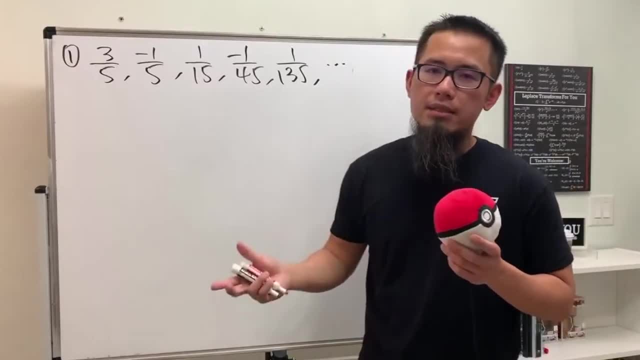 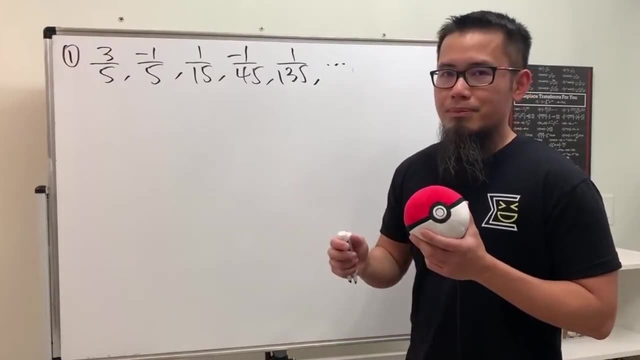 part is: does the sequence converge, why or why not? and if it does, what does it converge to? the second part is: does the series now, once you add them up, does it converge or not? so that's a different question and they are related right, and this is perhaps the 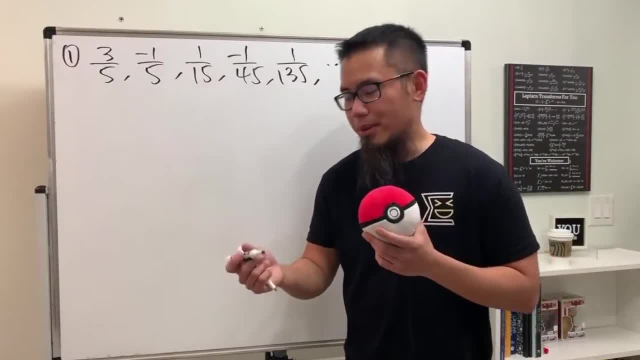 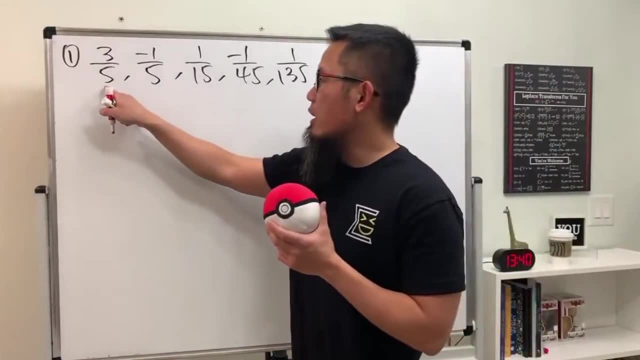 uh, uh. most important thing, if you are starting to learn about series and sequence, all right, usually you try to figure out from lab. so you are going to ask yourself: okay, how can we go from the first turn to the next term, and then from the next turn to the next turn, so on and so on. 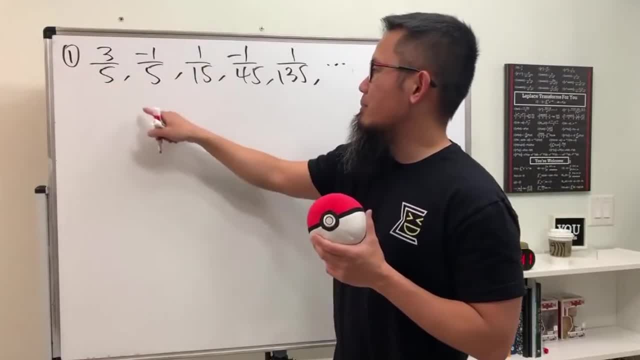 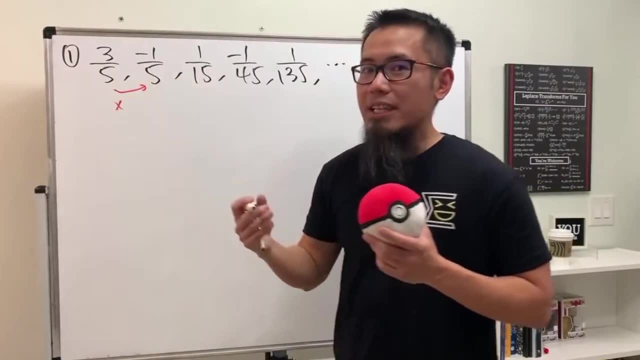 and it might not be too easy to see, because the five- but well, actually i don't know- it's actually just multiplied by negative one. sir, yes, it's divided by three, but when you are doing geometry series, whether or not closed in the third, it will fragment like half or a half, they don't. 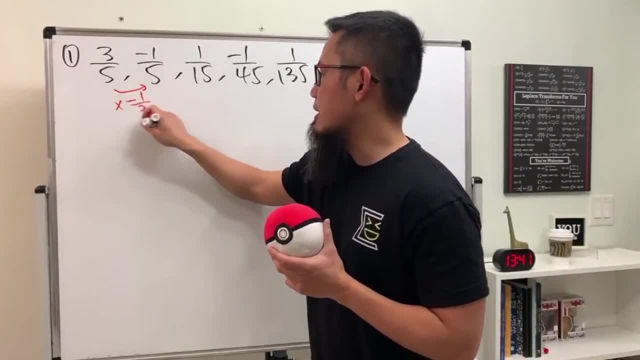 look exactly the same as here, but honor, of course, one that you just looked like your working efforts always look at this as multiplying by a fraction, So this is the same as multiplying by negative 1 third. All right, So it should be pretty clear. 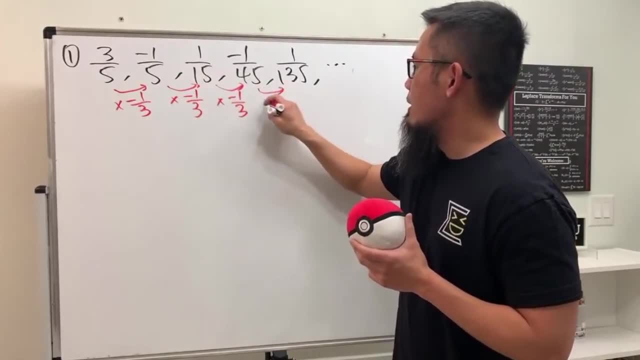 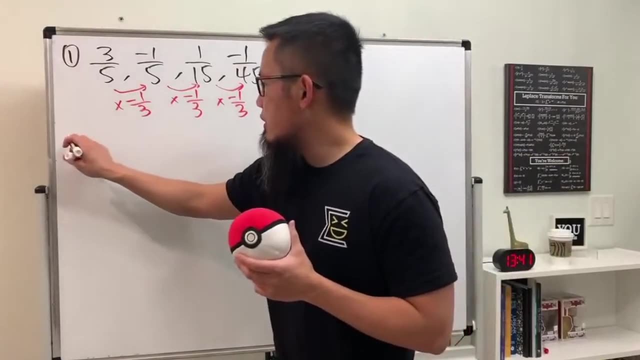 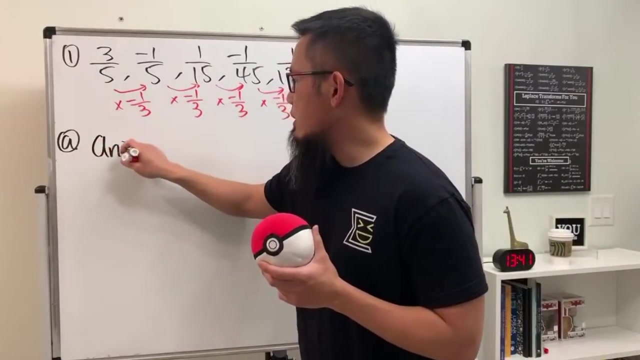 Yeah, Right. So this right here is actually a geometric sequence. So let me just give you guys the first part Again. the first part is to talk about if a n converges or not. First notice that a n is just equal to. 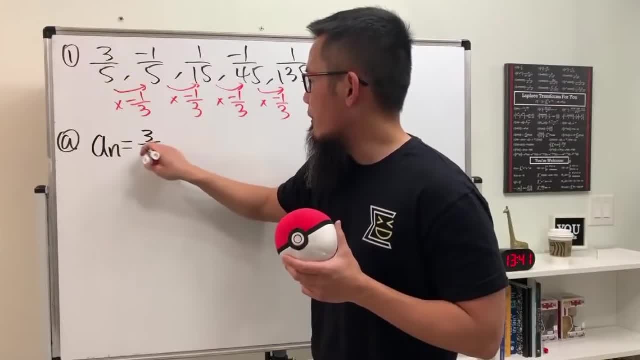 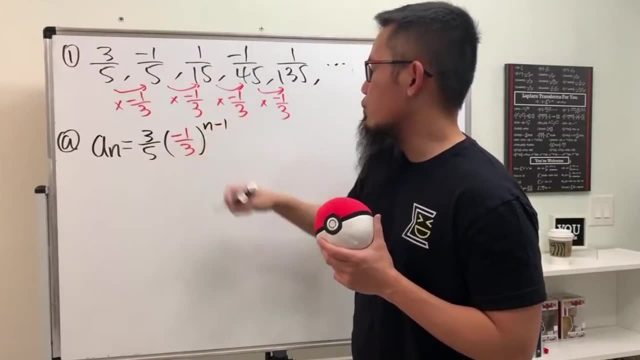 let's write down the first term, which is this: three over five, and we multiply by the common ratio, which is negative, 1, third, and then raise to the n minus one power, like that, And usually you can just leave it like this: 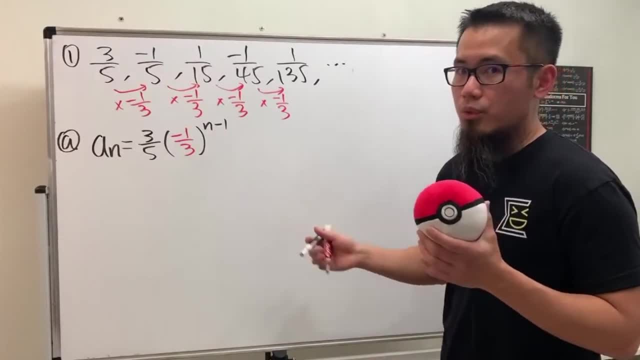 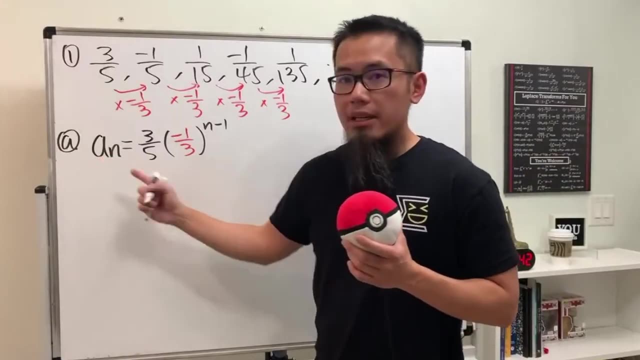 You don't really have to simplify, but that's just me. Depends on your teacher, Or maybe if you're taking a multiple choice question, maybe you have to simplify. do the algebra for that. But anyway, does a n converge or not? 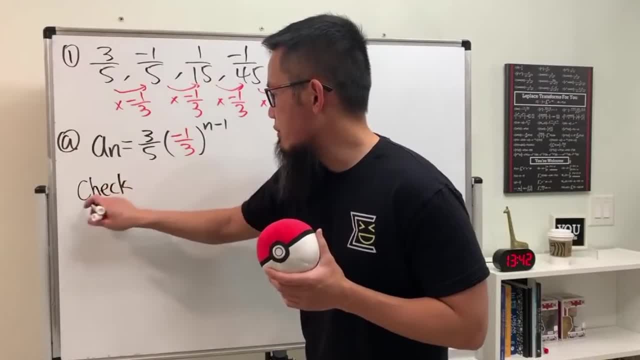 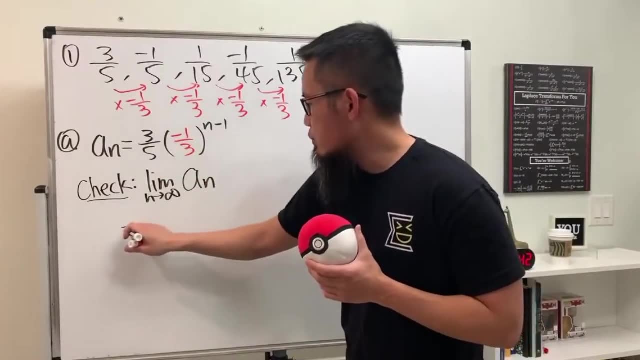 For this we always have to check right. We always have to check The limit, as n goes to infinity, of a n And because we have the a? n formula right here already, so we just do a limit as n goes to infinity. 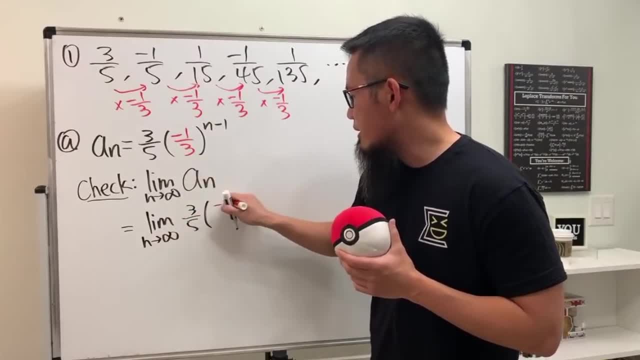 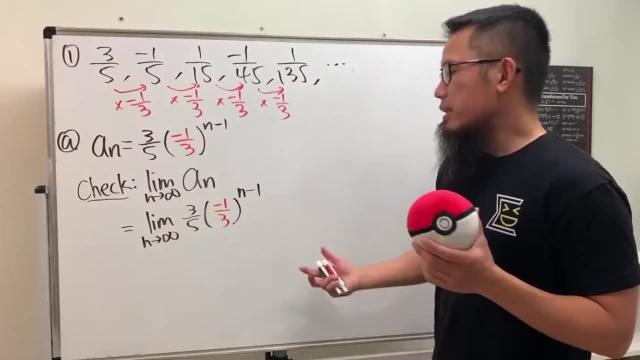 a, n is that which is three over five times negative, 1 third raised to the n minus one power. All right, And now it really depends on your teacher to see how much work that you have to show. But for my class, if you see, 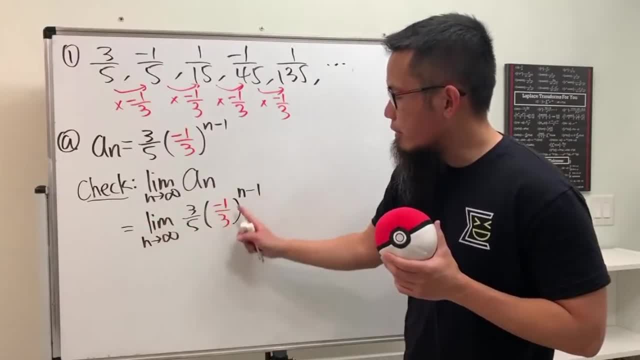 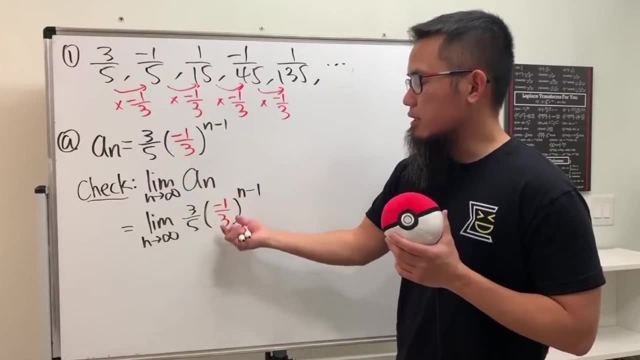 we have a limit as n goes to infinity. And this: now we have a limit as n goes to infinity. This number right is negative 1 third, because the absolute- and you can see that the absolute value of negative 1 third is less than one. 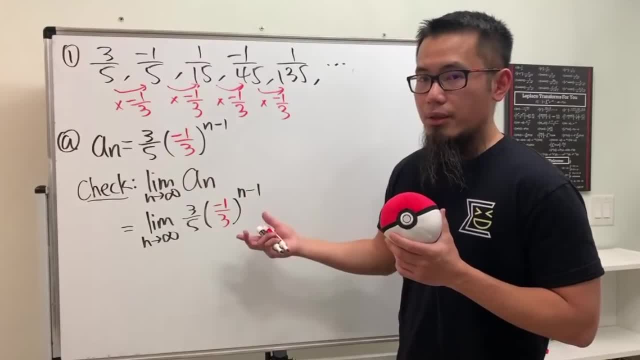 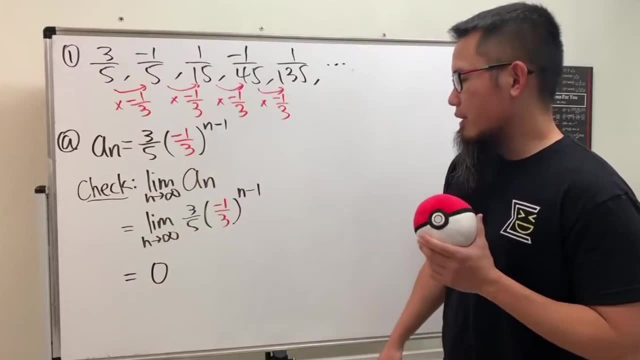 And then if you put this right, infinity right here, then you can say that this right here is just equal to zero Right. So that's pretty clear. I think that will be the jet. I will say Again, depends on how much of the word. 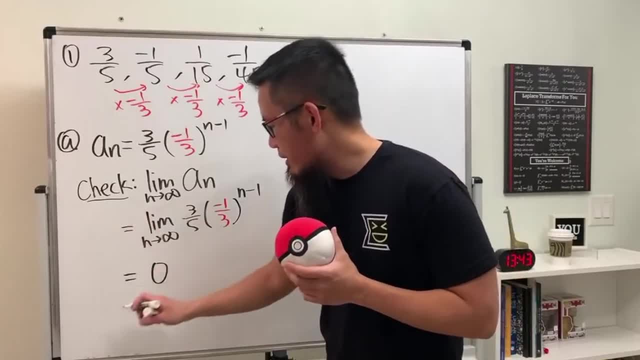 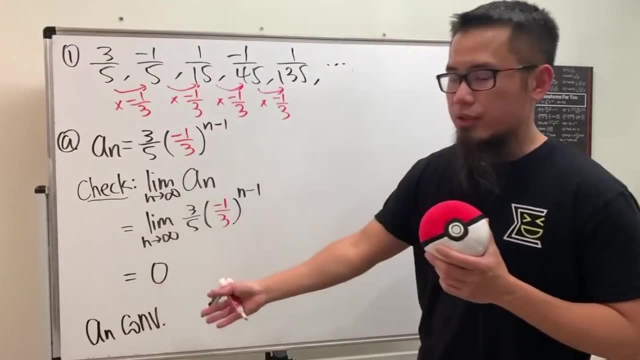 that your teacher wants you to show. All right, Here is zero. So therefore the answer is that, yes, a? n converges. Right a n converges, And right here we can actually say a? n converges to zero. 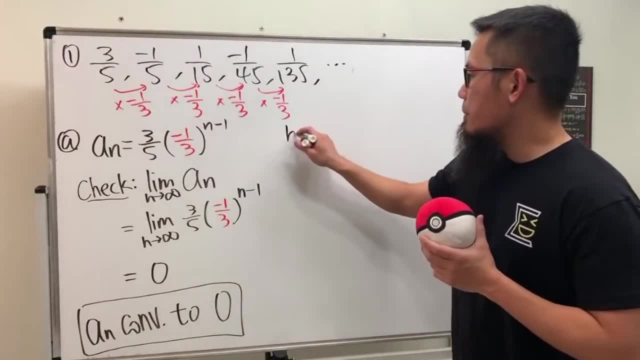 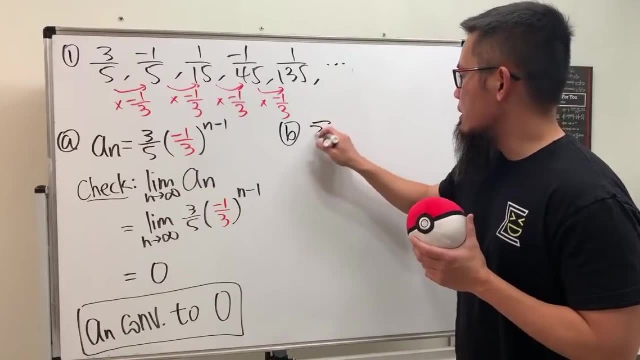 So this right here will be the answer for that. Part B. Part B says: does the series of a n converge or not? So we are going to check the series as n goes from one to infinity. n starts with one. right in this video of a n. 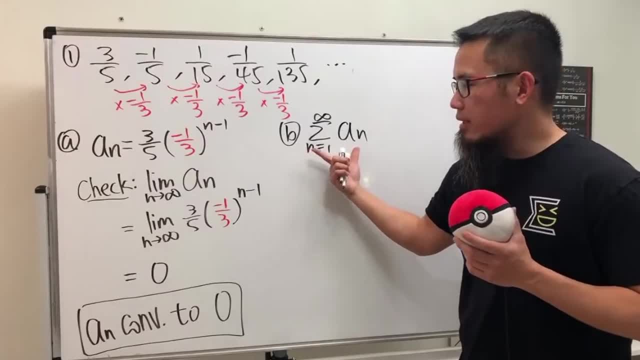 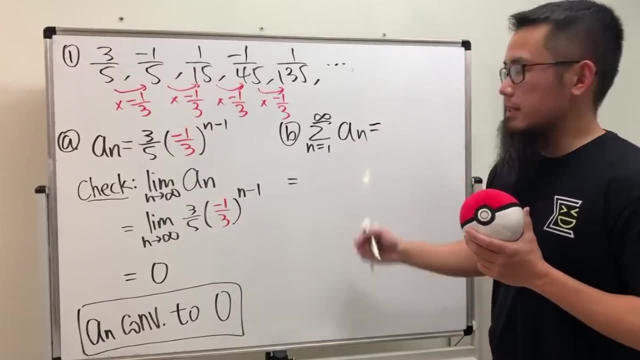 Does this converge or not? This is very different than that. So right here, check this out. This right here means what I will write it down for you guys. The series means we are going to look at all the terms right here and then we are going to add them up. 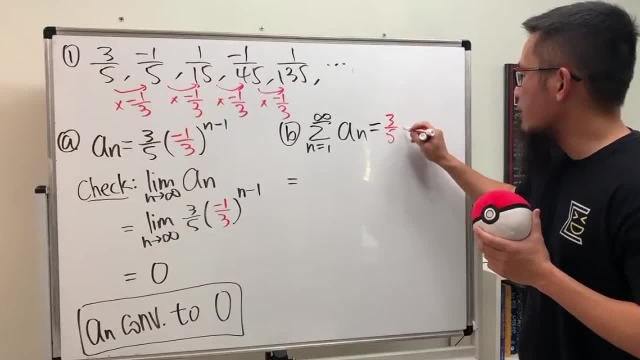 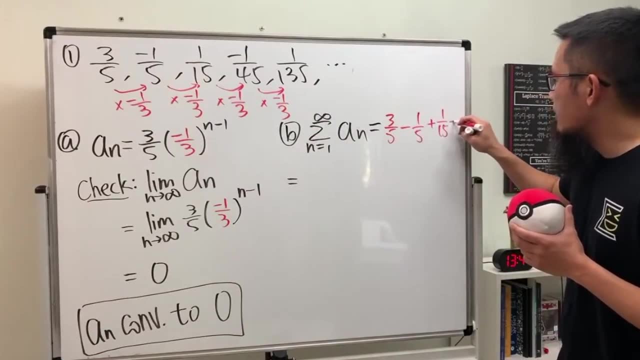 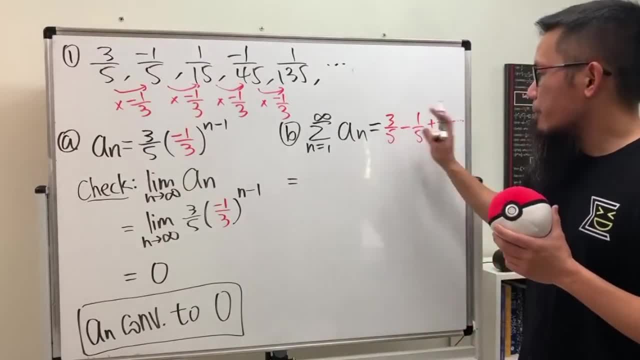 So that's what the question is asking. All right, So that's what the question is asking, All right. But anyway, though, this right here is a special case, because you know it's geometric, so we can just look at this and say: this is a series. 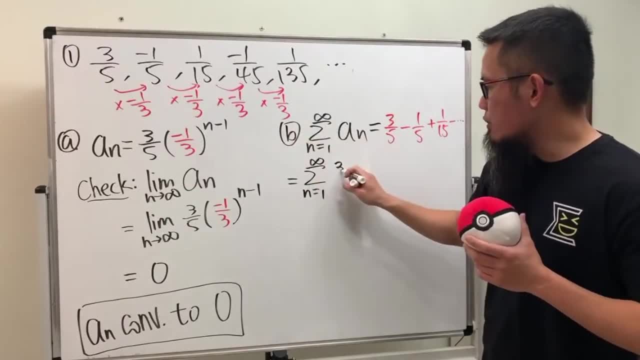 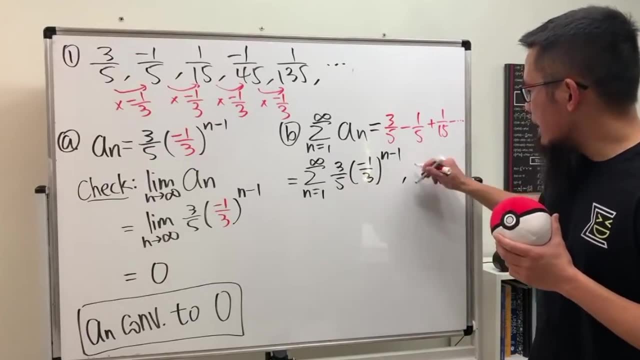 as n goes from one to infinity. a n is that which is three over five, negative one-third and minus one power. And again, because the absolute value of the common ratio, this right here, is less than one, This is one-third, which is less than one. 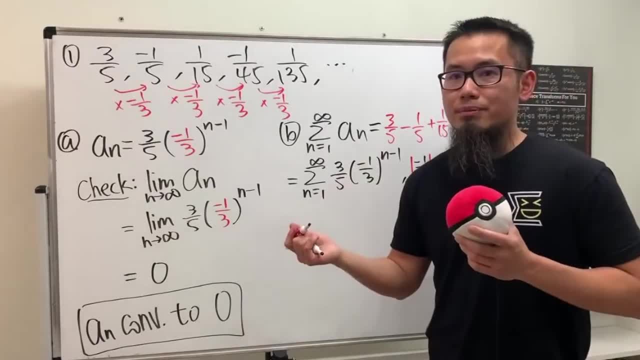 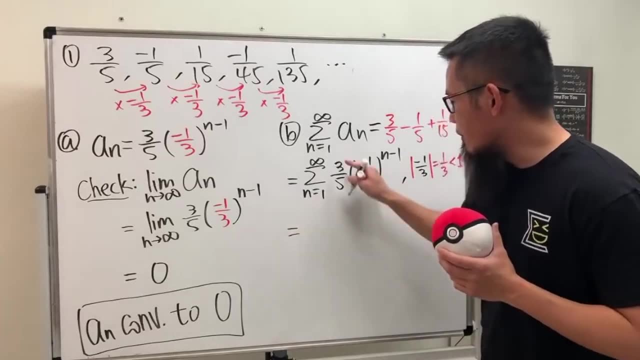 So we know. So this right here converges by the geometric series And, better yet, we can actually compute the value of this. And to do that we are just going to use the first term, which is three over five. 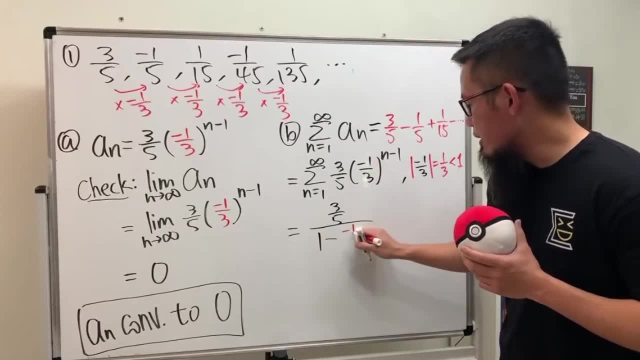 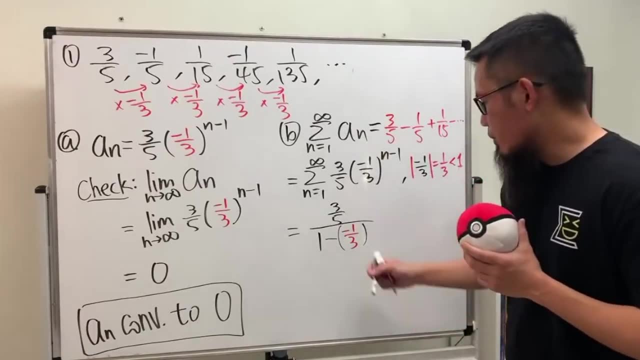 divided by one minus the common ratio, which is negative one-third. So that's very nice And again, this is legitimate, because this is true. And now just work this out. This is four over three on the bottom, and then 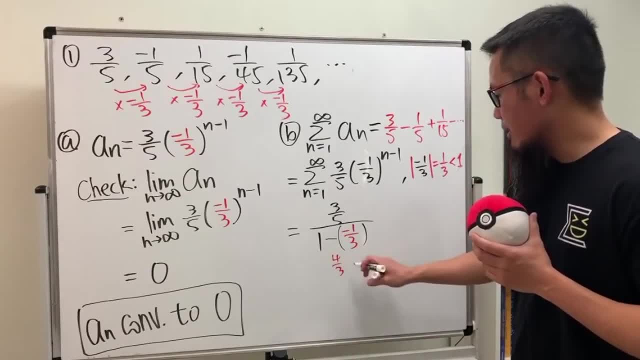 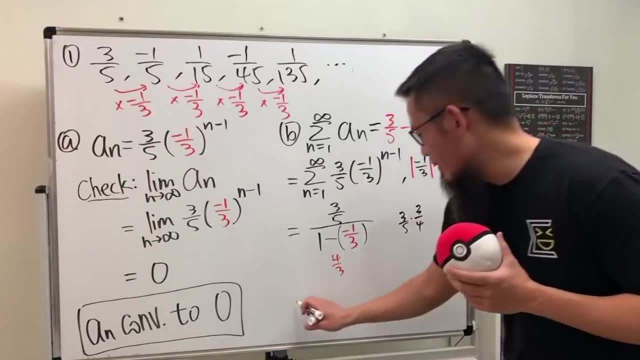 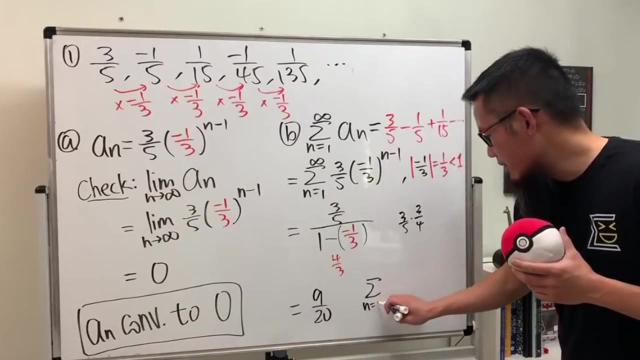 heh, yeah, And then let's multiply. So this is three over five times three over four, So altogether nine over 20, right, So right. here we'll just say this series as n goes from one to infinity of a n. 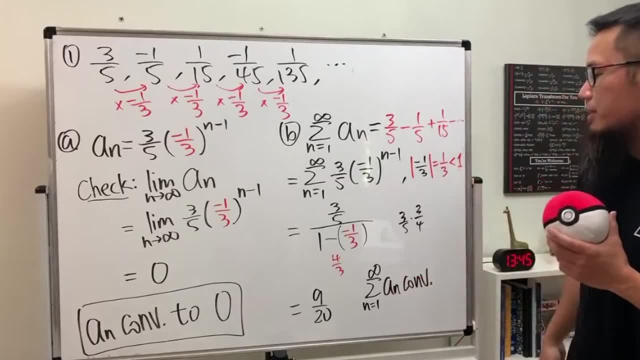 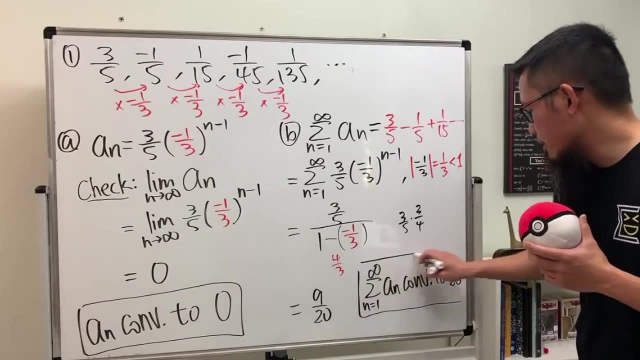 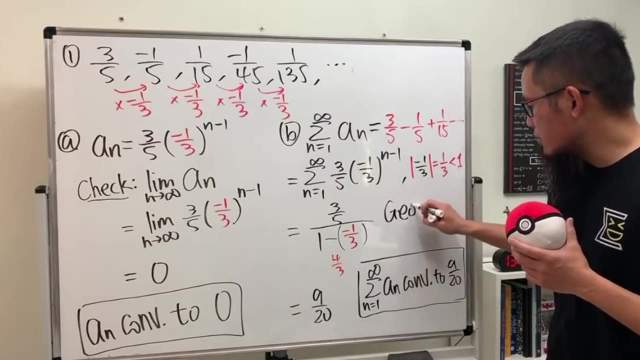 this right here converges by the geometric series and it converges to nine over 20, right, And maybe I should mention this right here as the geometric series somewhere, just to make it super clear, because the goal for this video is to 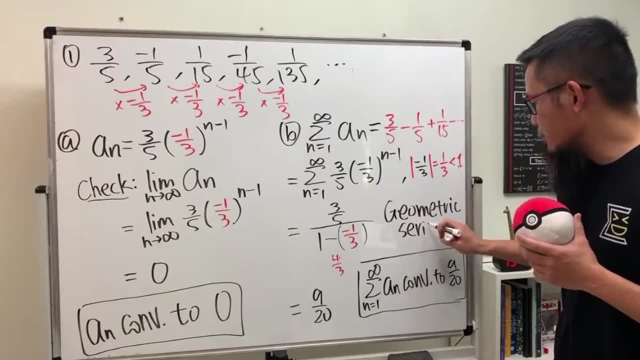 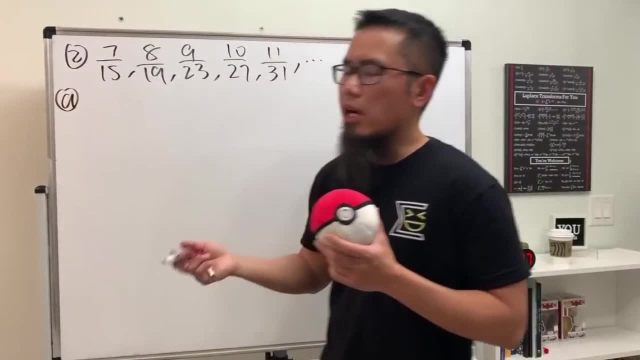 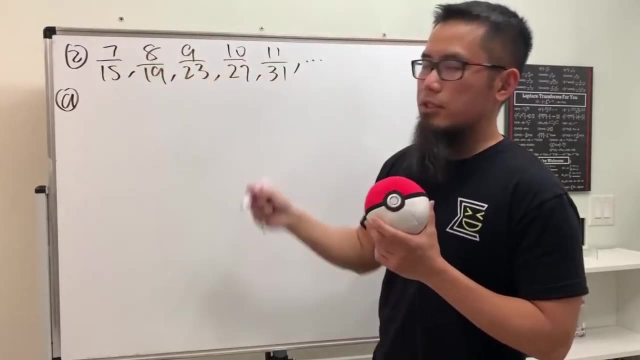 help the calculus to students right. First question: does a? n converge or not? So we're going to figure out formula for a n And for this I'm going to just write this down for you guys. Notice that the top is just always adding one. 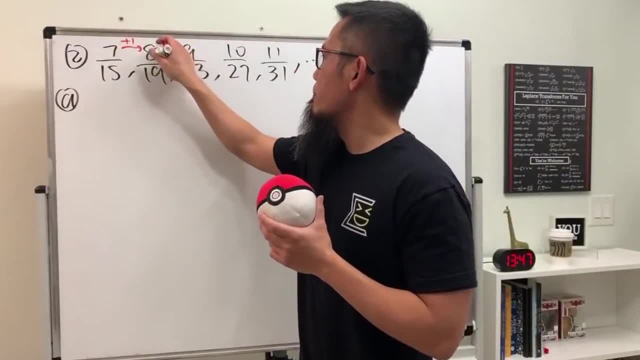 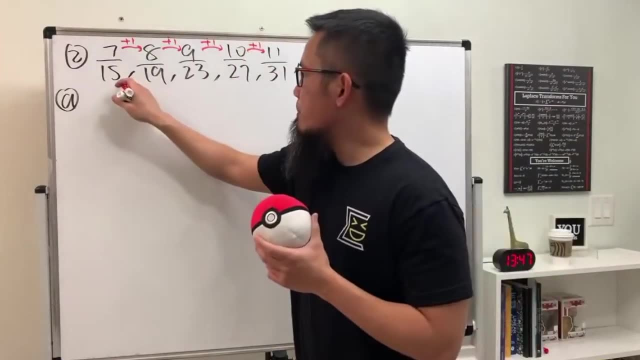 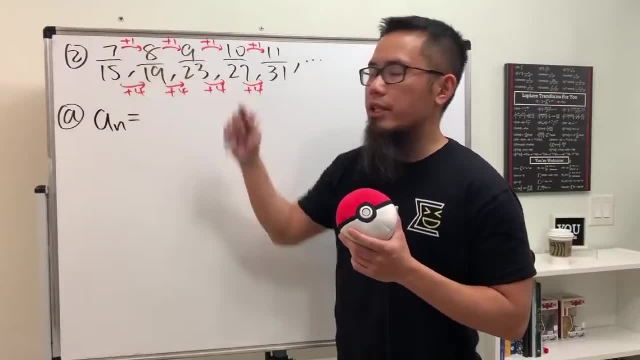 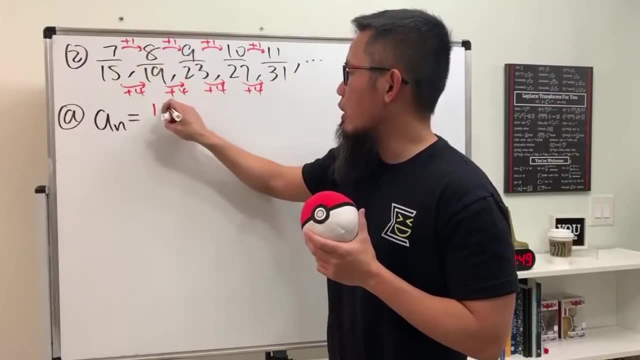 Notice, because we always add one on the top. so the top is actually what we call the arithmetic sequence. And this is how you can do it. The one is the common difference, That will be the coefficient of the n, And then, remember n, start with one. 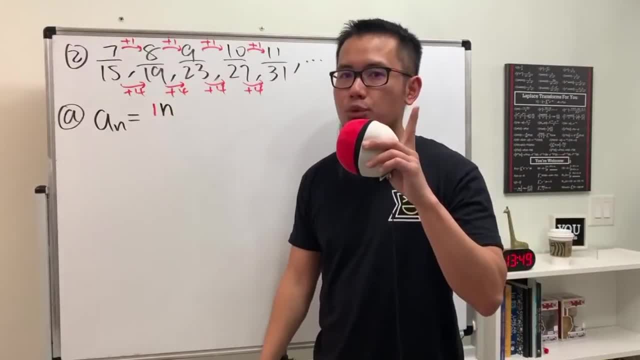 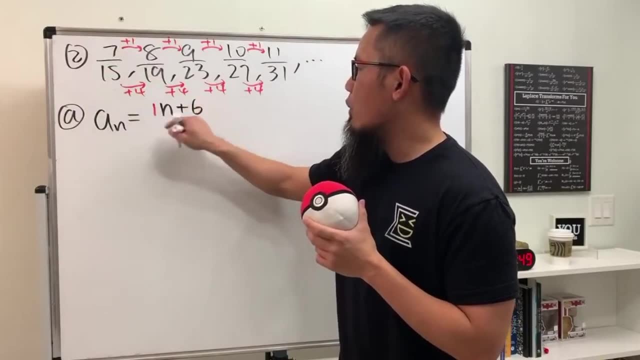 You put a one in here One times one is one And just ask yourself: one plus what will be seven? One plus six will be seven. So the top has the formula one n plus six. Well, don't worry, We'll do another practice down below. 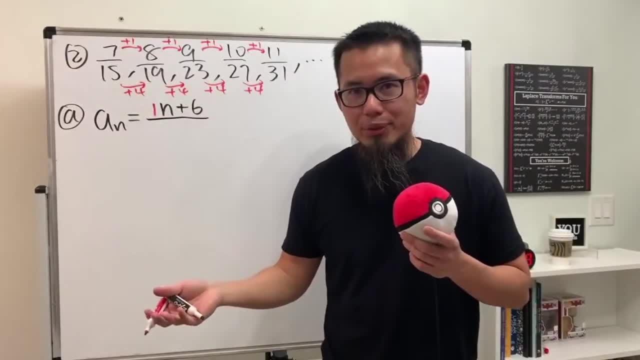 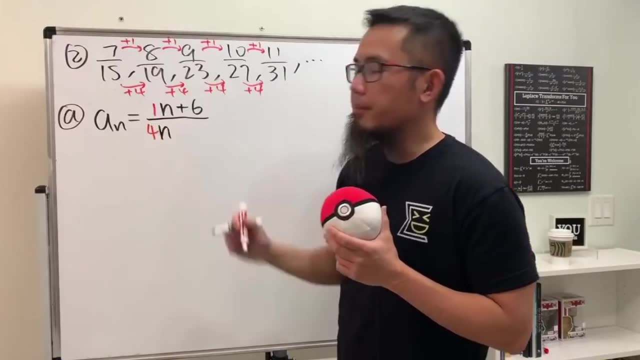 because the bottom is also arithmetic sequence, because you always add four, The four, the common difference is going to be the coefficient of n. So you put down four, n And again n. start with one. Put it here Four times, one is four. 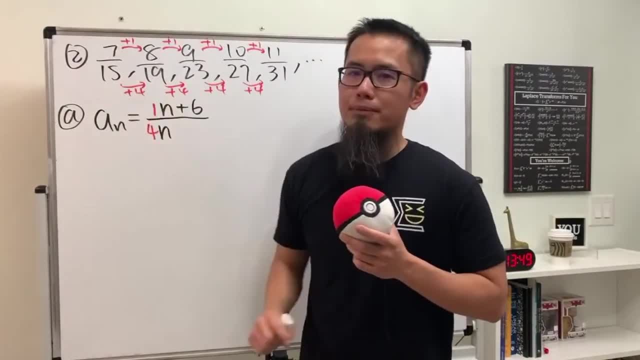 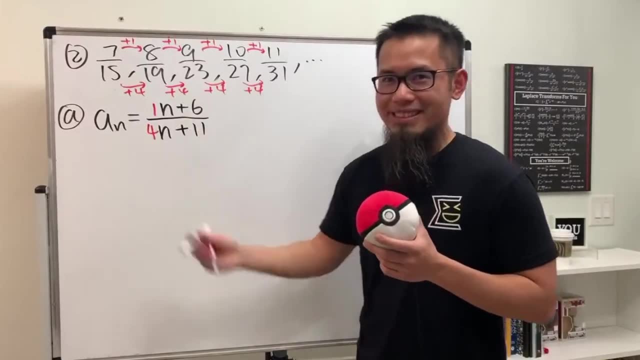 Four plus what will be four. Four plus what? Four plus what will be 15?? Four plus 11 will be 15.. So congrats. That's our formula for that right. And now does a n converge or not? 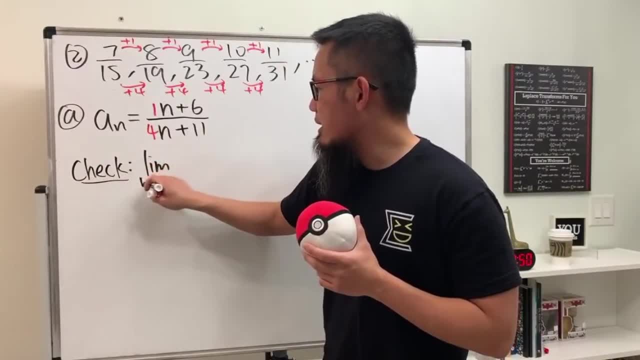 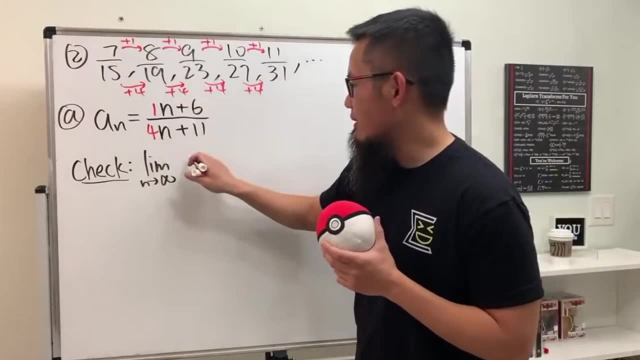 Well, for this we're just going to check the limit as n goes to. that looks like h, my bad. Thus the limit as n goes to infinity of a n right. And then let's see, this is the limit. 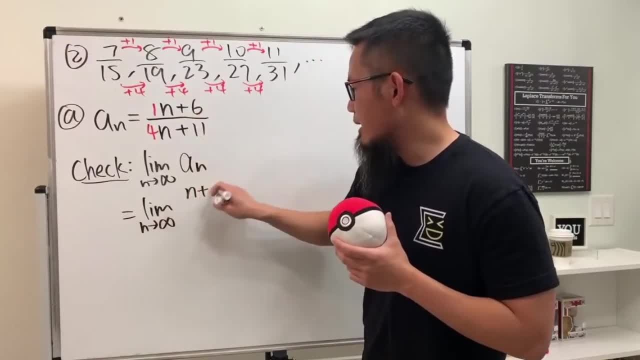 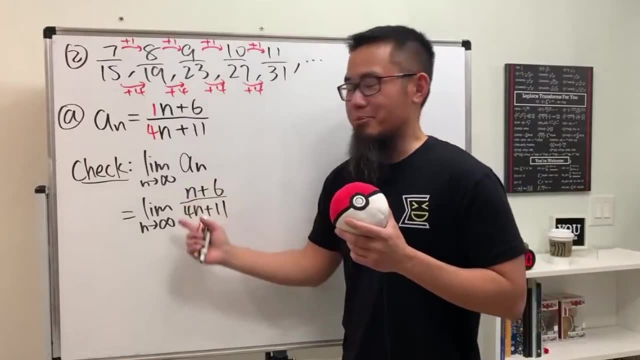 as n goes to infinity of n. All right, So this is n plus six over four, n plus 11.. Well, this is a Russian expression which is very nice, As n goes to infinity. this is like everybody's favorite limit question. 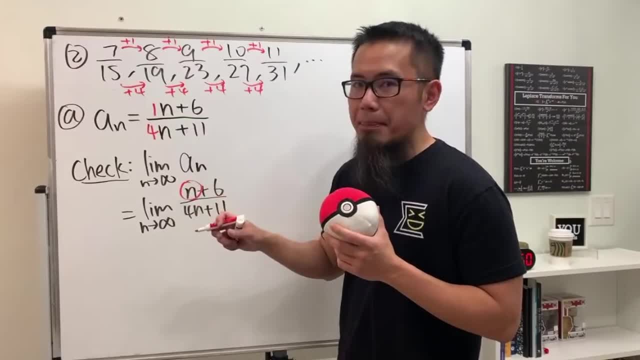 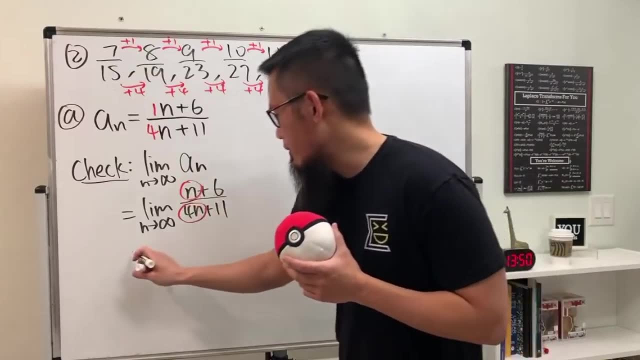 because all we have to do is pay attention to the highest power of n on the top, and then the highest power of n on the bottom, And then n reduced out, but we actually get one over four for the final answer Like that. 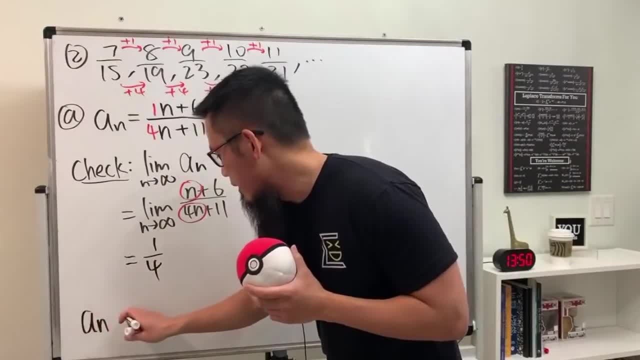 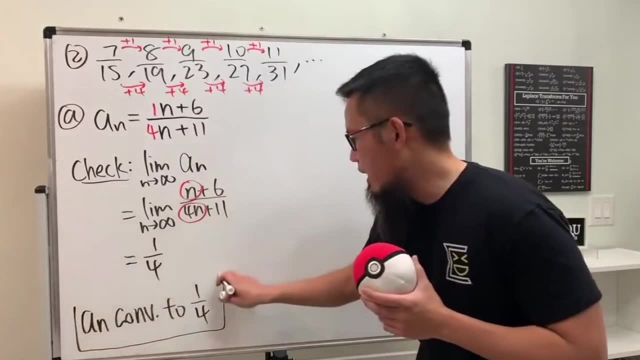 So, ladies and gentlemen, a? n does converge. I'll just write that down and we'll say: a? n converges to one over four. So this is very nice. Now for part two. you know it. We are going to see if the series as n goes from one. 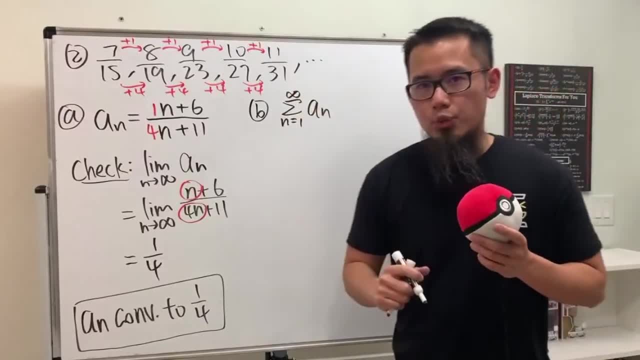 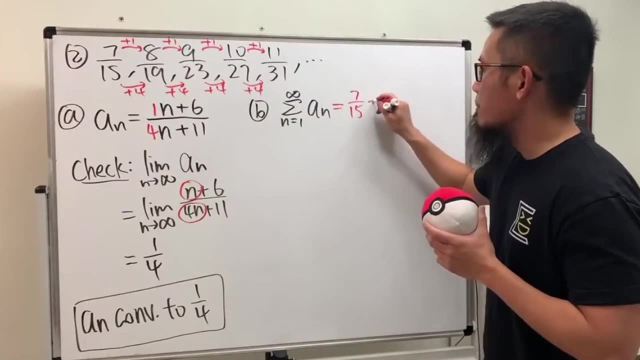 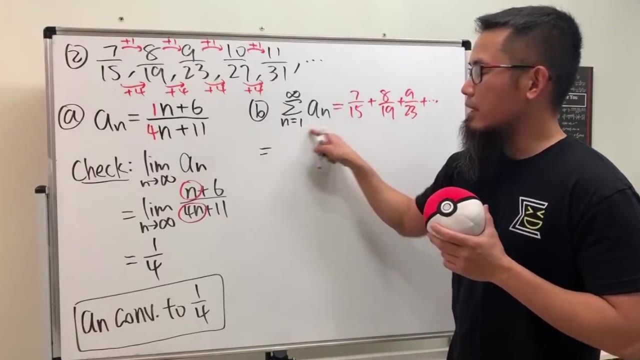 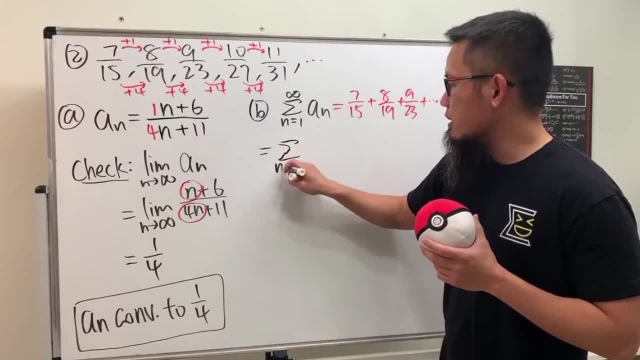 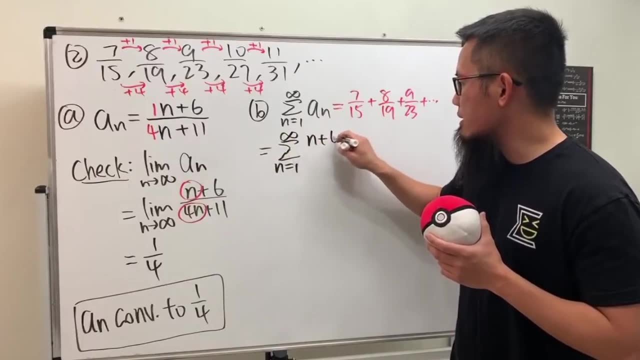 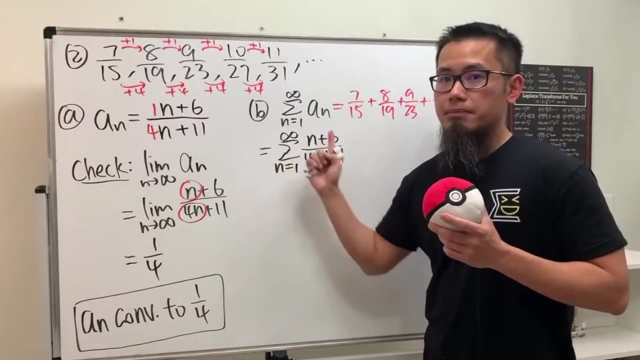 This right here, right, Sometimes, you will see, the question is just this: The series as n goes from one to infinity and they will just have the a n, which is n plus six over four, n plus 11.. You are going to see how to deal with this question a lot. 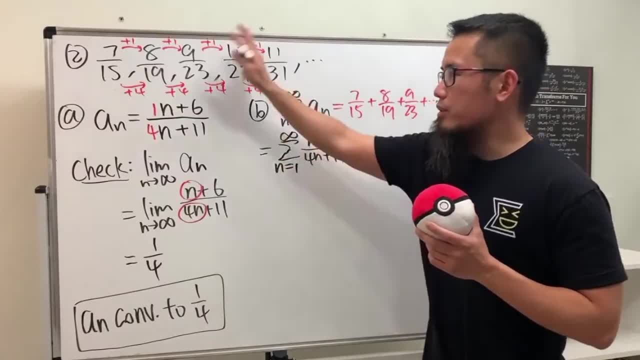 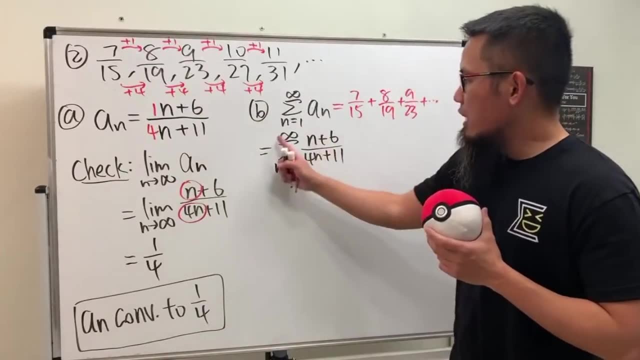 right in calculus two, especially the later section. You're not going to see other things, It's just like this, right here, you know, in front of you, You have to do it right away. If this happens, this is what you do. 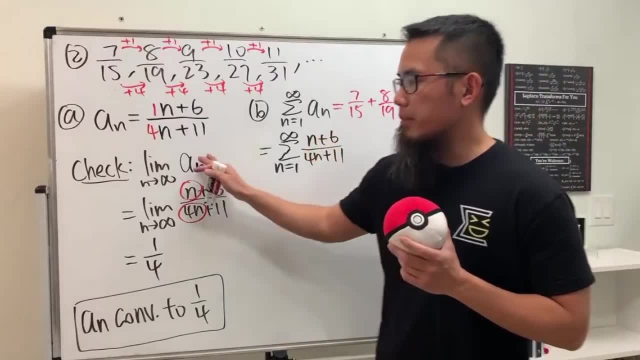 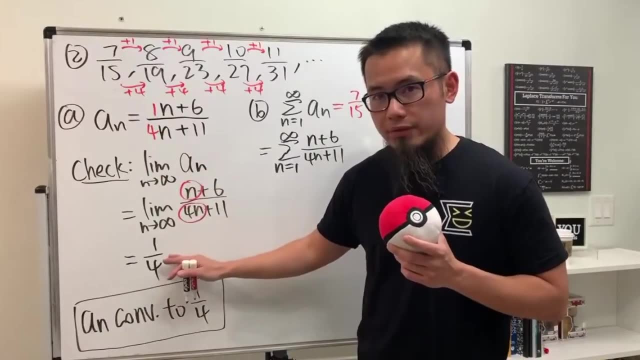 You always just look at this expression and do the limit on the side. If you do the limit, you will see that the limit is equal to one over four. The limit of a? n is equal to one over four. It's one over four. 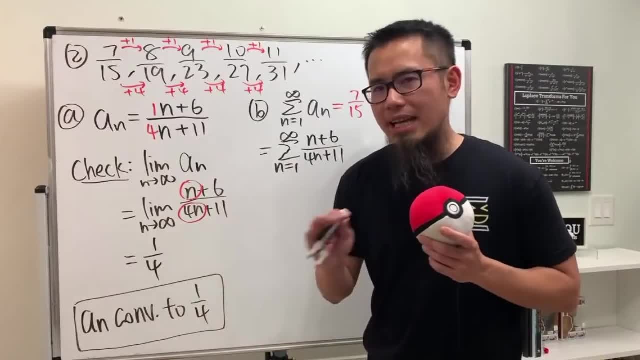 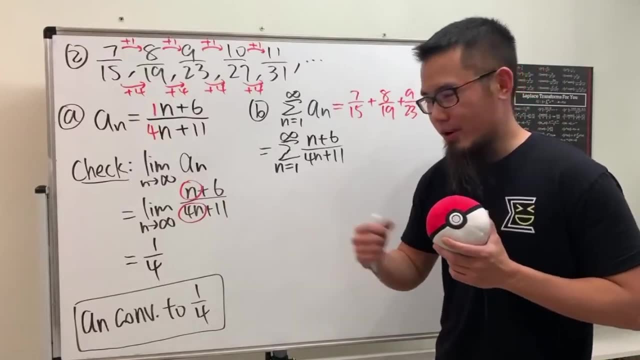 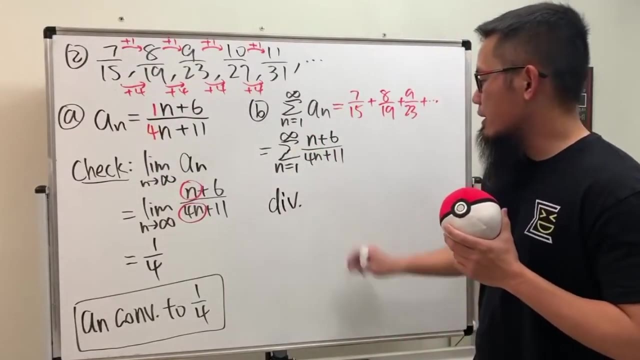 This is so nice because one over four is not equal to zero. So you can say that this right here diverges. And this is how you can write down your work Again: this right here- you can actually just say this, right here- diverges because if you take the limit, 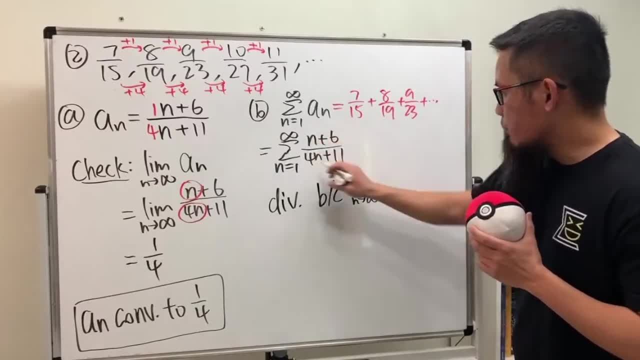 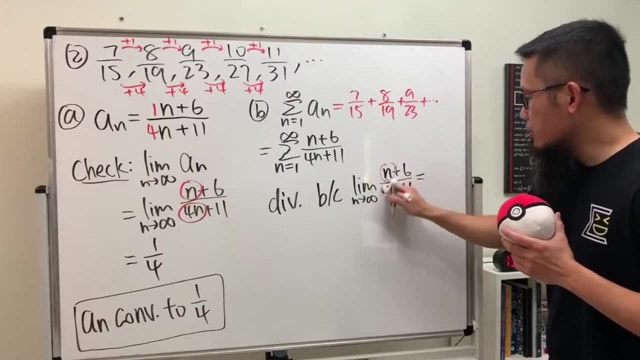 as n goes to infinity of this part, which is the a? n portion: n plus six over four, n plus one. this, right here again, as I told you, is one over four. But just you know, don't write down one over four. 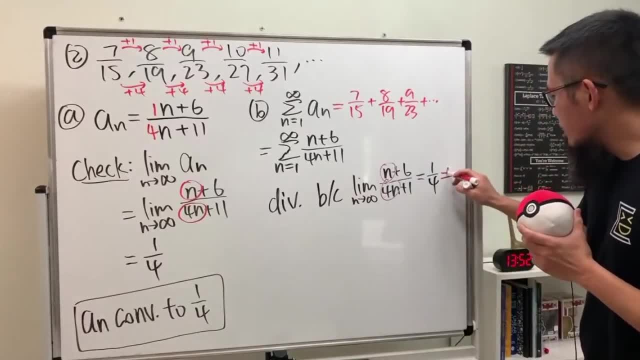 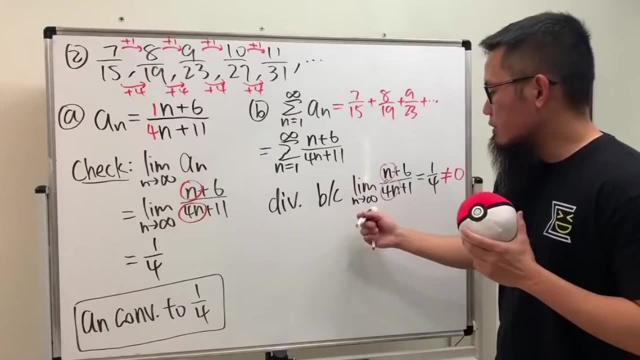 Don't just write down one over four. The most important thing is that you are going to write down: this is not equal to zero. This right here diverges because of this right here is not equal to zero. So right here I'll just say: the series n goes from one. 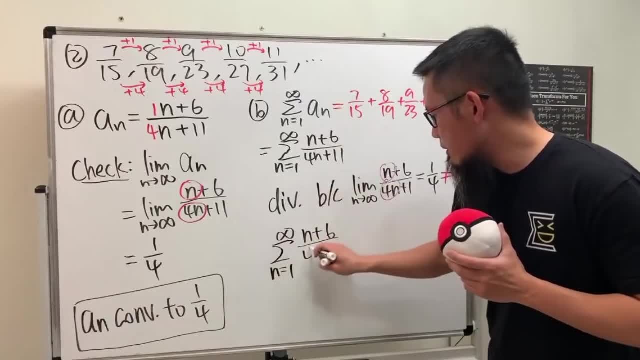 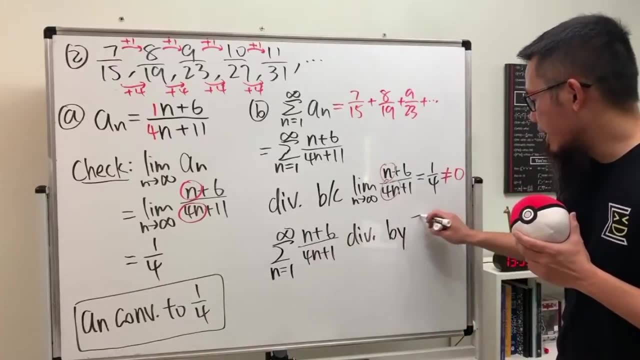 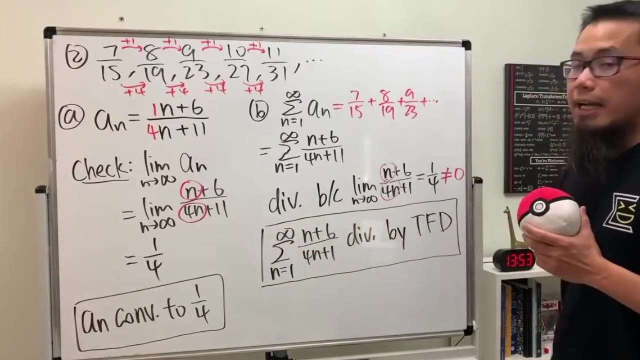 to infinity. this guy- let me just write it down right, This right here diverges and we can just say by test for divergence. So this right here is how you can write down your reasoning for that. And again, this is the little word I got to show. 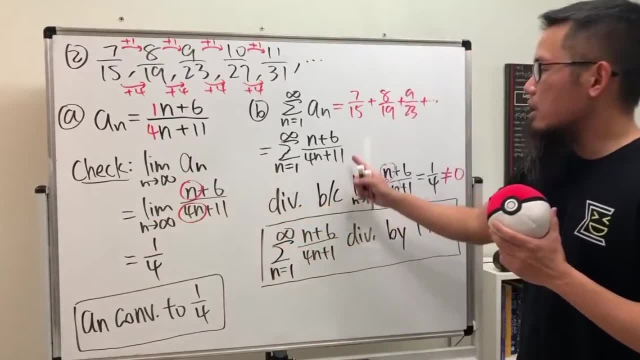 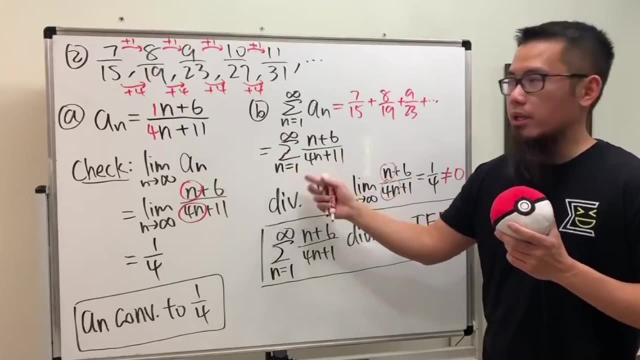 And again, yes, we know we did this already, but I'm just saying that if you have to do this question on your exam- which you will have to most likely- the question is just this: right, They wouldn't tell you to do the first part. 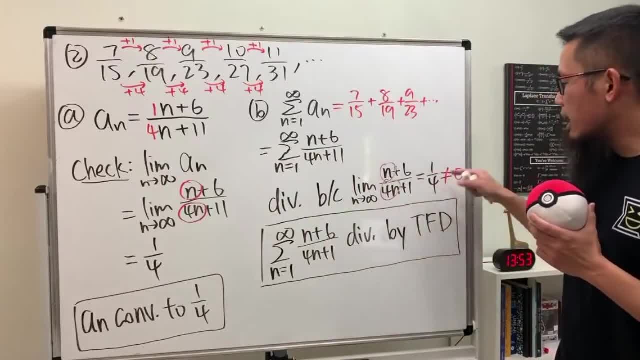 Then in that case, always do a limit on your own. If it's not equal to zero, congratulations, We can go from here to here and say this right here. diverges by test for divergence. Well, why is that when the limit's not equal to zero? 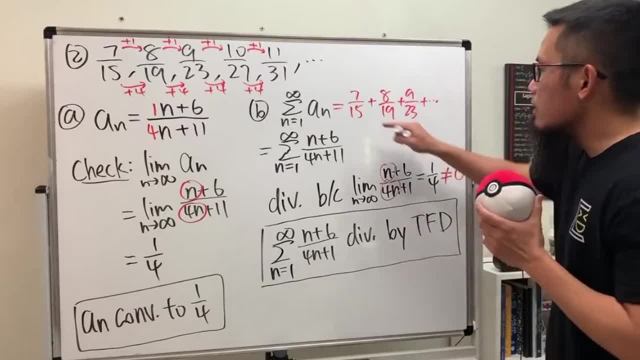 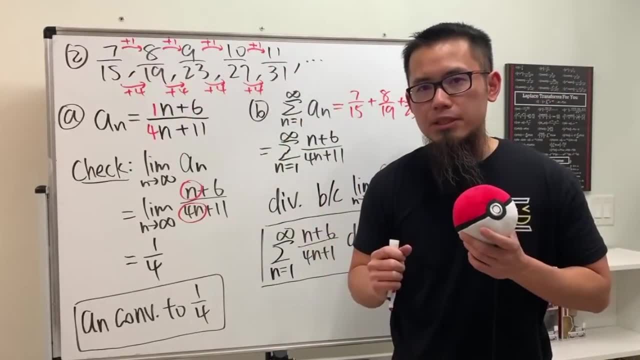 this right here diverges right. So that's why we have to do this right away. Here's the idea. Remember this right here means that we are looking at all these numbers and then we are going to add them up and we have infinitely many terms. 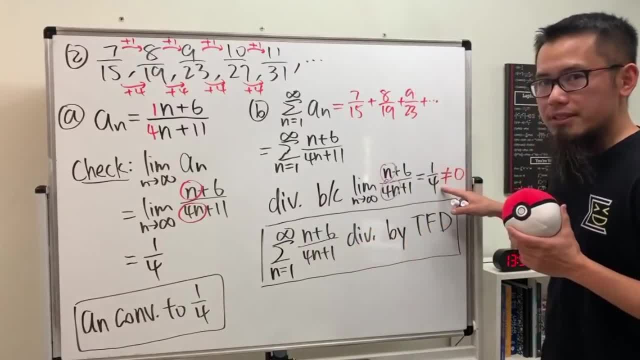 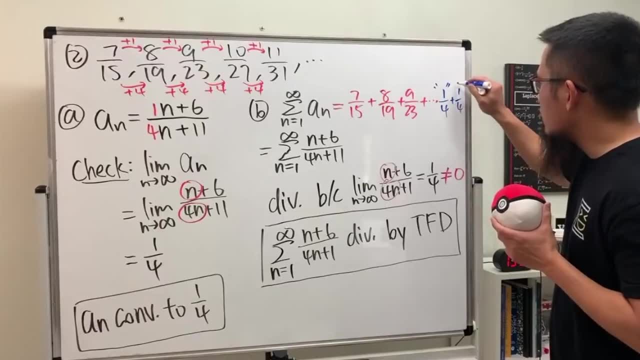 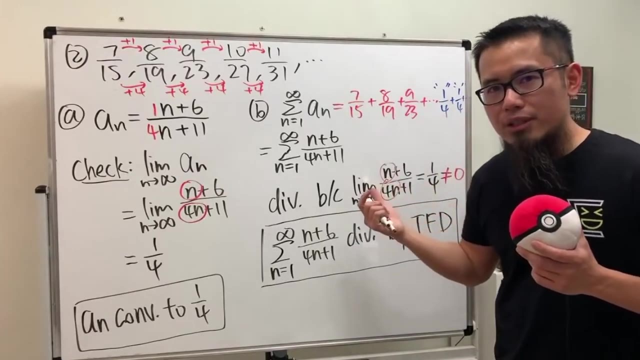 Well, the limit is being one over four. right here is telling you that eventually we are going to add one over four, one over four, and so on, and so on, infinitely many of them. And now imagine if you have to add up. 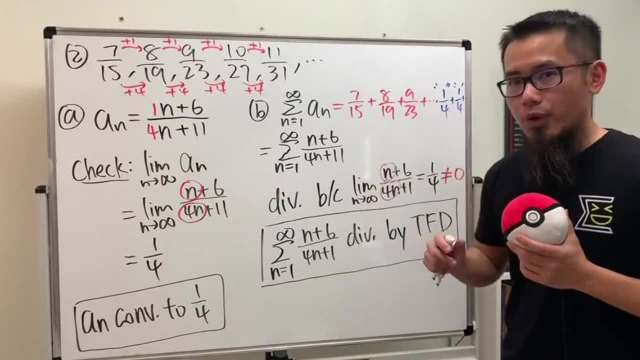 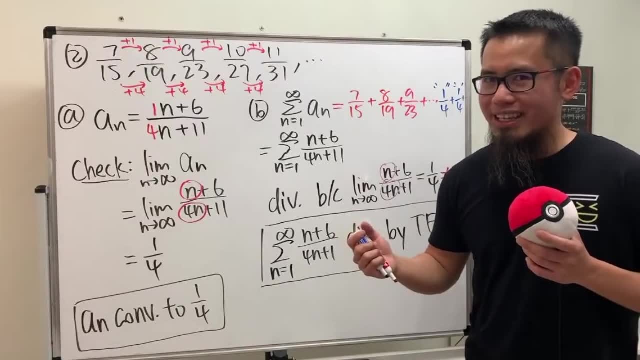 one over four. right Approximately being like this is about one over four. If you're adding up all this right here infinitely many times, what will happen? Well, it will get bigger and bigger, isn't it? Yes, So this right here will actually go to infinity. 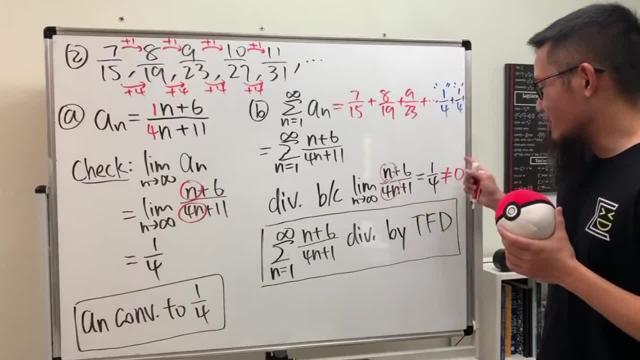 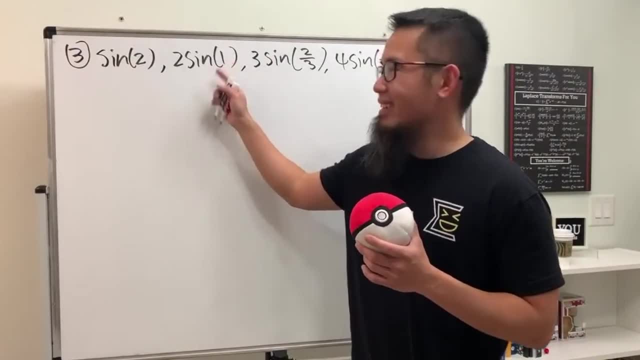 That's it, right. So when you don't see this being equal to zero, you can be really happy for that. So here's the deal. This right here is actually the same as two over four, Right? so no sorry. 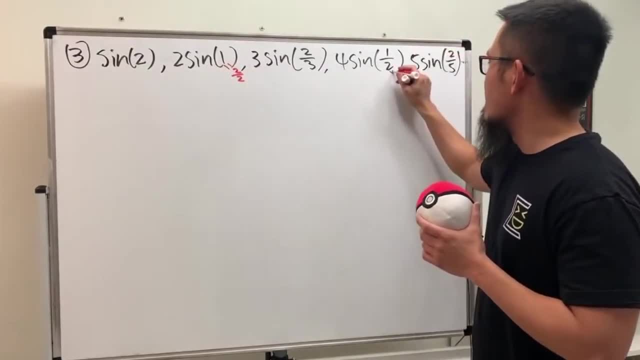 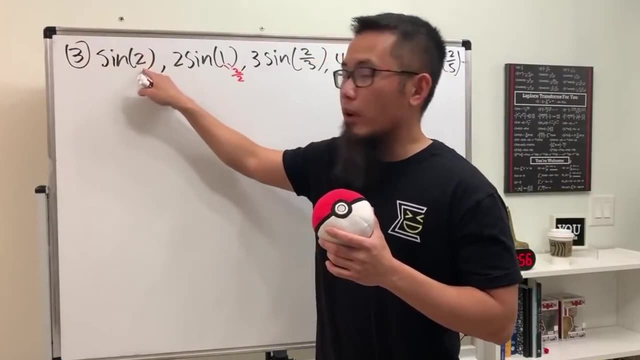 This right here is the same as two over two, And this right here is the same as two over four. And remember, n starts with one. so this is the same as one times sine of two over one and then two times sine of two over two. 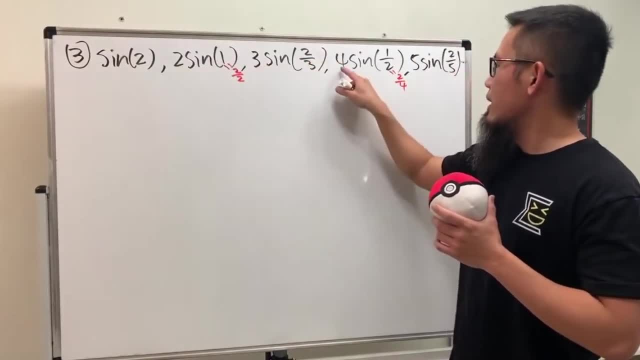 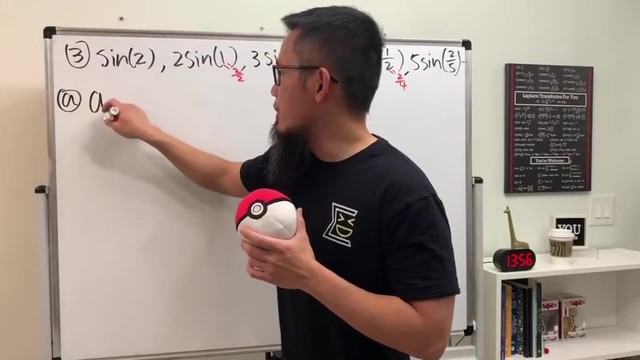 and then three times sine of two over three. the three match and the four match like that, And last, one same thing. So anyway, same thing. Part a, first, we know a n. The formula is just n times sine of two over two. 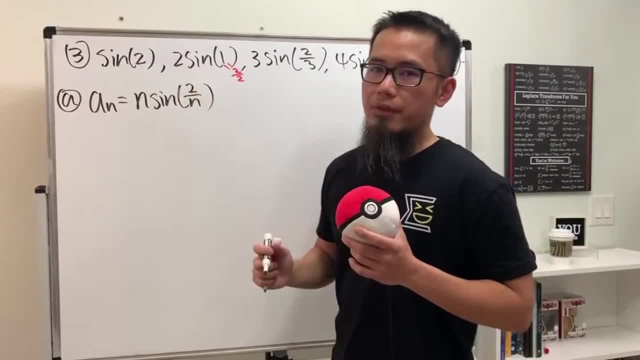 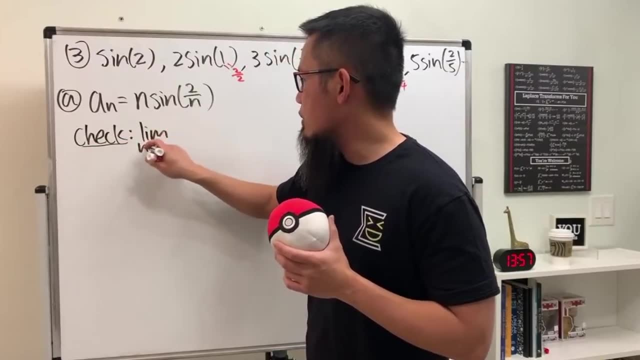 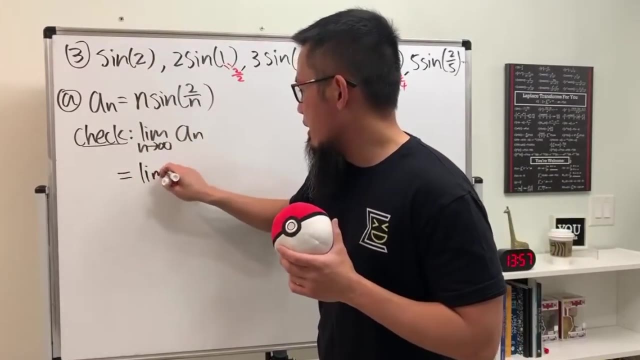 Two over n, Does this converge? Well, let's type a look. We are going to check the limit as n goes to infinity of a n. right, This is how you check if a? n converges or not. So check the limit as n goes to infinity. 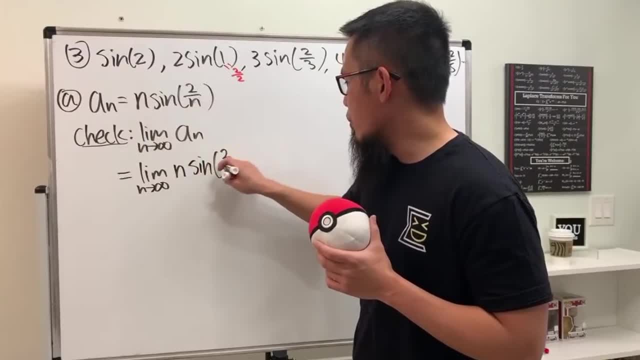 a n is that which is n times sine of two over n. Now we have a small trouble because if you put infinity to here Now we have a small trouble, because if you put infinity to here, Now we have a small trouble because if you put infinity to here, 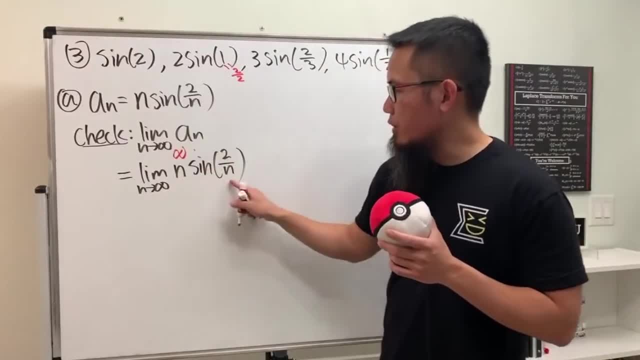 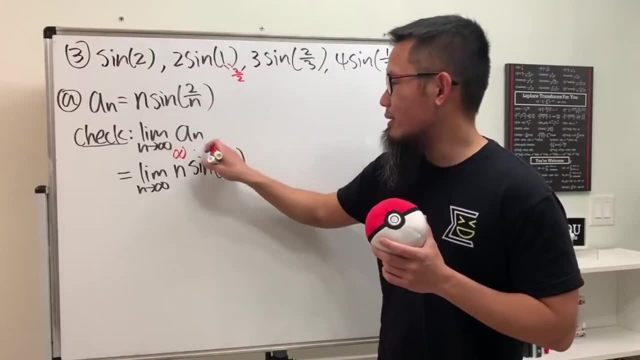 we get infinity. And if you put infinity to here, two over infinity is zero. And if you put infinity to here, two over, infinity is zero. Sine of infinity is So sine of zero is zero. So this is actually an infinity times zero situation. 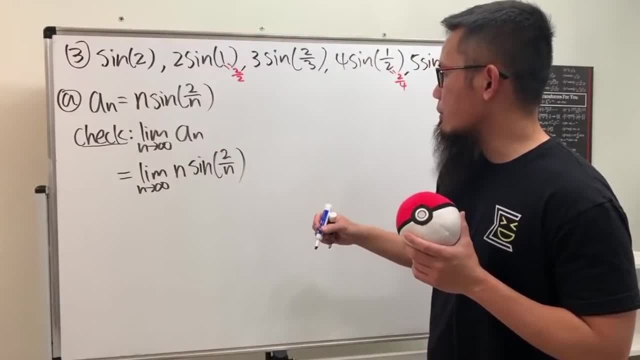 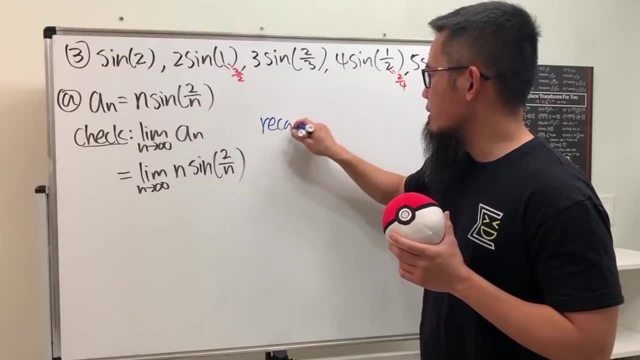 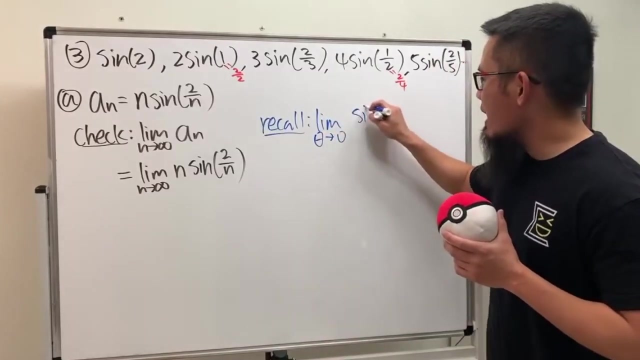 I'm going to remind you guys what a secret weapon is. Perhaps I will do it right here: Recall, Yeah, recall. This is one of the secret weapons. The limit, as theta goes to zero sine theta over theta, this right here, is equal to 1.. Alright, and please do not do. 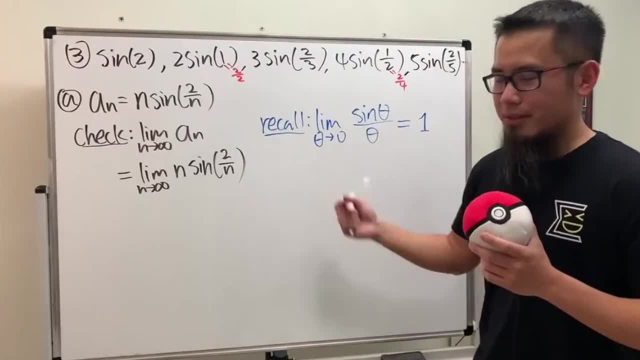 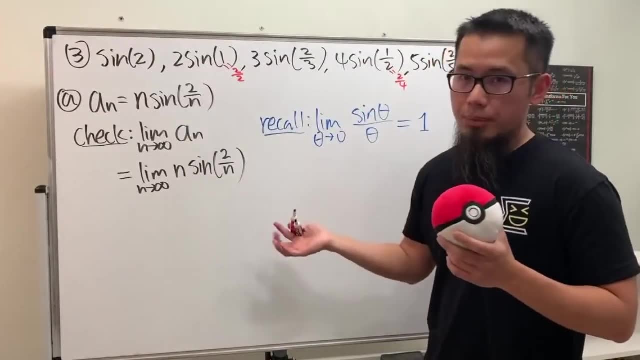 L'Hopital's rule for this: just use this, and then we'll not chat up here. So for this right here we can actually do some substitution and we can put this into this form and that will be it. And the way to do it is we can let theta. so I'll just 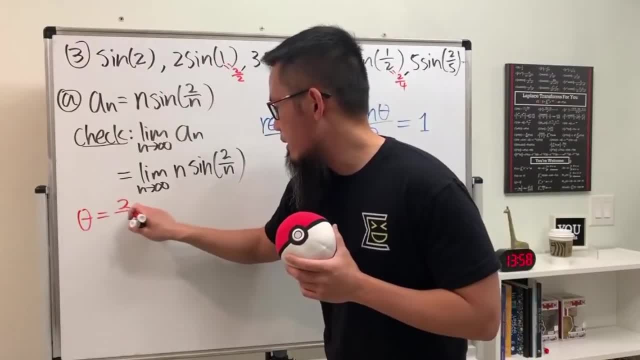 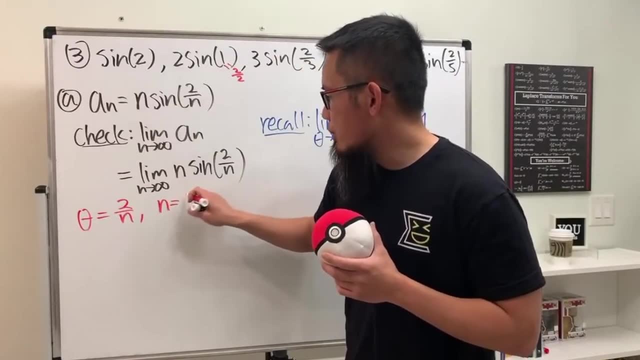 put this down: let theta equal to 2 over n, and of course we can just multiply n on both sides and divide theta on both sides, then you will see that n is equal to 2 over theta And because n goes to infinity, you can see that if you put that right here. 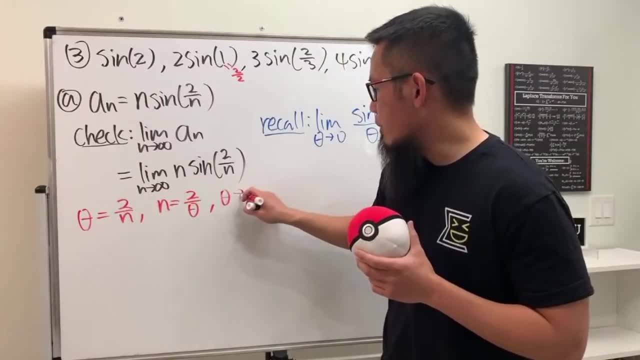 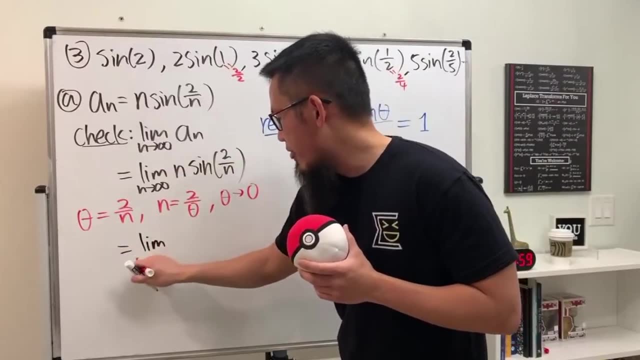 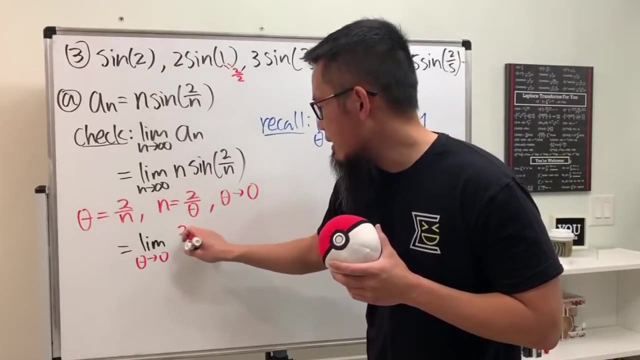 2 over infinity is 0, so you can see that theta will go to 0. So we can take this limit into the theta world limit, as theta goes to 0 now and you see, n is equal to that, namely 2 over theta. And then here we have. 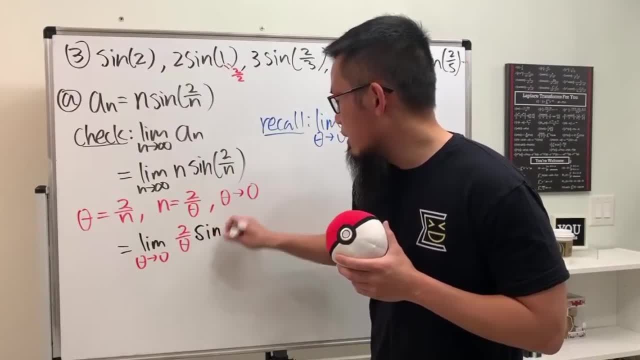 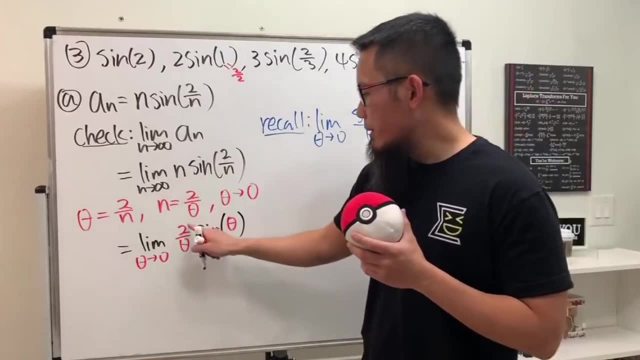 that, namely 2 over theta. And then here we have that, namely 2 over theta. And then here we have sine of 2 over n, which is theta, And cleaning things up a little bit, this is a constant multiple we can put in the front, So here we have 2 times the limit. 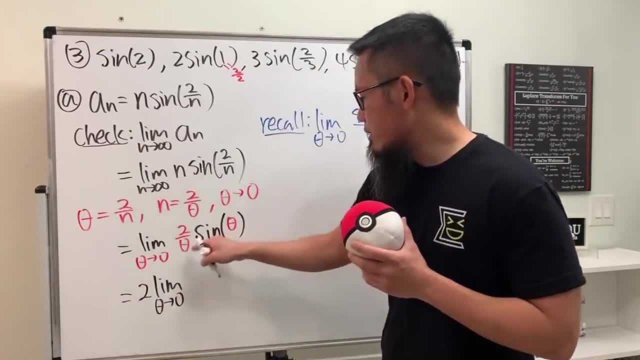 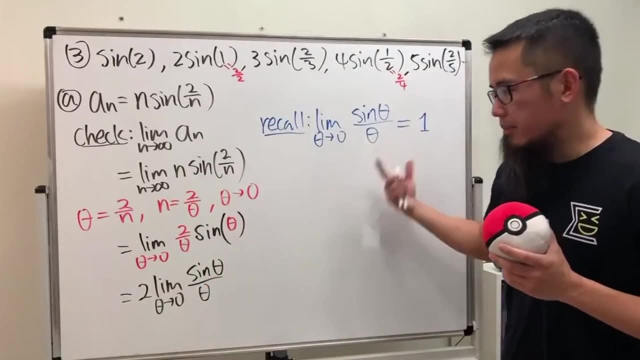 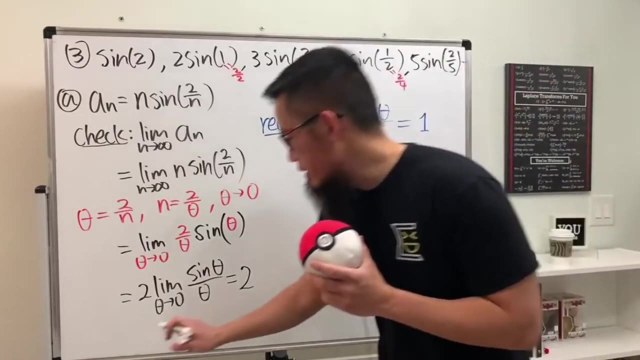 as theta goes to 0, and then put this over that, so we have sine theta over theta. Well, this right here is precisely the limit, and that will give you 1.. 1 times 2, we get 2.. So that's it. So, finally, we can say that a? n does converge and it converges. 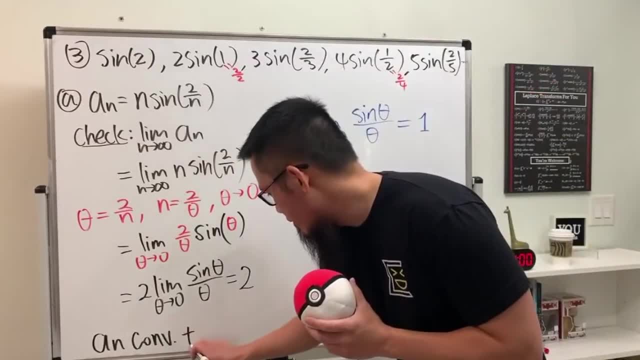 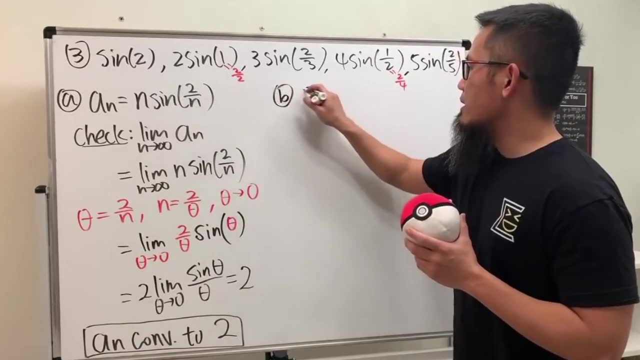 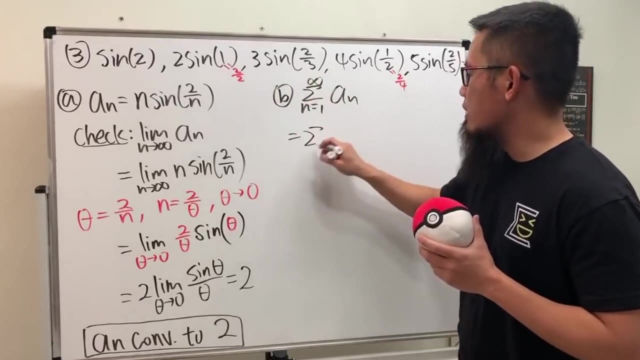 It converges very nicely to the number 2.. So this is it For part b. again, does the series as n goes from 1 to infinity of a, n converge or not? Well, I'm just going to write this down. Most likely later on you will see the question being asked like this: right, The 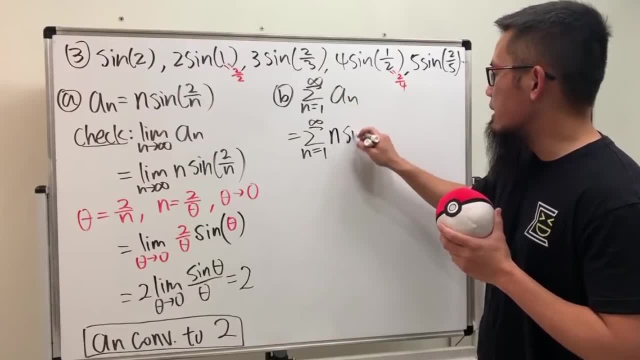 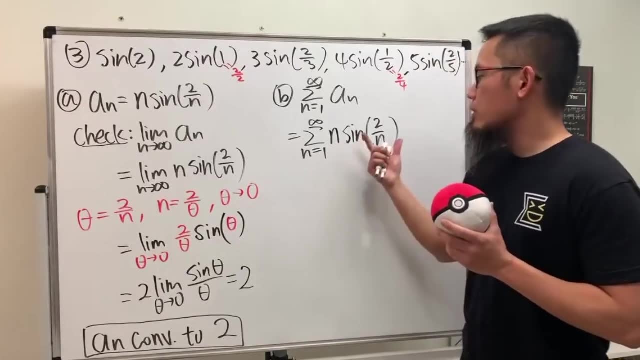 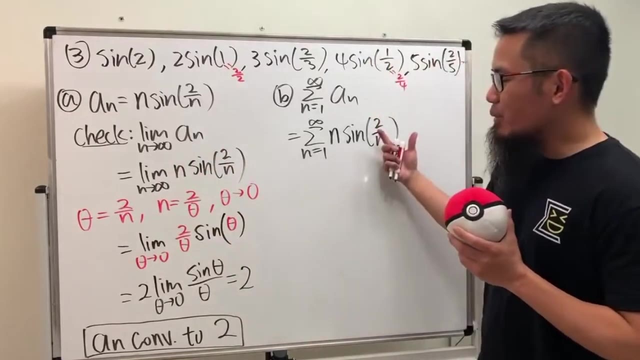 series, and then they will just put down the formula: n times sine of 2 over n. If this is what you are dealing with again, go ahead and take the limit on your own, but because you can do the test for divergence And you'll see that, hey, this right here. 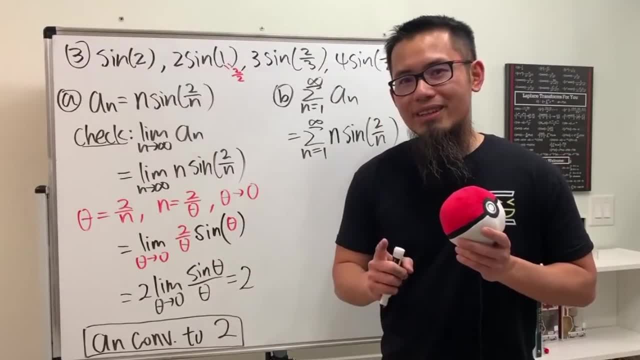 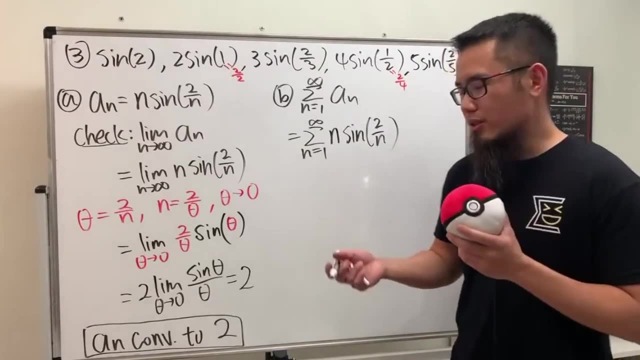 the limit is equal to 2,, which is not equal to 0. So does this converge or diverge? Yeah, diverges, Nice, TFD, right. We did that earlier And again. this is just how you can write down the answer, So you can say this right here. Diverges because 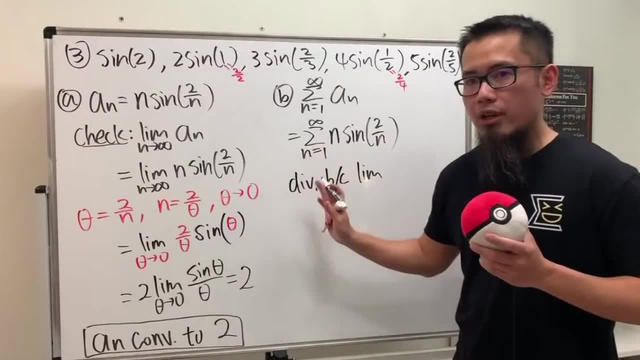 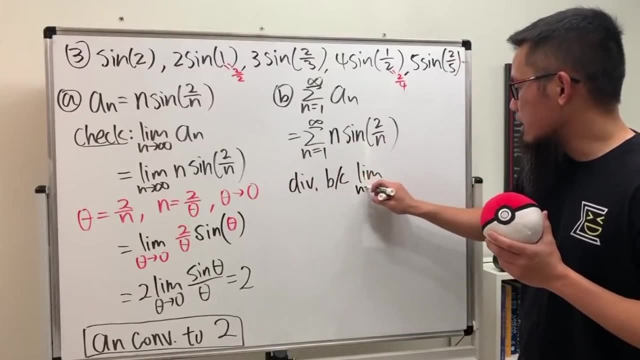 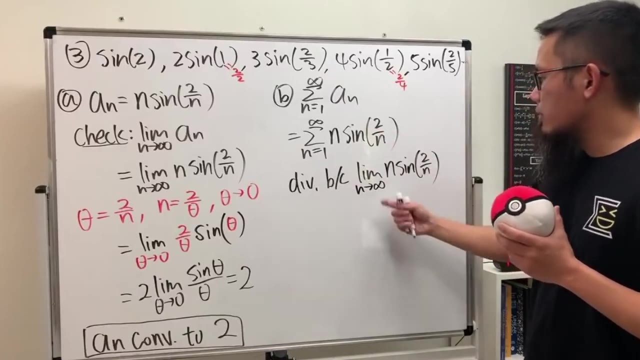 again, I'm just putting this down right here under the assumption that we are doing this on its own. So that's why you will just say the limit, as n goes to infinity, of that. you do a limit of this part, you put this down and you show that this right here is equal to 2,. 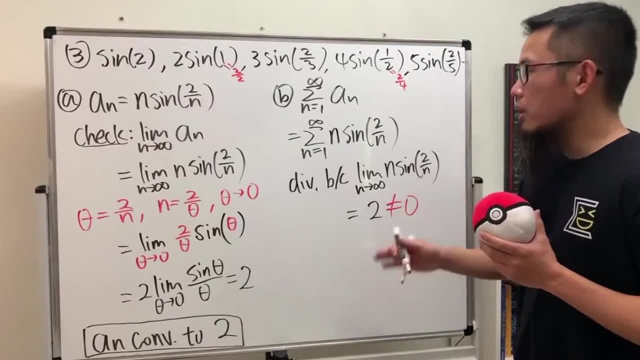 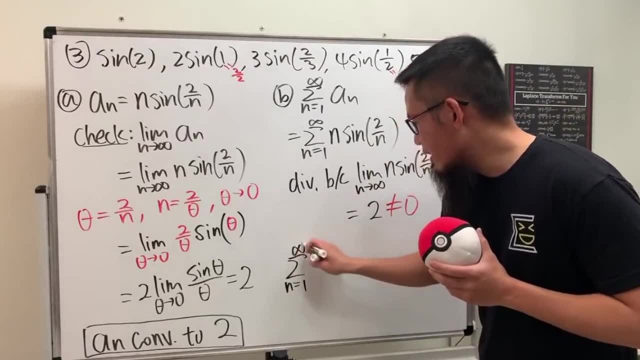 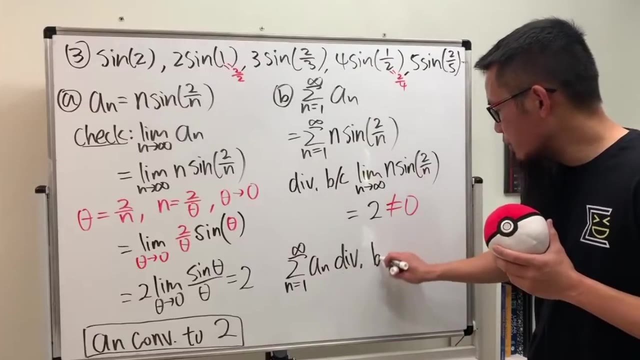 And again, 2 is not equal to 0.. Therefore you can draw the conclusion, And the conclusion is that the series as n goes from 1 to infinity of a n right. In this case this right here diverges and give a reason by test for divergence right. 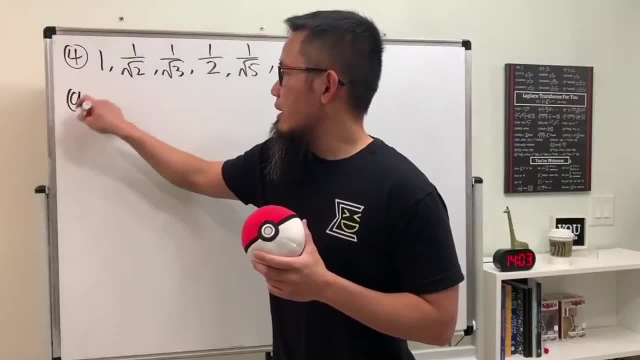 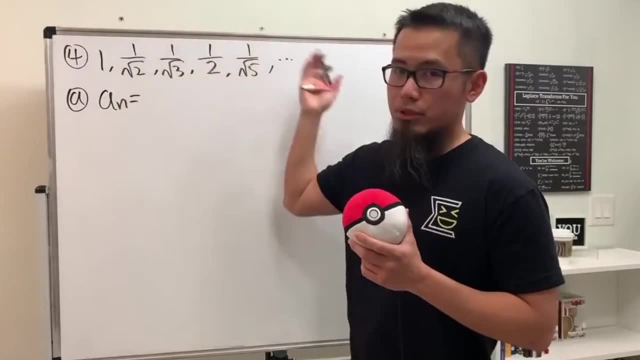 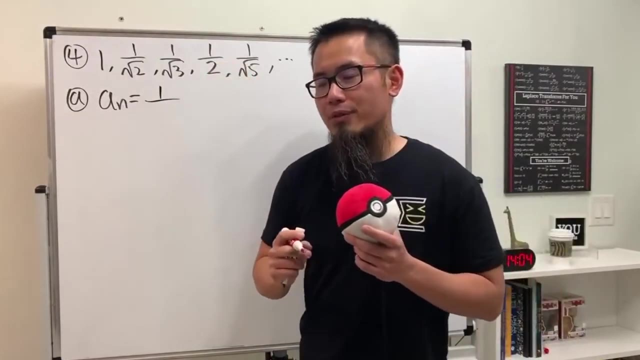 So that's how you can present your answer. Okay, a? n. right. First one figure of formula a n. everything on the top is just 1.. So it's 1 over this, 2. It's the same as square root of 4.. 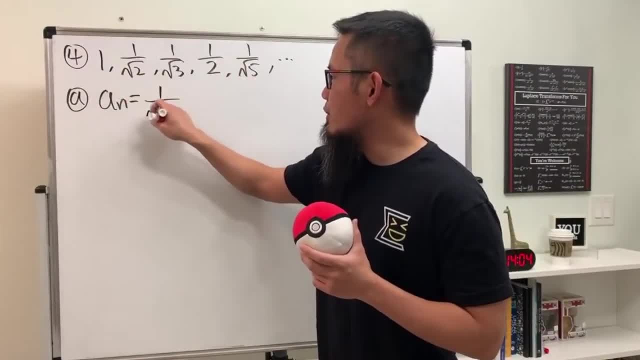 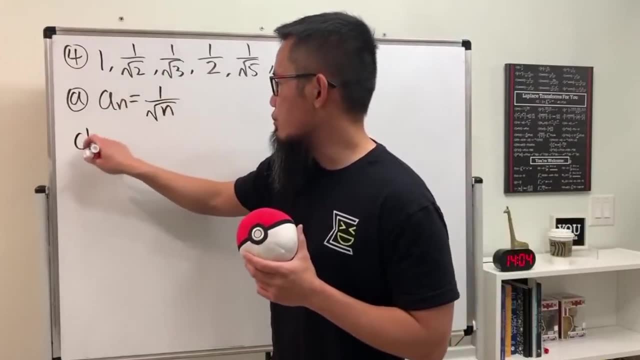 So all in all, in fact, this is just 1 over square root of n, right? So that's pretty clear. And again, does a n converge or not? Well, let's go ahead and just do the usual thing. I want to be consistent throughout this video. 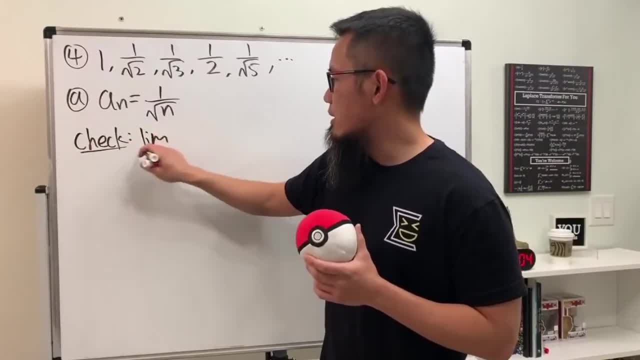 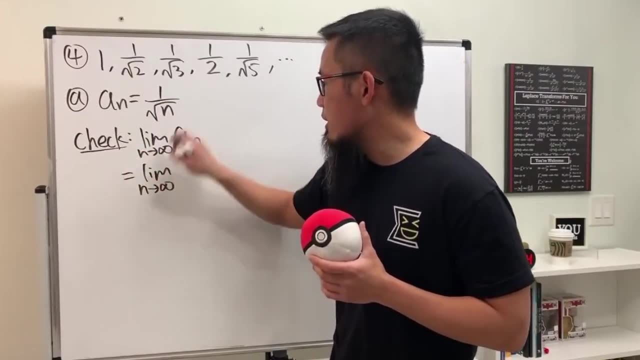 So that's why I keep putting down the check And we'll check the limit As n goes to infinity of a n, And this right here means we'll just check the limit as n goes to infinity of that right. Pull infinity to here. 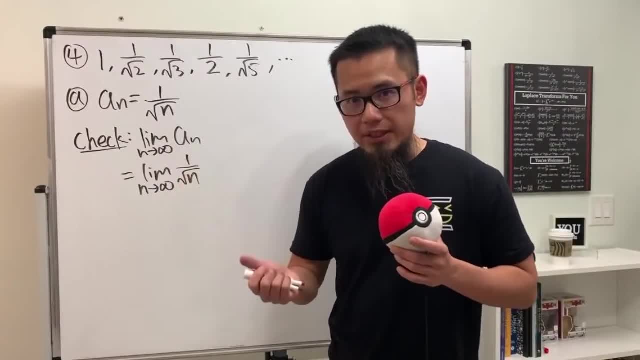 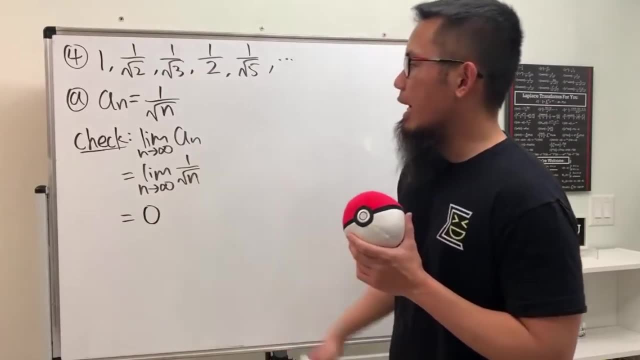 You can work this on your head: Square root of infinity is infinity. 1 over infinity is 0.. So all in all, this right here gives you 0,. all right, Good. So this means a n converges to the number. 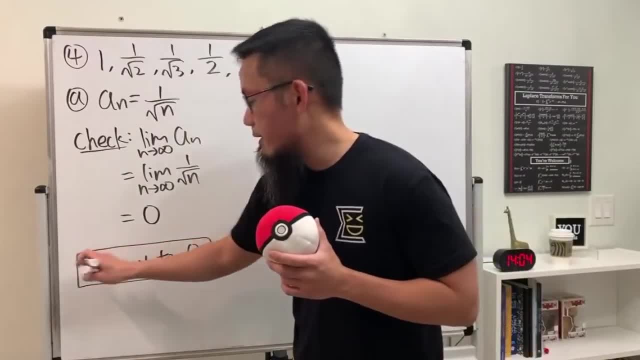 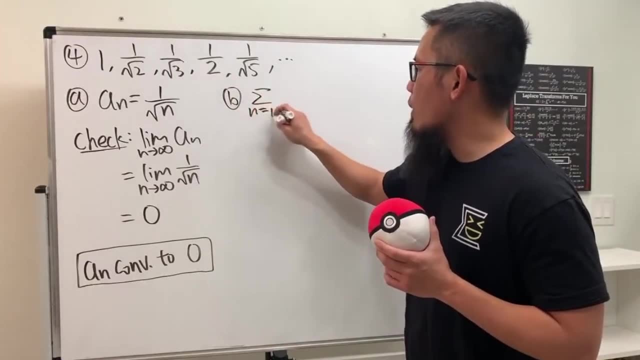 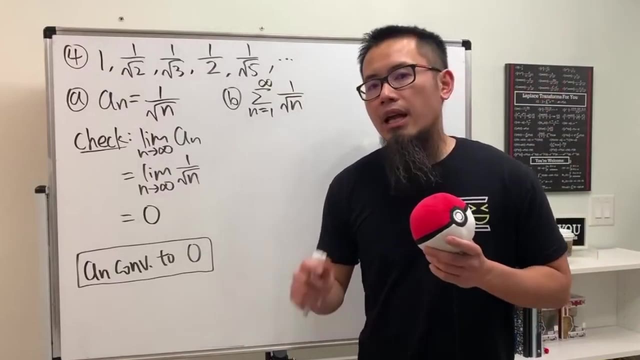 So this is very nice. right Now for the second part, we are going to see if the series as n goes from 1 to infinity, 1 over square root of n converge or not. I showed you guys two questions previously, right. 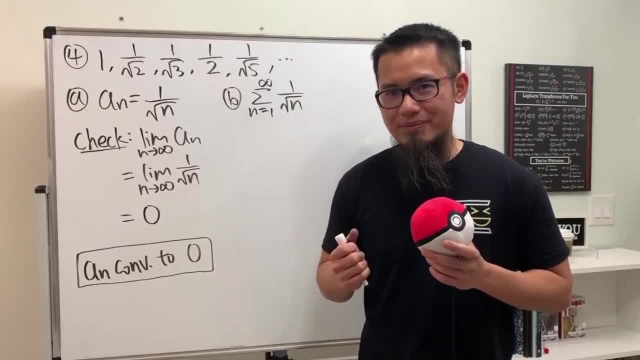 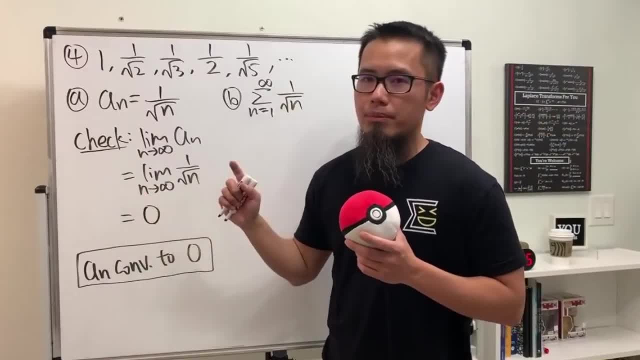 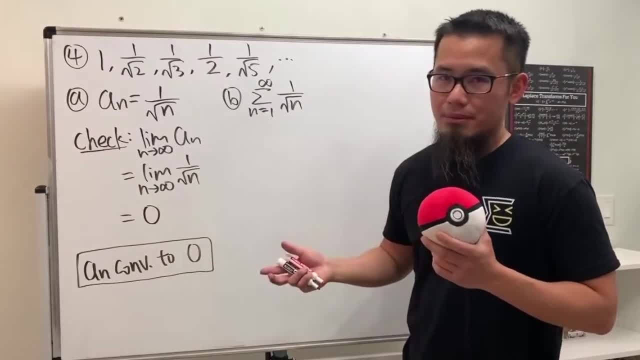 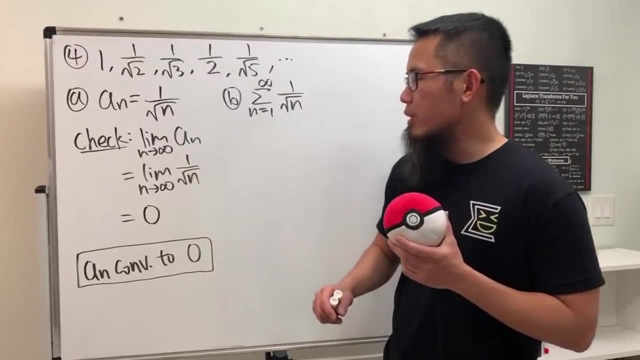 will converge right away. It does not mean anything If you see the limit of a n being equal to 0, we cannot draw any conclusion. The only place that we can draw conclusion is that if the limit of a n is not equal to 0,. 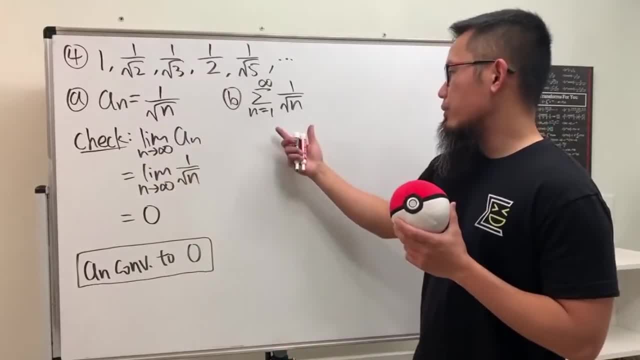 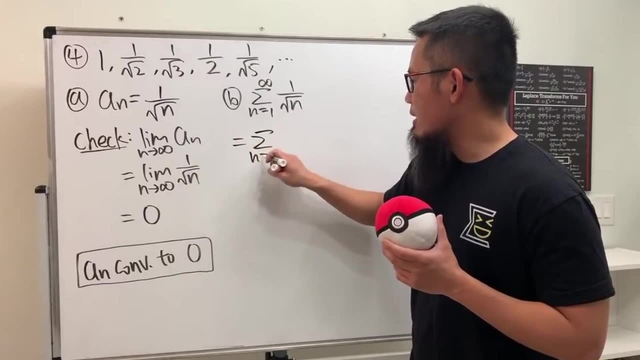 then that's the test for divergence. Well too bad in this case, but this is not so bad either, because the theory is this: right here: It's the same as A. the series as n goes from 1 to infinity of 1 over n. 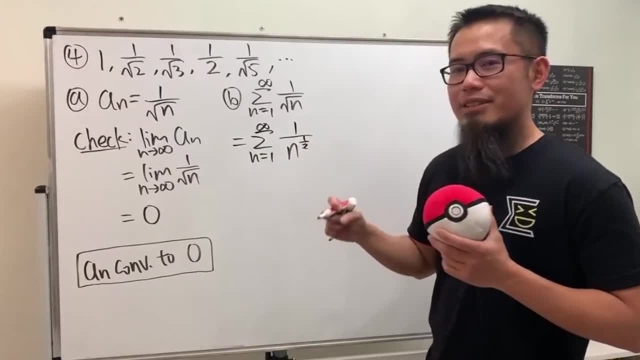 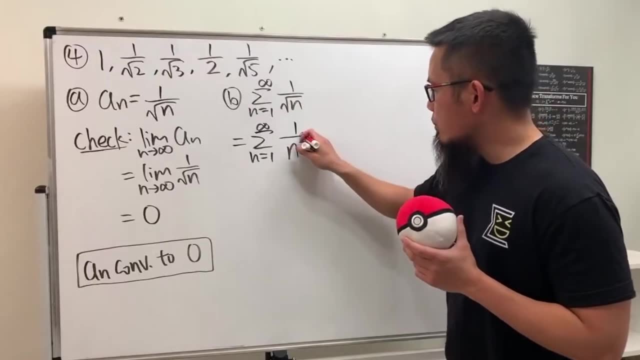 Square root is the same as 1 half power. So in fact, this right here is actually just a p-series, And this is how I usually show work to my students. I tell them to circle the power right here and just put down: okay, p is equal to 1 half. 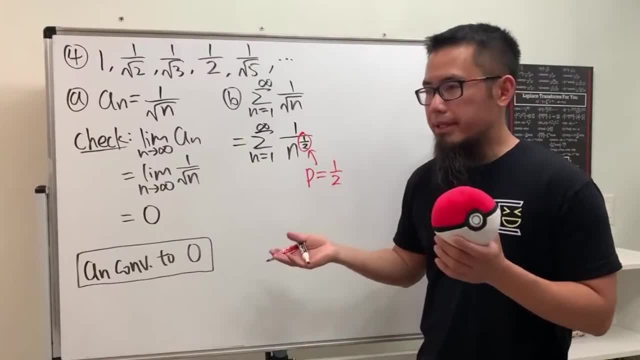 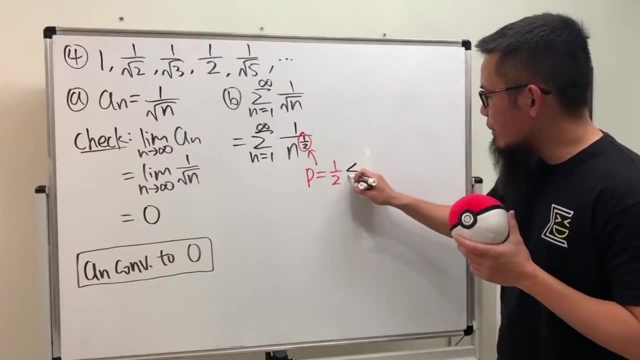 And when you put this down- I know that you are using the p-series, But do not just put down: p is equal to 1 half. Now you will have to tell me that 1 half is less than or equal to 1.. 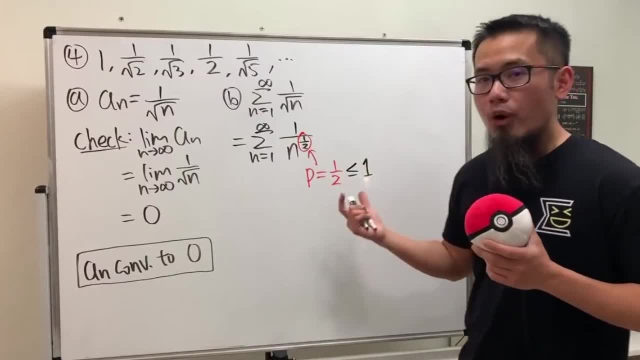 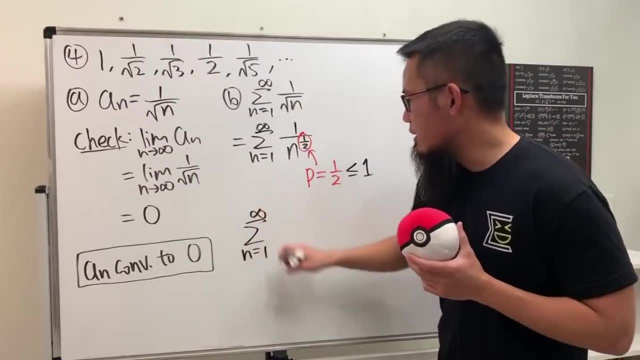 Because you are telling me that p is less than or equal to 1,. therefore this right here diverges. So right here we can just say: the series n goes from 1 to infinity of a n. So this right here actually diverges. 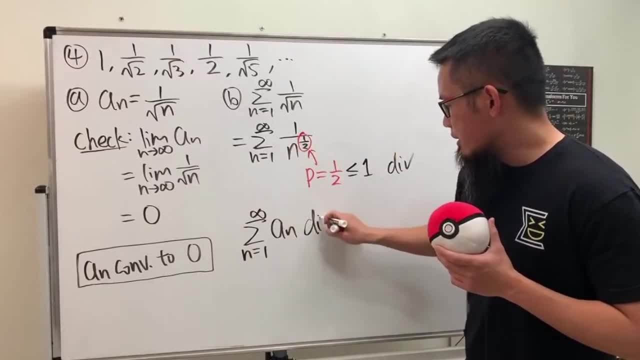 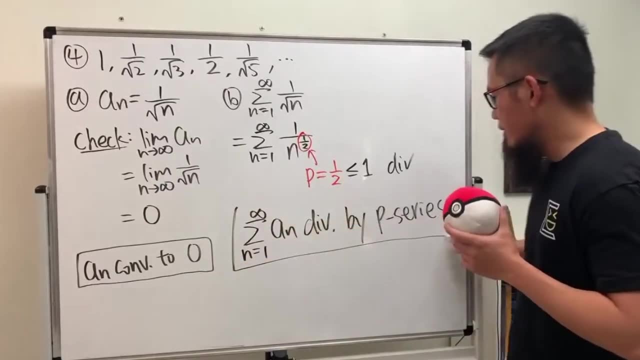 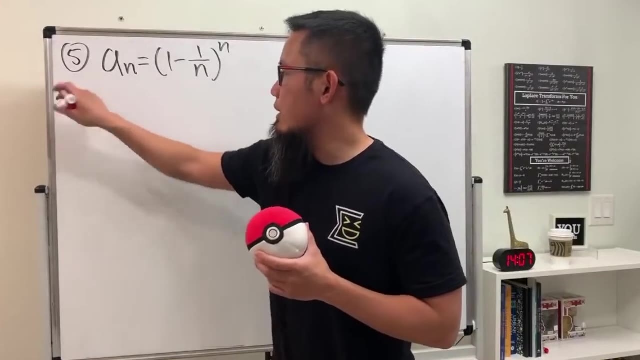 So I just write down this right here: diverges And we can just say by p-series: All right, So this is everybody's favor. I will say First part: does a? n converge or not? Well, we will just check the limit. 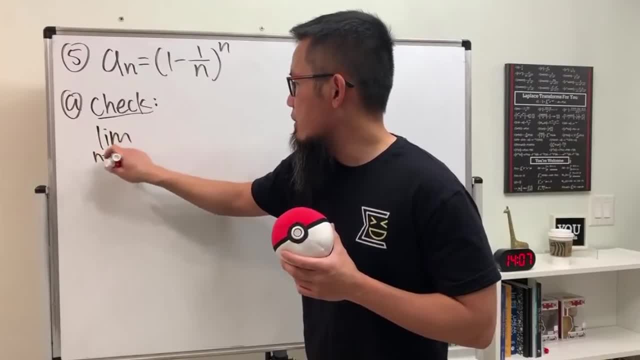 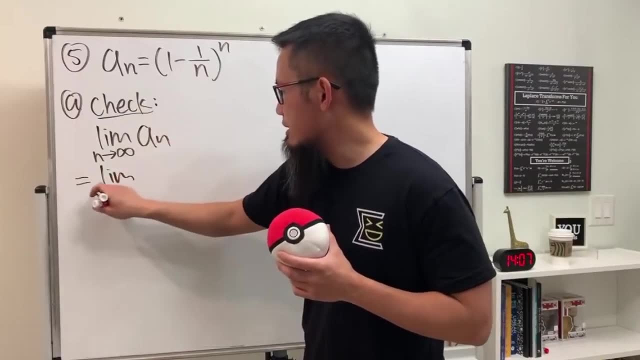 I'll just put this down right here, As n goes to infinity of a n, Right, So this right here means we are going to check the limit. as n goes to infinity a n, is that? so just write that down, All right. 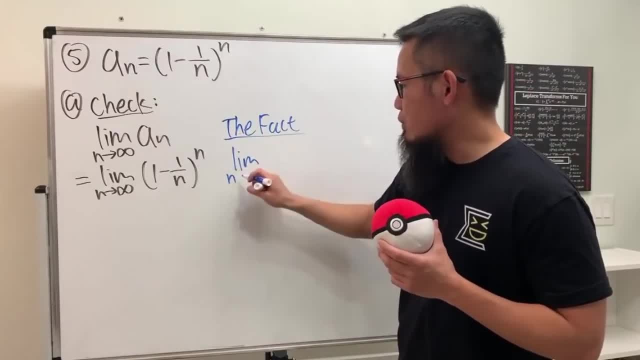 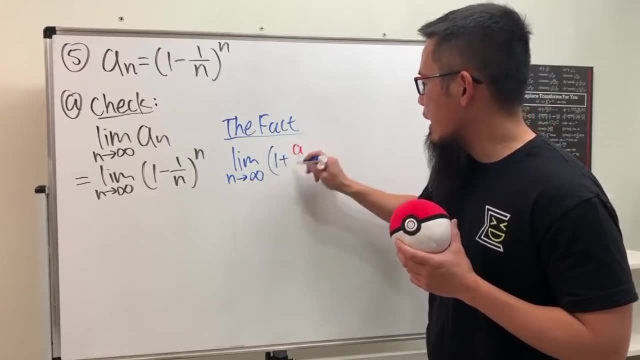 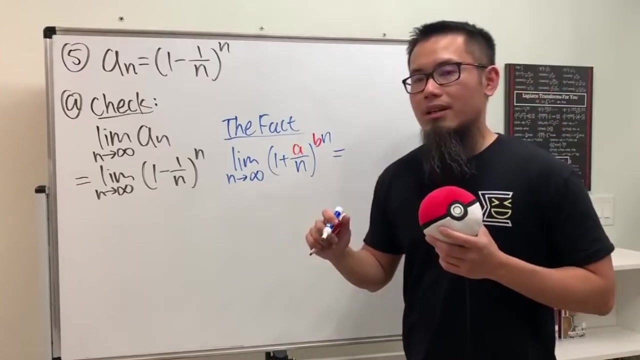 The fact is, if you have the limit as n or x, whatever letter that you're using doesn't matter, Goes to infinity. and if you have 1 plus a over n, raised to the b? n power, This right here it's equal to e to the a? b power. 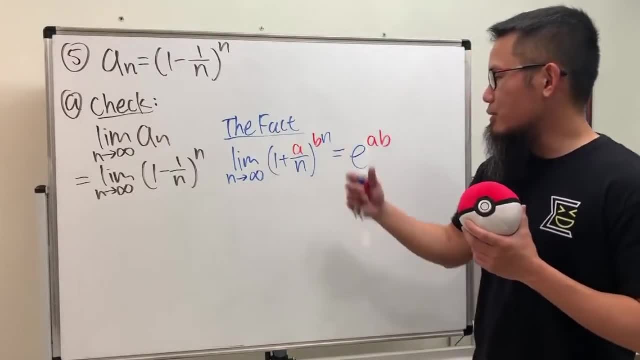 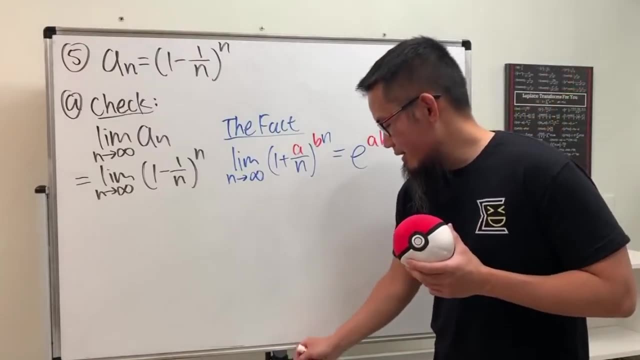 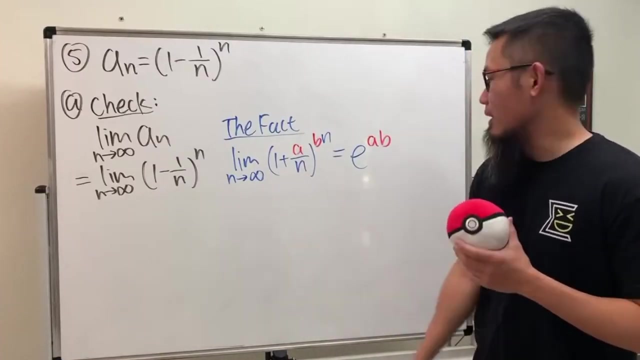 It's very nice And for my class, I tell my students this so you can use it without showing any other things. It's because it's convenient, and I also make them do the proof of this so they know how this is true, and after that we'll just use this as a formula, right? 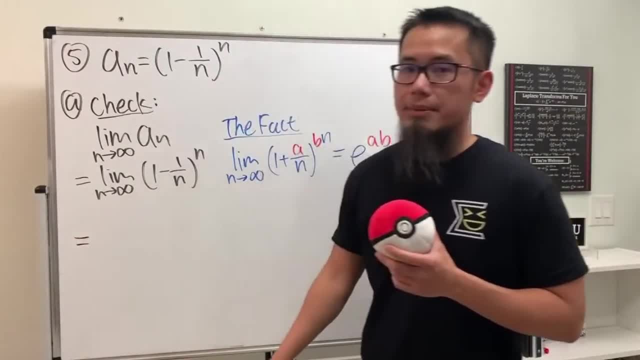 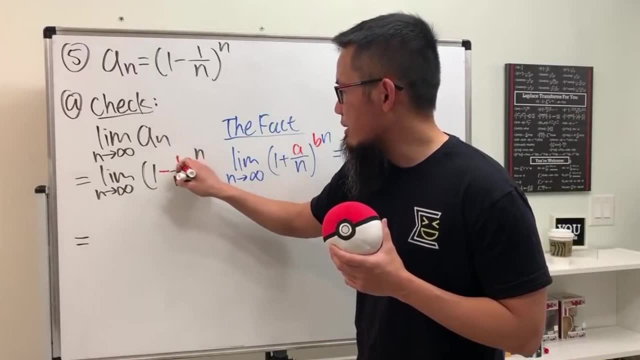 So in this case, this is how it can show work, especially if you're in my class, Notice this right here fits into this form and pay attention to the. a value is actually negative 1.. So you'll just write down: a is equal to negative 1, right, a is equal to negative 1.. 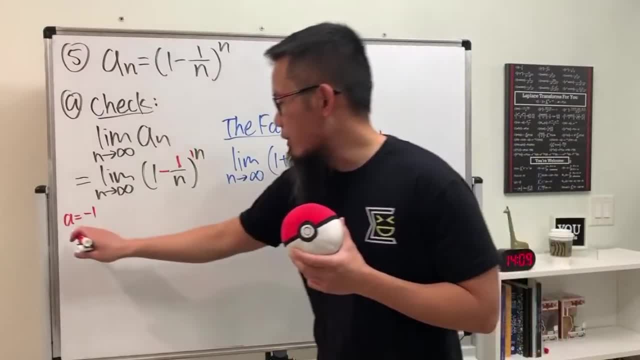 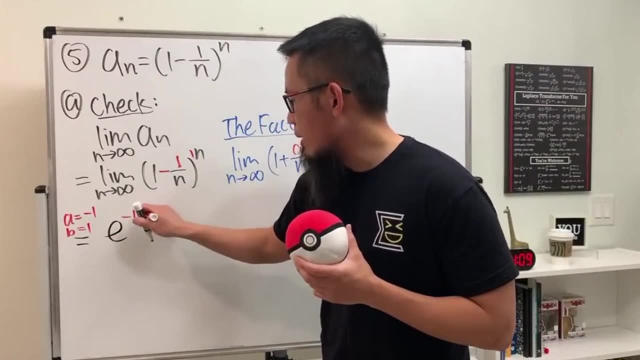 And then the b value is just 1, so you'll just write down: b is equal to 1.. So all in all, you can just write down: this is equal to e to the negative 1 times 1 power. Of course this is just equal to e to the negative 1, and that's 1 over e, right? 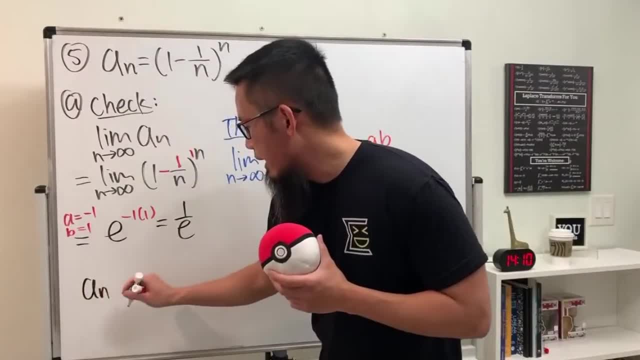 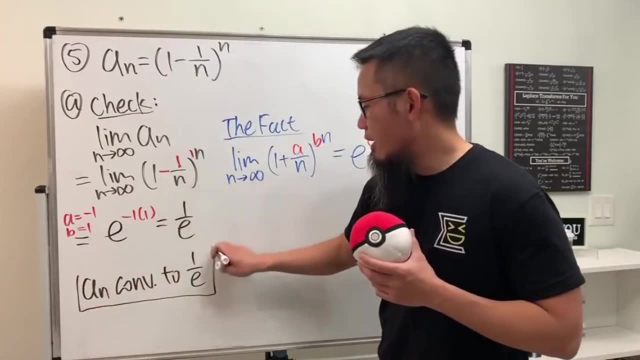 Therefore, we know that a? n does converge, so let's put that down: a n does converge and a? n converges to 1 over e. All right, And I think some of you guys are very happy about this already, right. 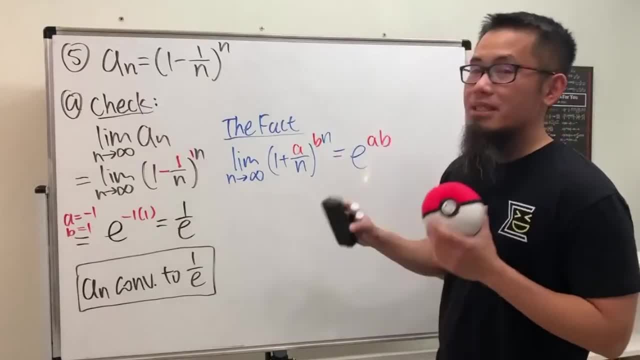 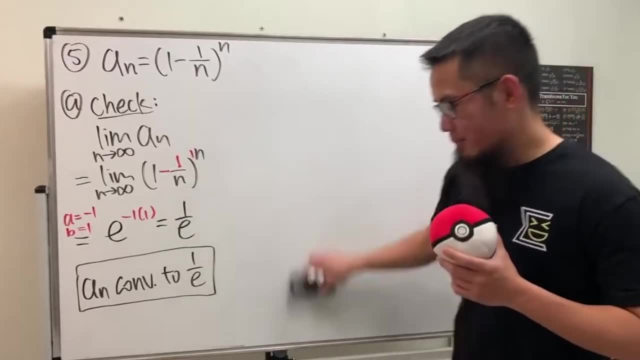 Anyway, this is the fact. Earlier I called that limit the limit. If you guys have seen this before in my old videos, thank you. And if you are taking Cal2 for the first time and you're watching this for the first time, then you know that's one of the things that you'll see. 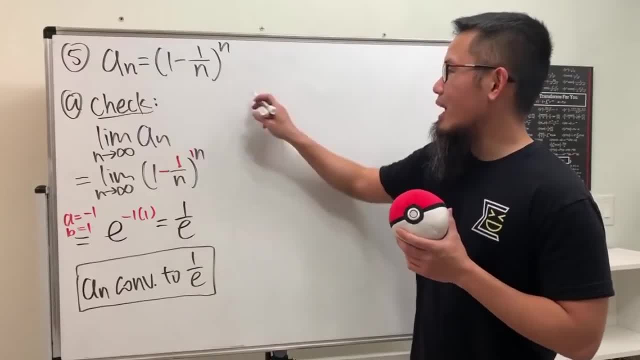 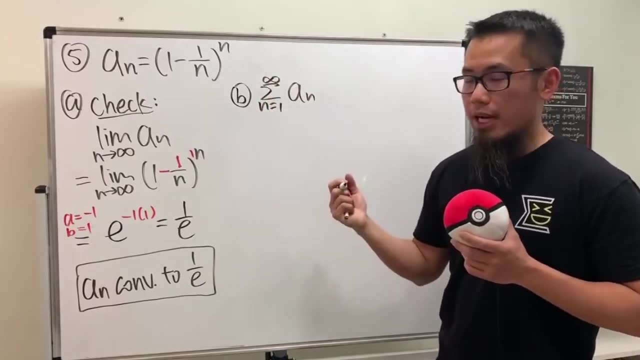 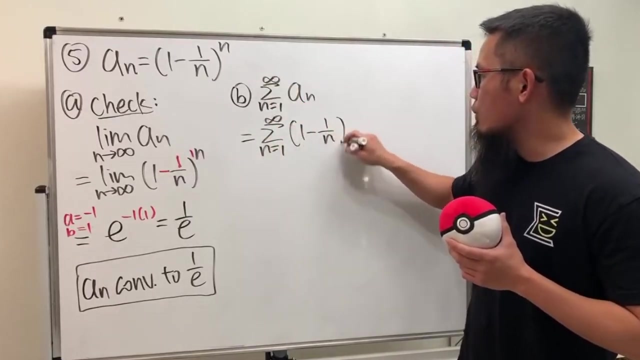 Okay, that's a? n converges. Now part b: Does the series of a? n converge or not, right? So again, this notation: does this converge or not? This is asking us to do the series, as n goes from 1 to infinity, of 1 minus 1 over n raised to n's power. 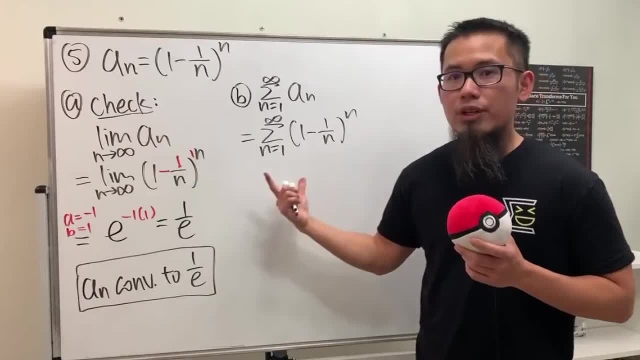 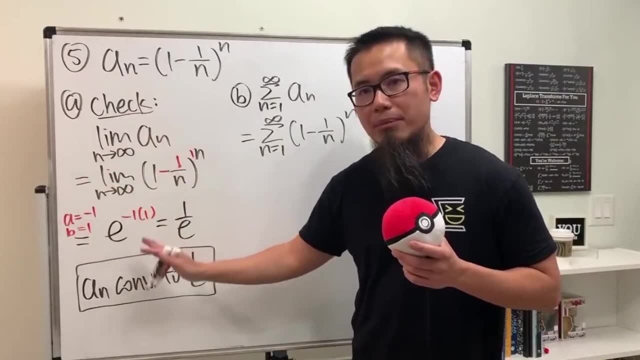 One more time. you're going to see just this for the question, And when you see that what you do is do the limit on your own, on the side, And then you see that the limit is equal to 1 over e, which is so nice, isn't it? 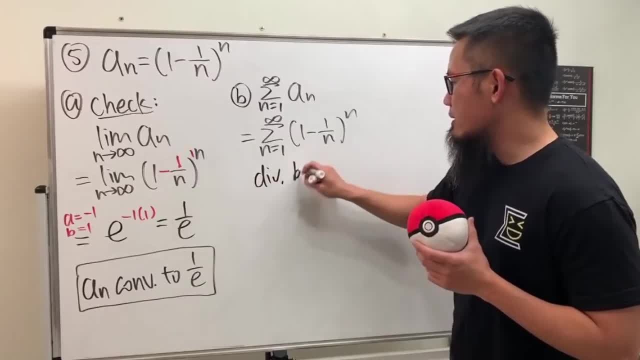 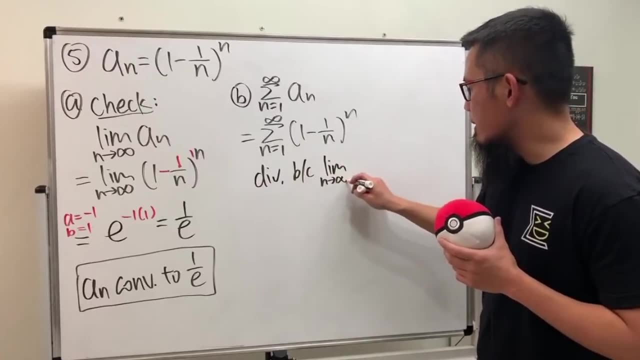 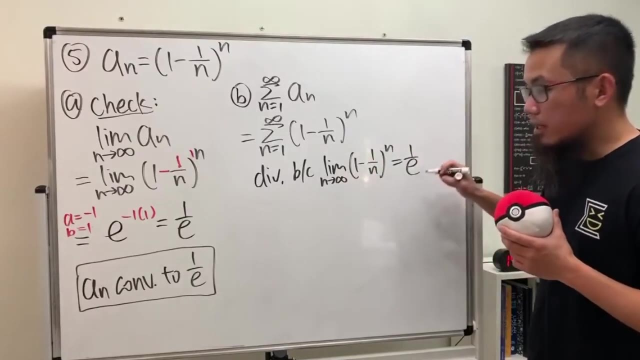 Because you know this right here, diverges Because, again, supply that if you are doing this on its own, Because the limit, as n goes to infinity, of 1 minus 1 over n, raised to n's power, this right here is equal to 1 over e, which is not equal to 0. 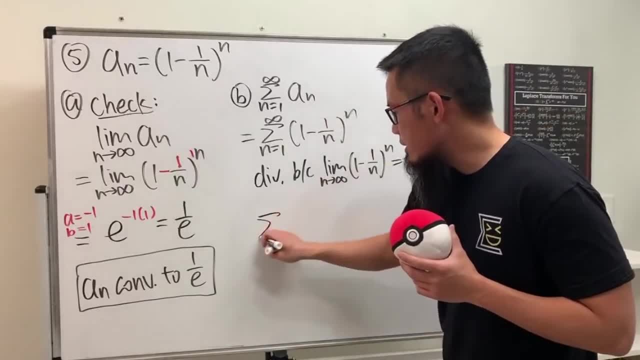 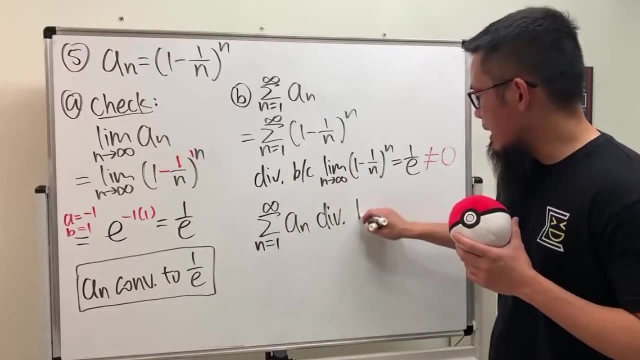 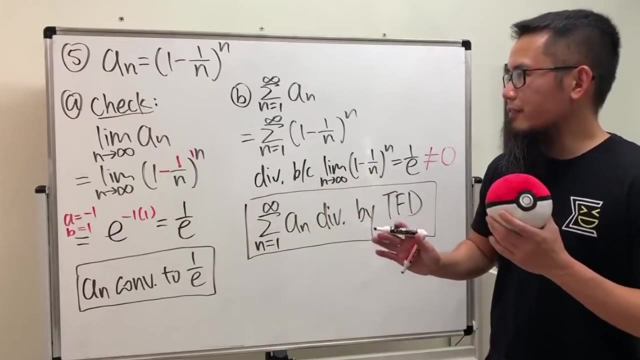 Therefore we can just say: the series n goes from 1 to infinity of a n. This, right here, Diverges by test for diverges. So hopefully, by doing these five questions already, you'll notice the difference between a n converges versus the series of a n converges. 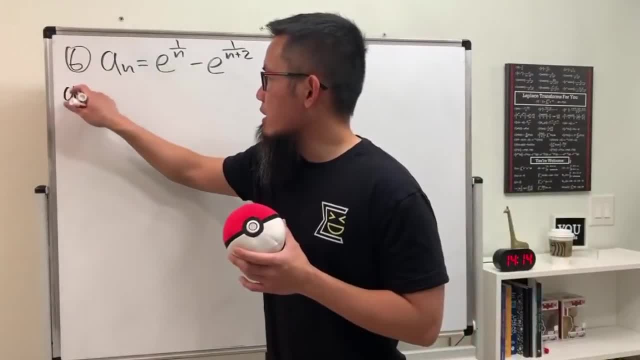 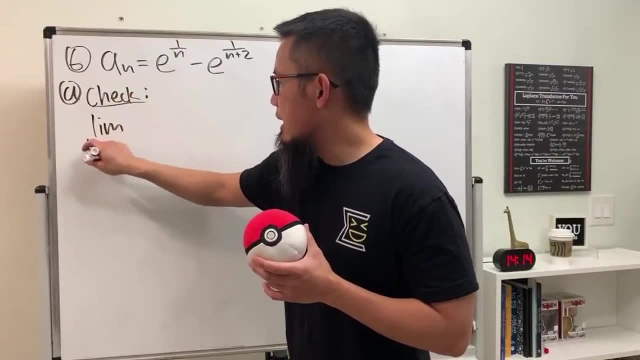 So this is the formula that we have Again. first part: does a n converge or not? So let's go ahead and just do the check. So we're going to check the limit as n goes to infinity, and then just this right here, right? 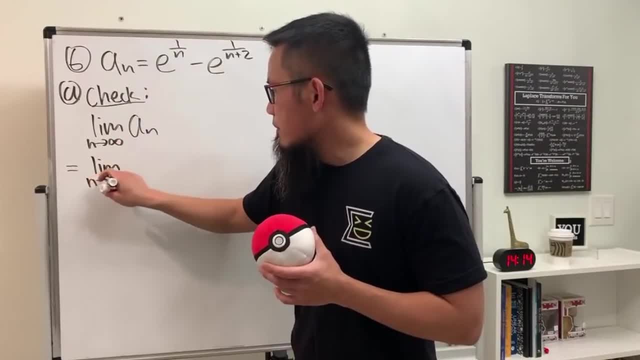 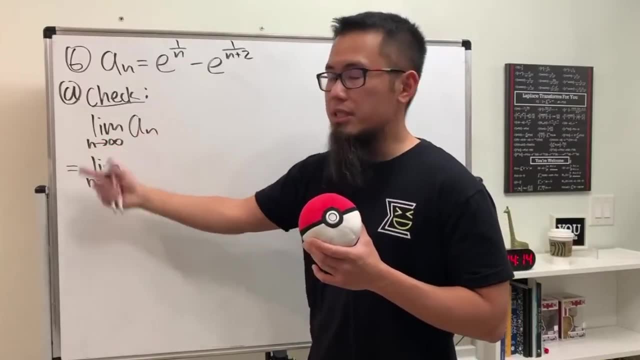 So a n, And notice that I always write this down in this video because I just want to show you if you need to check if a? n converges or not. You have to do this, And then the next step is this, which is that 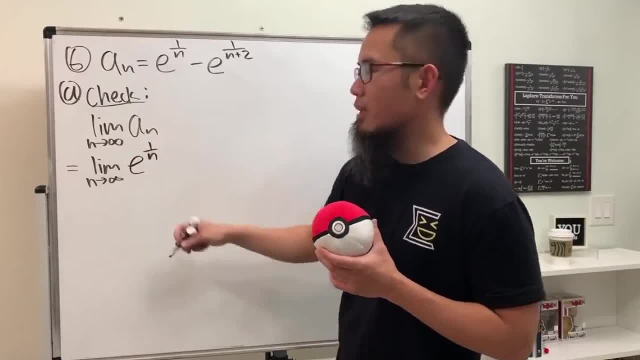 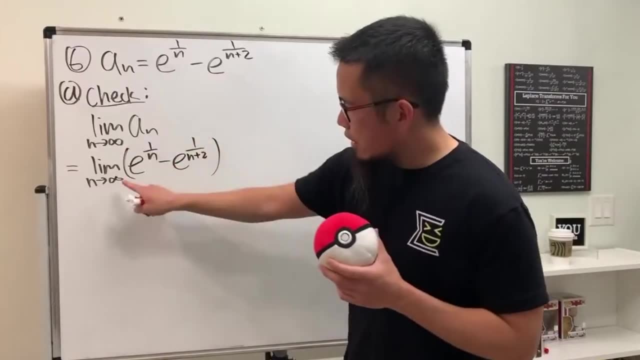 So you can skip this part if you would like. but anyway, All right, Now check this out. If you put infinity to here, you get. Let me just put this down so we can follow along. We get e to the. 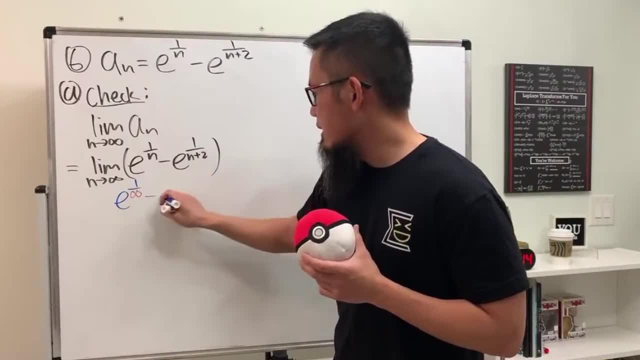 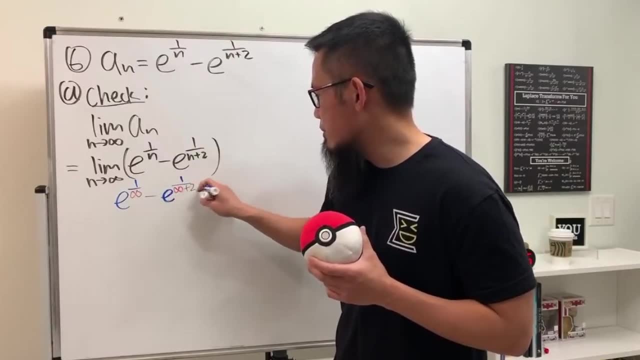 1 over infinity and then minus. e to the 1 over infinity, plus 2, right. So that's pretty much the idea. But this right here is just 0. So e to the 0 is just 1.. And then minus. 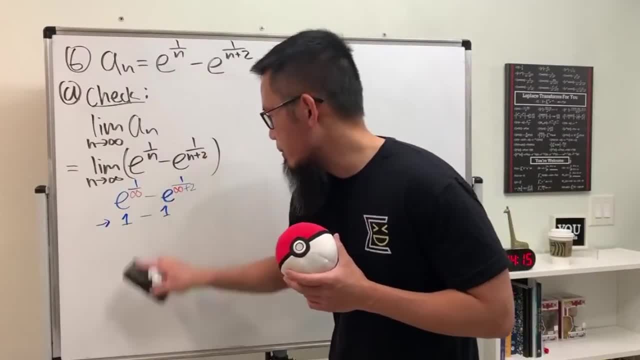 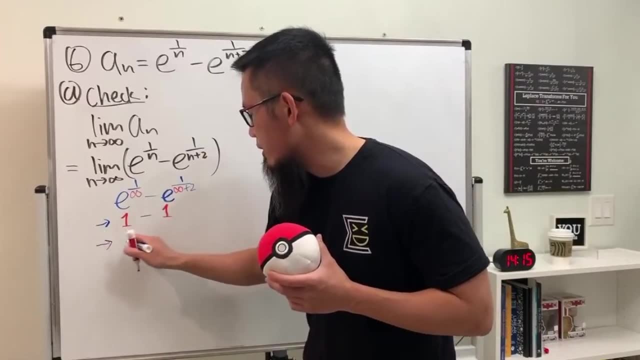 Again, this is also e to the 0,, which is just 1.. Perhaps I'll put this down in red, Sorry about that. This right here is 1.. This right here is 1.. So finally, you can conclude that this right here goes to: 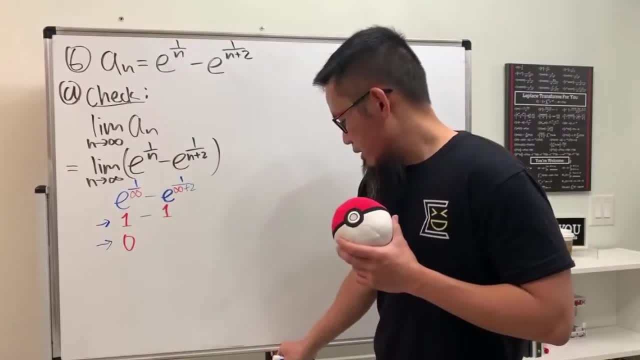 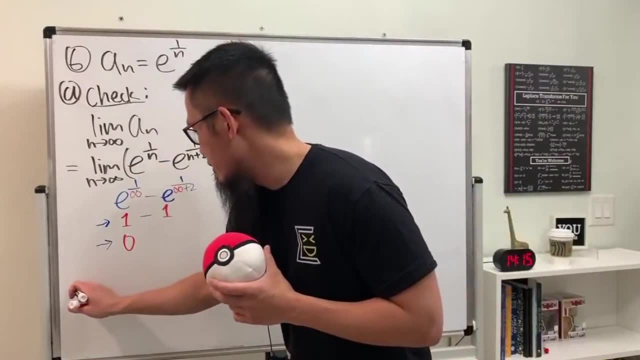 0, right. So if you want to show some kind of work, that might be okay. But anyway, though, this right here is also pretty clear, that it's just equal to 0.. So does a? n converge? Yes, a n converges. 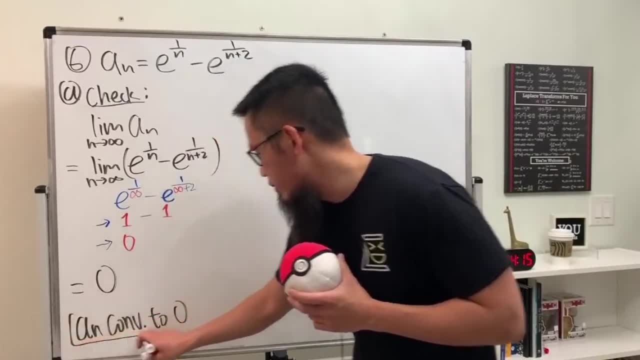 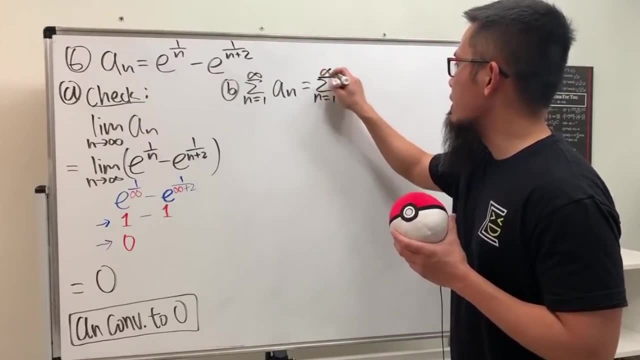 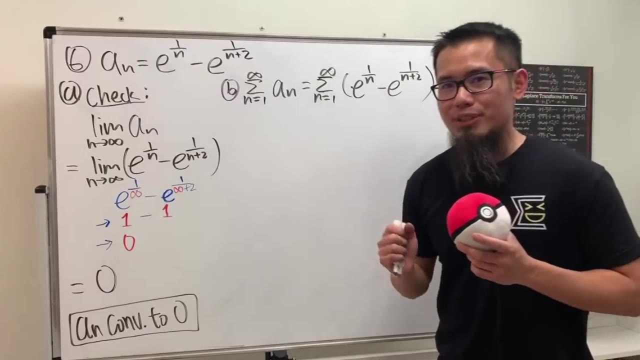 And we know that it converges to the number 0. Perfect. Well, this right here is the series, as n goes from 1 to infinity. And again, I'm just going to write down the AM formula. For the first time of the day, this is a telescoping series. 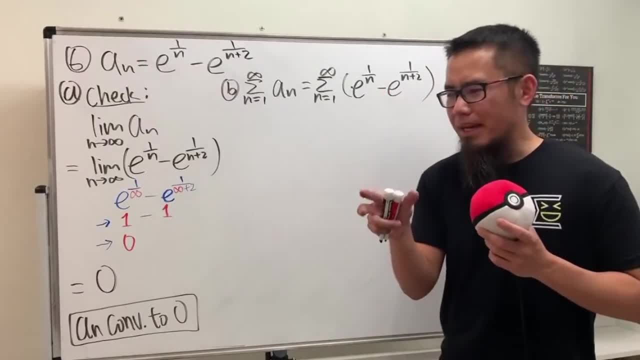 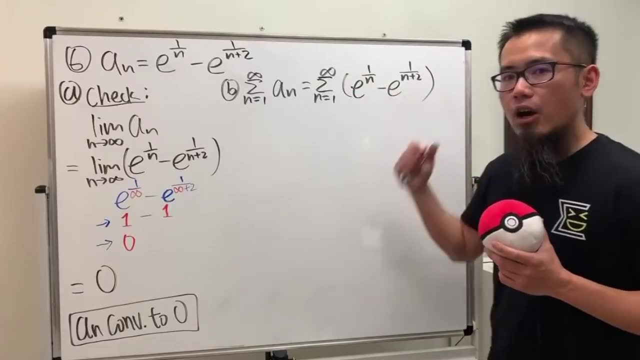 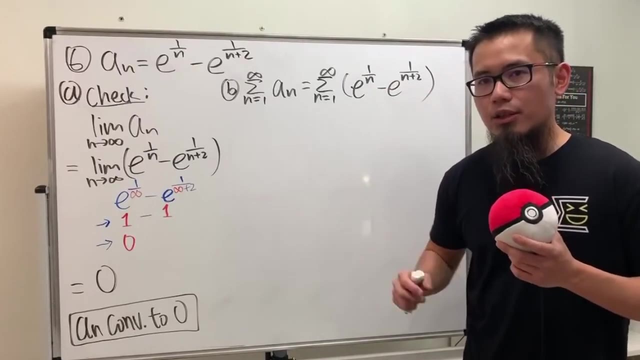 Why? First, the subtraction might give you a big hint, right, So pay attention to that. But more importantly, notice that this and that they are of the same kind, but they're just all by 2.. So that's why this is a telescoping series, right? 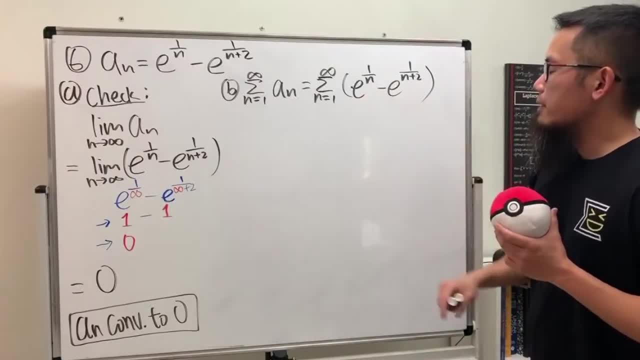 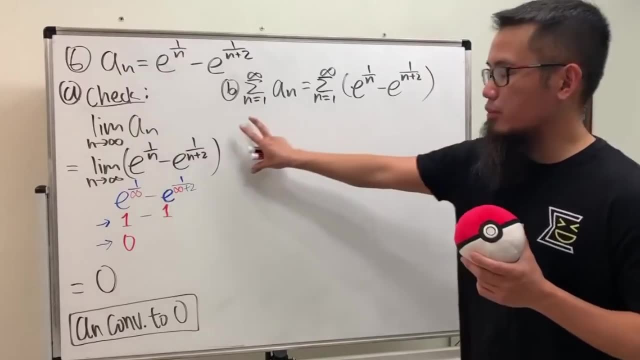 So that's the idea for that. Now check this out. This is how we can do it. I'll show you guys a fast way to get the answer, and then I will show you guys why this is true. So I'm going to leave a space right here, right. 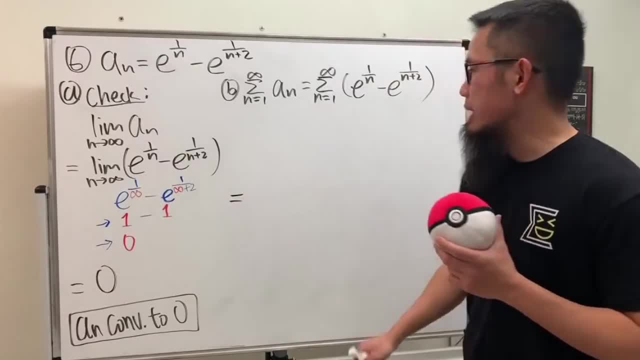 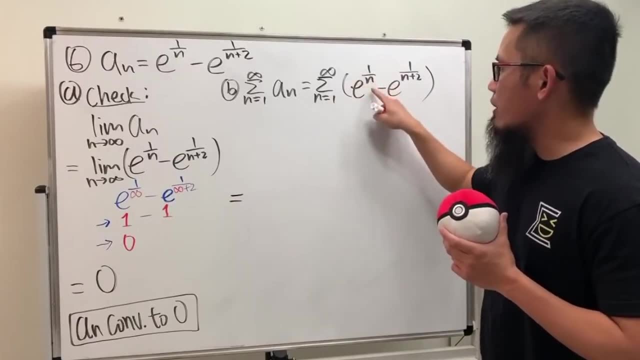 So this right here. the fast way to do it is pay attention to the starting n value, which is 1. in this case, You are going to put the 1 into the first term, right here. So I'm going to write it down like this: e to the 1 over 1, right. 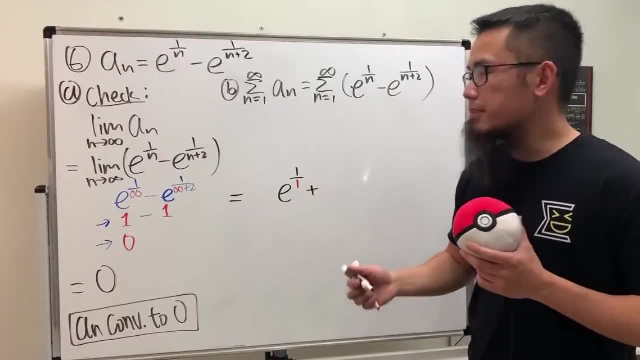 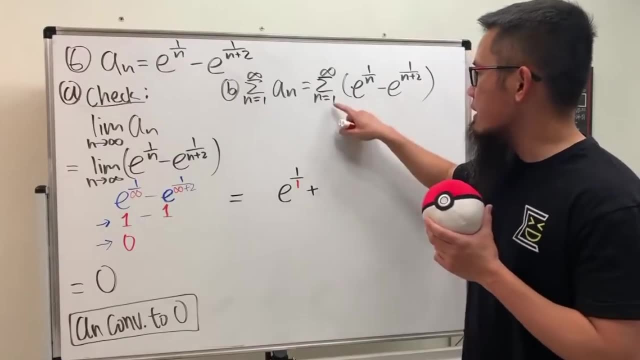 And then we are going to add, and the reason that we have to add is because they are of by 2 terms. So we have to do this twice. The first thing is n is 1.. You put a 1 in here, which we did. 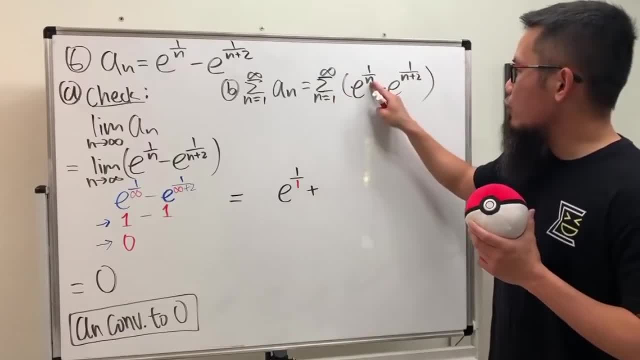 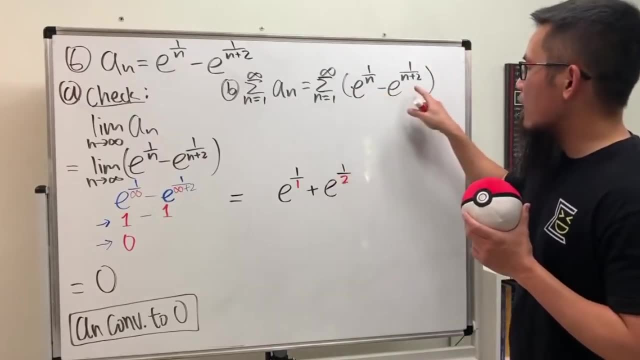 Then the second thing is that when n is 2, you put that right here and then you add them up, So we have e to the 1 over 2, right, And again because they are of by 2, that's why you do this twice. 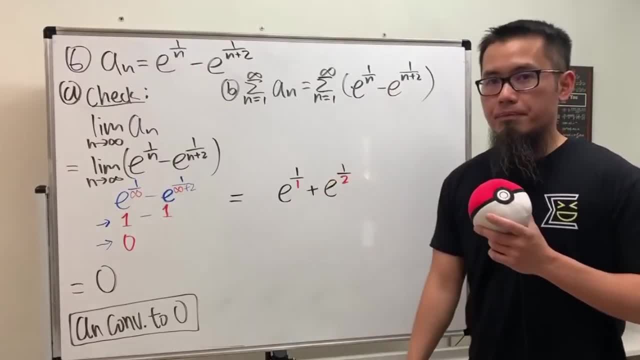 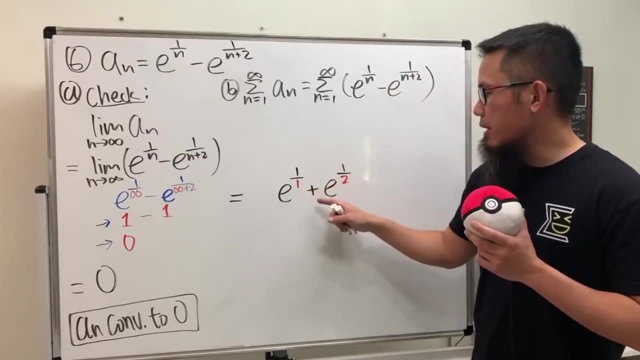 n is 1, put it here. n is 2, put it here. You can imagine: if this is n plus 4, then you do it 14 times. Then you end up with e to the 1 over 1, plus e to the 1 over 2, plus e to the 1 over 3,, plus e to the 1 over 4.. 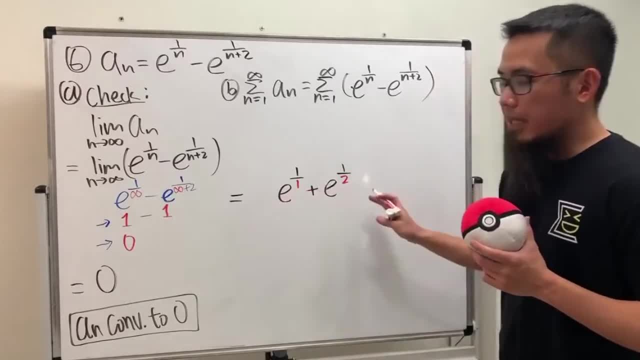 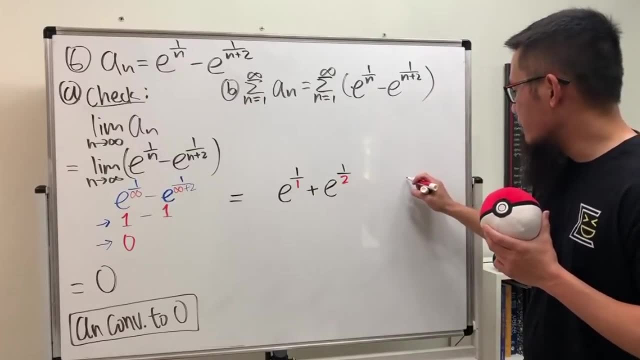 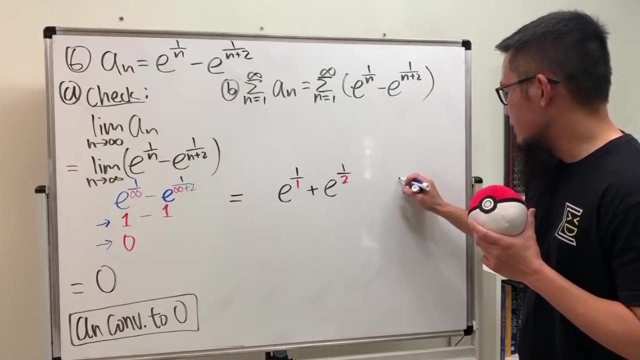 That's the idea. Okay, but this is not it yet. What you want to do next is write down the last term right here, and that's minus. So you're just going to write down: we are going to minus, so put this down in blue: minus, yeah, minus. 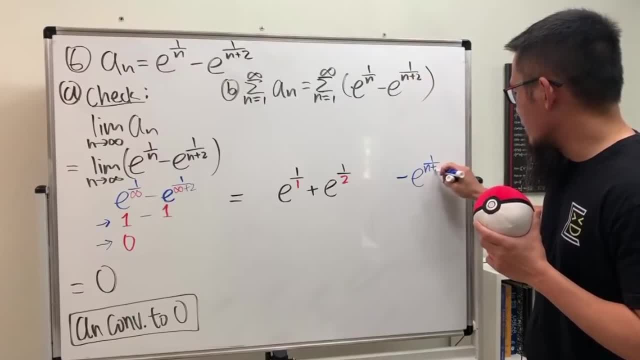 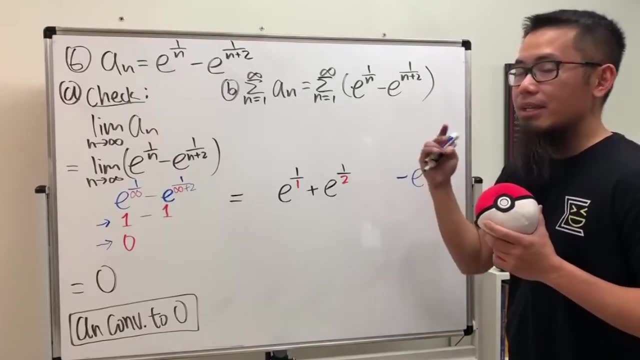 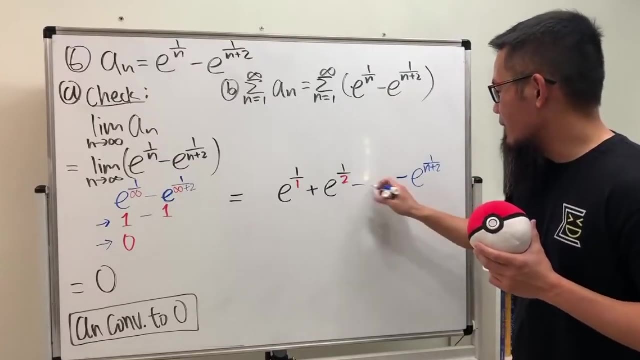 This term, which is e to the 1 over 2.. n plus 2,. right, You put down the last term right here, but again, because they are of by 2.. So this is the last term. You also have to write down the previous to last term, which is just 1 less than this, which is e to the 1 over n plus 1.. 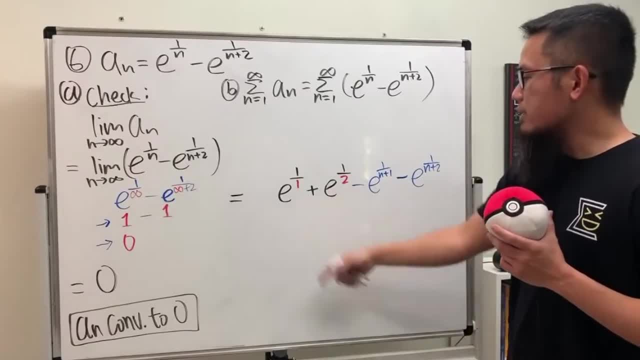 You just decrease this by 1.. So 2 turns in the front and 2 turns at the end, like that, And I'll show you guys why this is true right in a sec. So this is e to the 1 over n plus 1.. 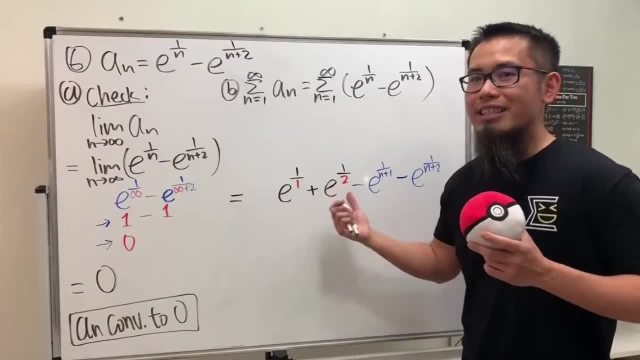 So this is e to the 1 over n plus 1.. So this is how you can write it down and in fact, this is what we call the n-partial sum formula, especially when you have a telescoping series, right? 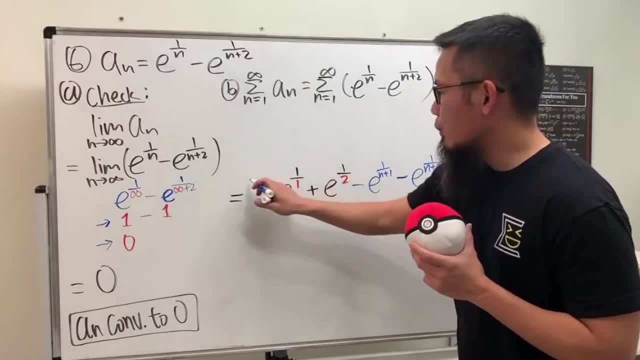 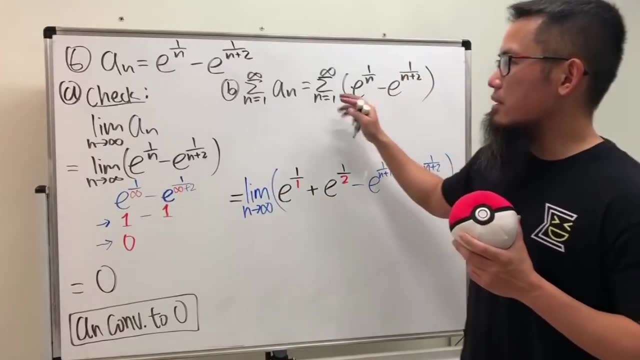 But this is not it yet. What we want to do is, after this, we are going to take the limit as n goes to infinity, Because remember this right here means that we are going to add up infinitely many terms right here, right. 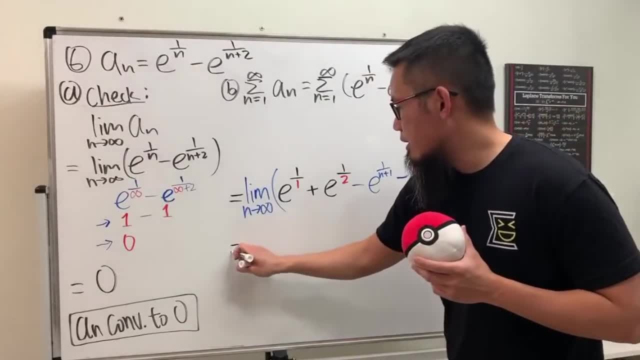 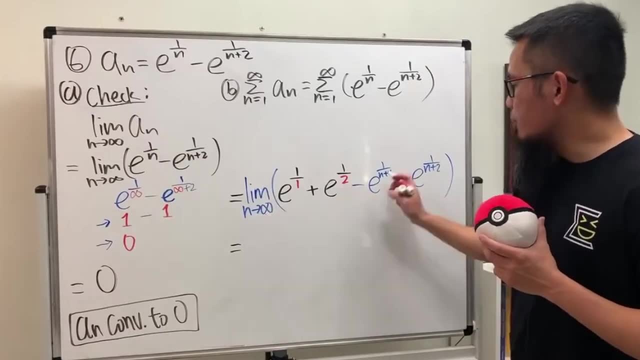 Alright, now check this out. This right here is just a number. This right here is just a number, But This right here, when n is infinity, you put it here. you get e to the 1 over infinity plus 1, which is e to the 0's power. 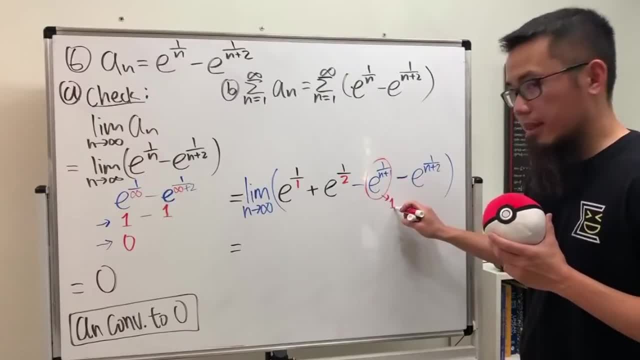 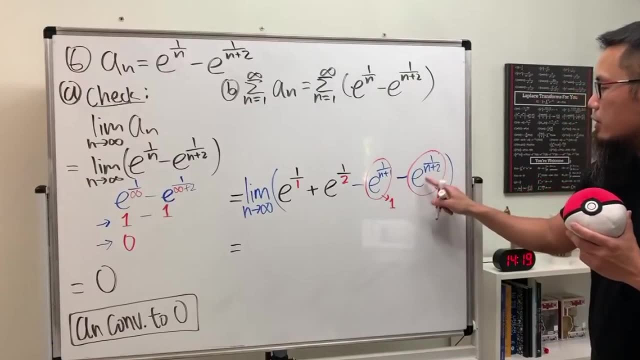 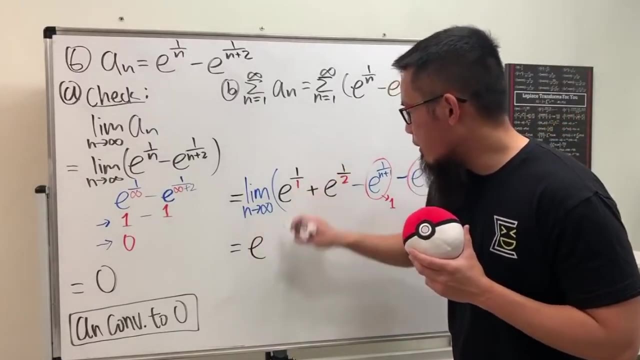 So, in fact, this guy will approach 1.. Likewise, this guy, when n approaches infinity, this is e to the 0, and we will get this being approaching 1.. So, all in all, this right here is actually e to the 1st plus e to the 1 over 2.. So all in all this right here is actually e to the 1st plus e to the 1 over 2.. So all in all this right here is actually e to the 1st plus e to the 1 over 2.. 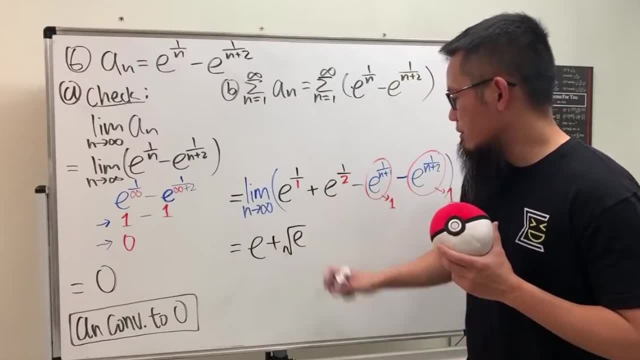 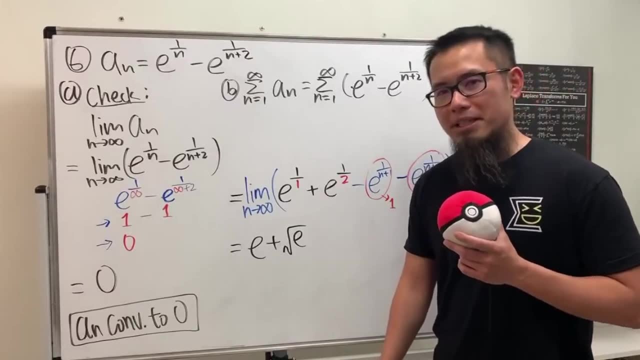 If you would like, you can write it as square root. be a little bit fancy. I would say: Minus 1, minus 1, do not put that down as minus 1 minus 1, please write it down as minus. 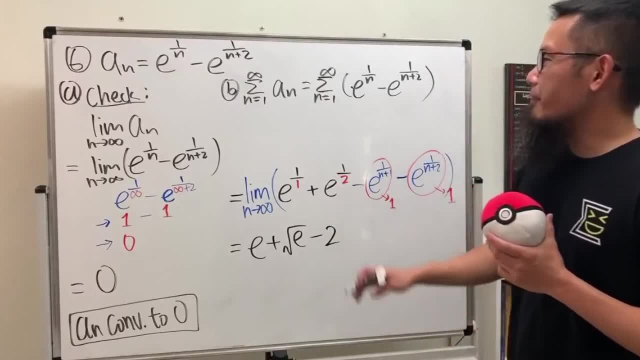 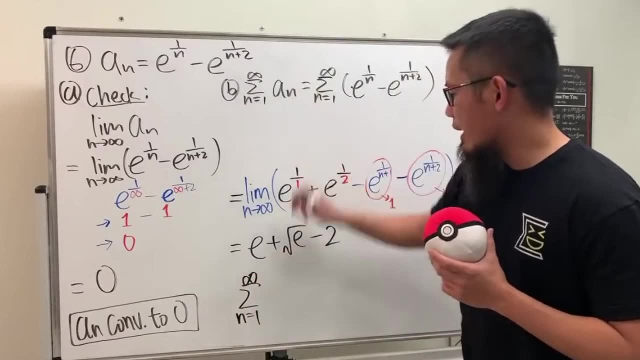 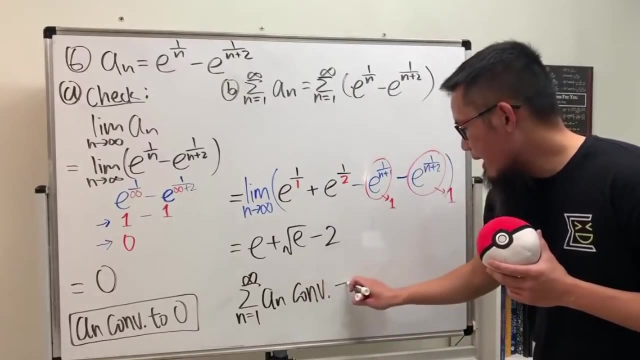 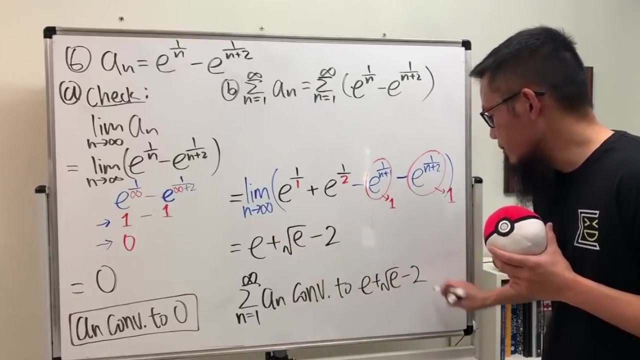 2.. Anyway, though this right here, we know that the series as n goes from 1 to infinity of our a n, which is that this right here converges, and in fact we know what it converges to. it converges to this e plus square root of e minus 2, by telescoping right. 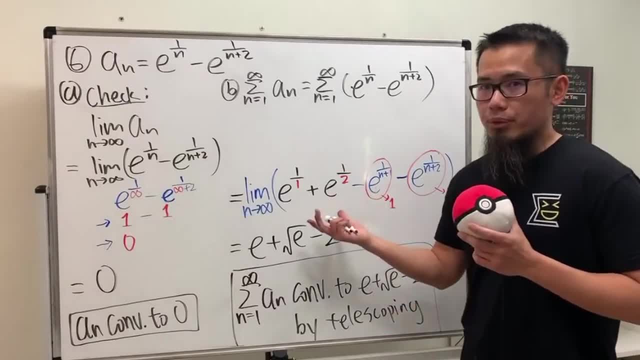 It's not really like telescoping test, but it's just a telescoping method to end up with that answer. so let me just write that down for that. Remember: earlier I told you guys write down some terms and then we'll just write down. 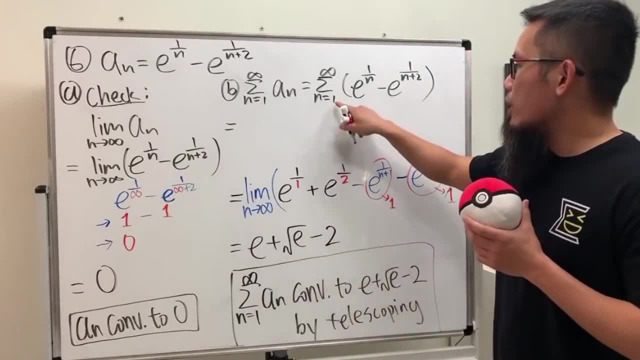 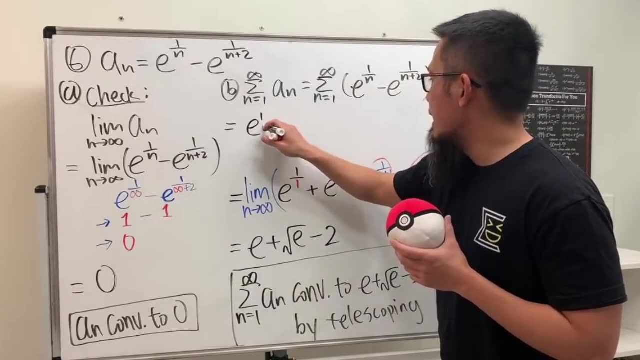 some terms and then we're just going to cancel things out, right? So the first deal is that we're going to put down 1 into the n's. that's the first term. So for the first parentheses we'll get e to the first minus e to the. put a 1 in here. 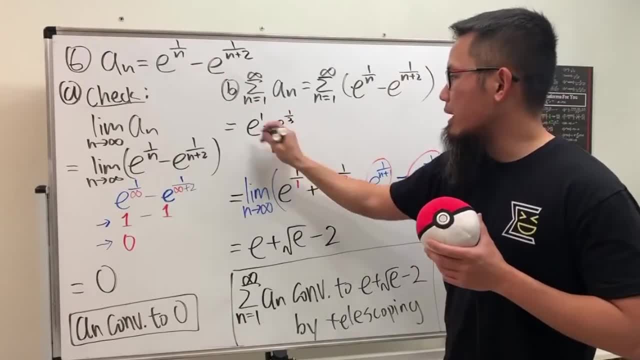 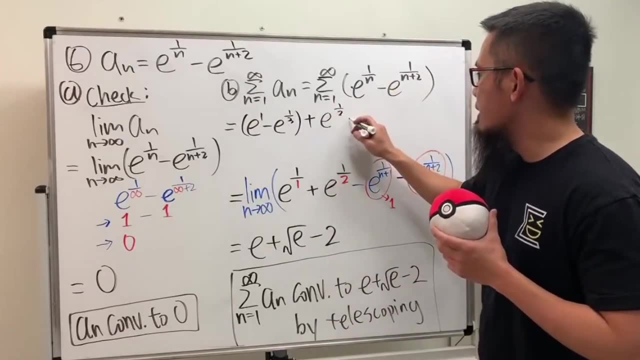 we get 1 over 3, so we have 1 over 3.. And keep in mind this: right here is the first term. Next, when n is 2, you put it here. put it here, so you have e to the 1 half and then. 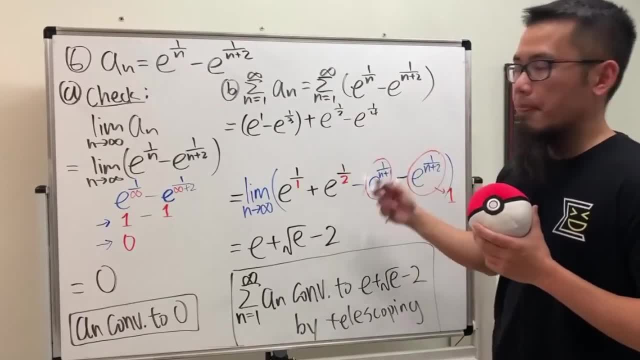 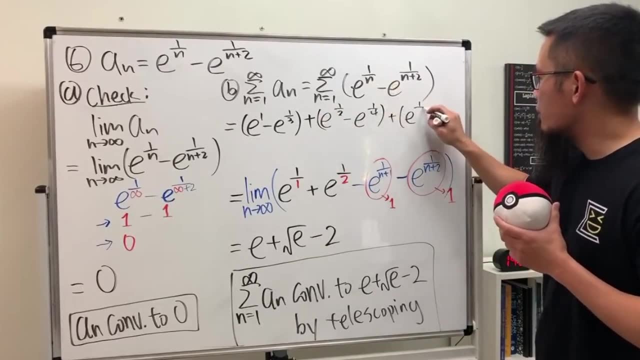 minus. put a 2 here, so you have e to the 1 over 4,. yep, So that's the second term, And then just write down the first term. Write down a few more, which is e to the 3, right 3 in here, which is 1 over 3, and. 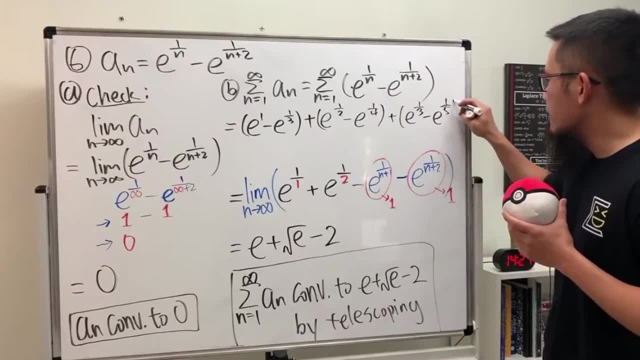 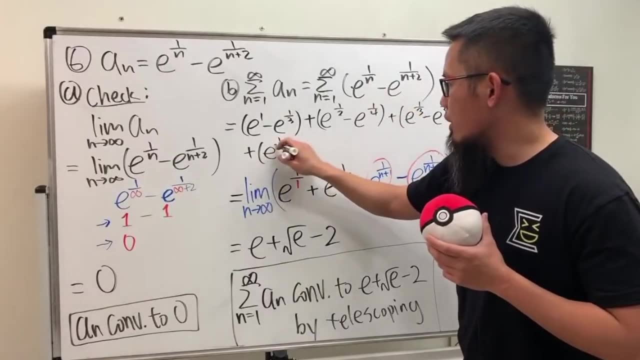 then minus e to the 1 over 5, and then plus. let's put down one more: when n is equal to 4, put it here, so you have e to the 1 over 4, and then minus e to the 1 over 6, and so: 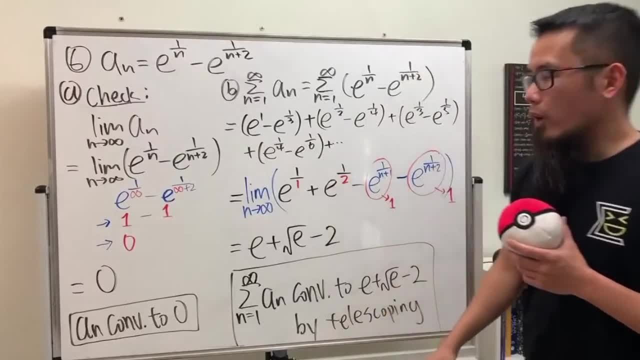 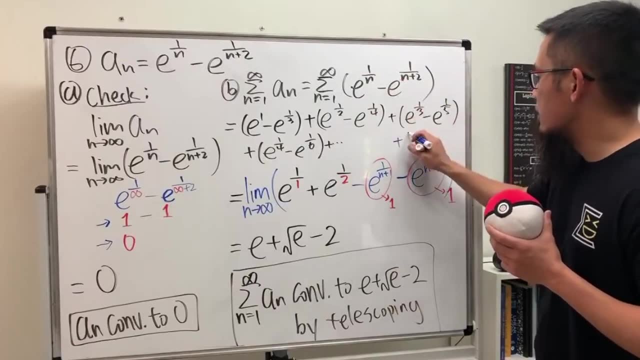 on, so on, so on. right, Well, we are going to write down the n's term as well. The n's term is going to be just this, namely e to the 1 over n minus, e to the 1 over n plus. 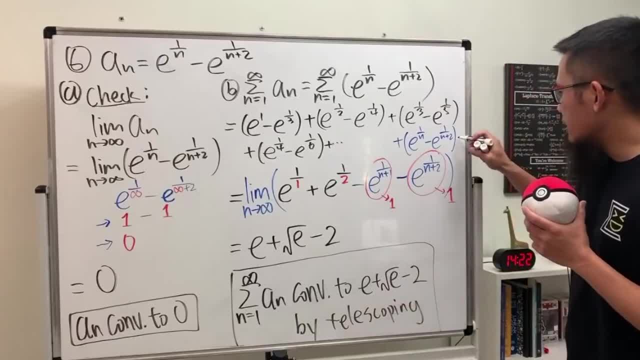 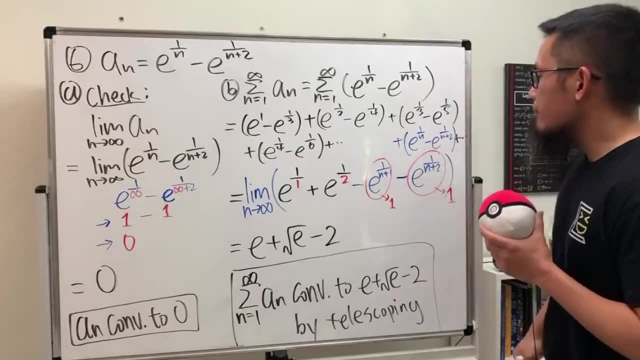 2. And after that, keep in mind there's a plus. dah, dah, dah, right. This is just. you stop at n. Well, because they are all by two terms, you should also write down the term beforehand. 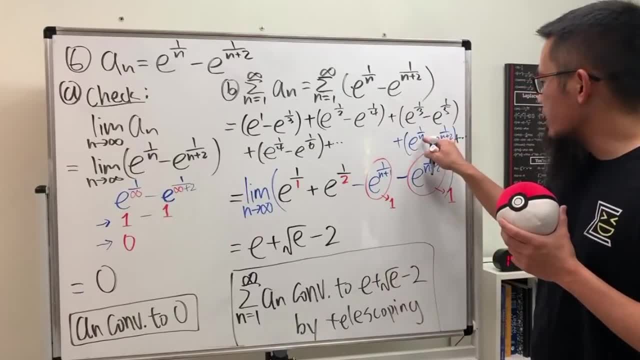 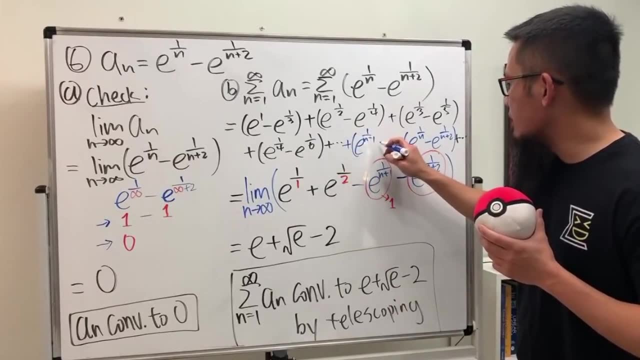 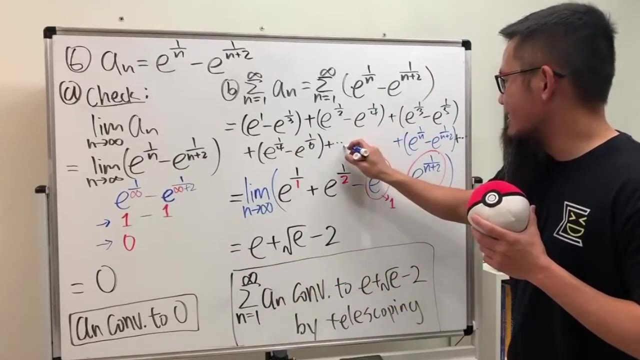 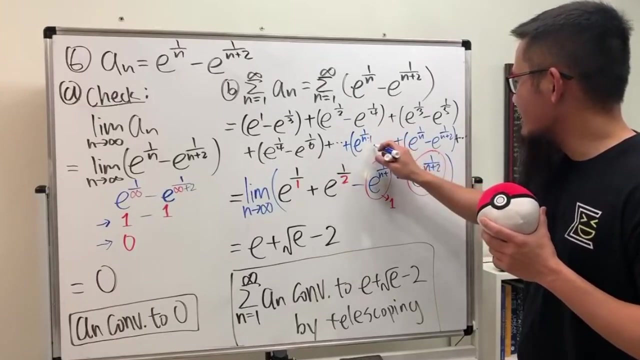 which is going to be. you substitute n minus 1 here and here, So we get e to the 1 over n minus 1 plus. sorry, let me just write it down better, because it's not clear at all: e to the 1 over n minus 1, and then minus e to the 1 over n plus 1.. 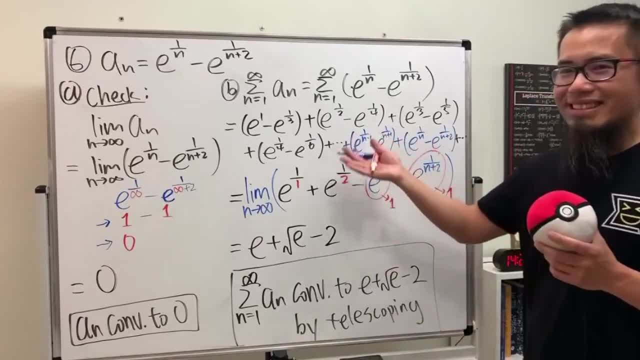 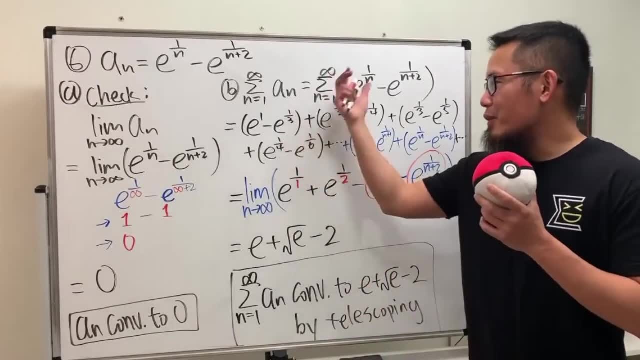 All right, we good so far. This is the write-out, and then I'm fitting everything right here. That's, I'm pretty happy about it. Now you see that when we write down everything, it's like this long right. 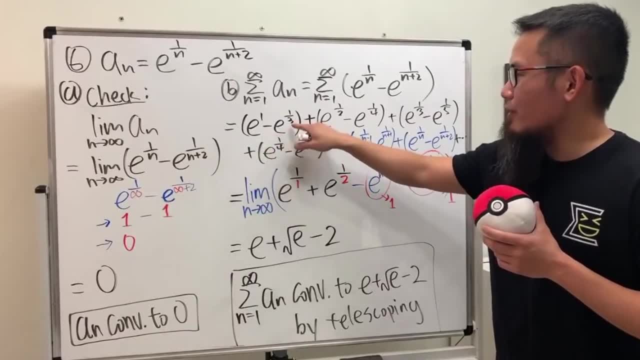 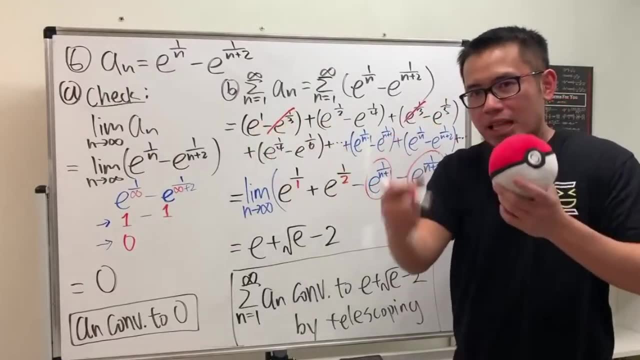 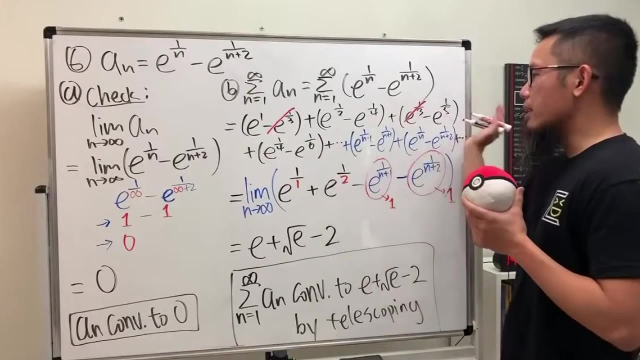 But the truth is, hey, we have negative e to the 1 over 3, but here we have positive e to the 1 over 3.. So we can cancel this out and that. So it start to clap right. This stays, and you see this right here. e to the 1 half also stay, because you don't. 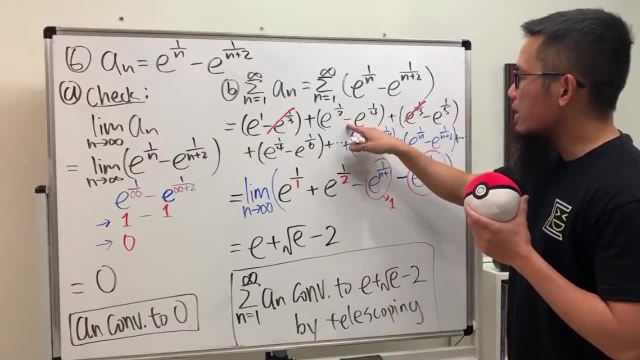 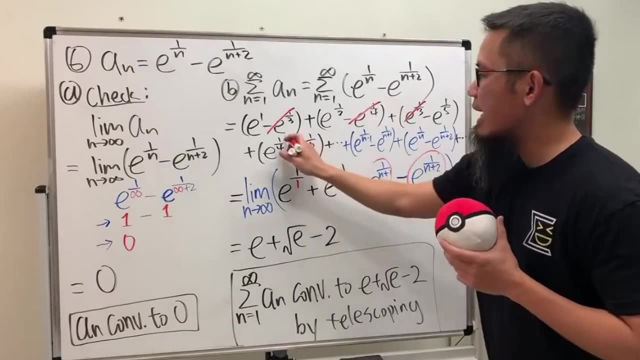 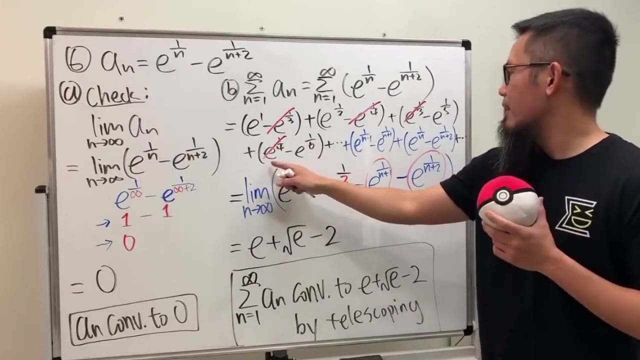 see another e to the 1 half. But if you look at negative, e to the 1 over 4.. Guess what We have this e to the 1 over 4.. So this and that get canceled. And now you see, in this parentheses this guy get canceled first. keep that in mind. 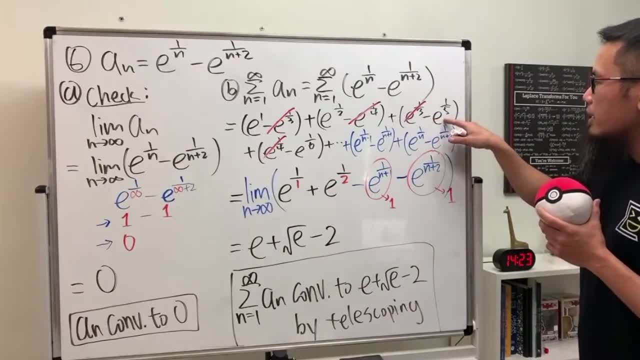 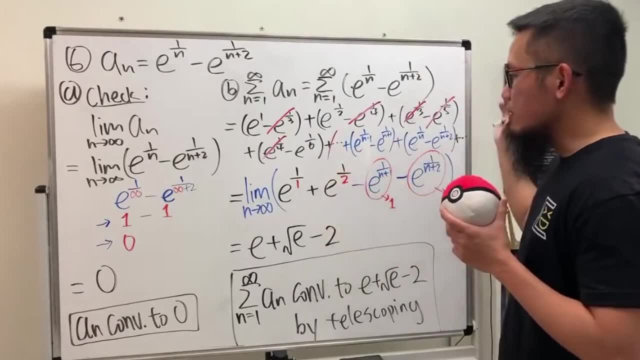 Anyway, though, here you can see that negative e to the 1 over 5, this right here will cancel out with this term. I just didn't write it down And then so on, so on, so on. this guy is going to cancel out with some guy right here. 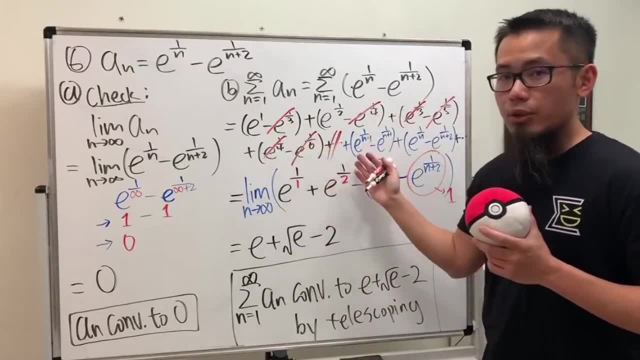 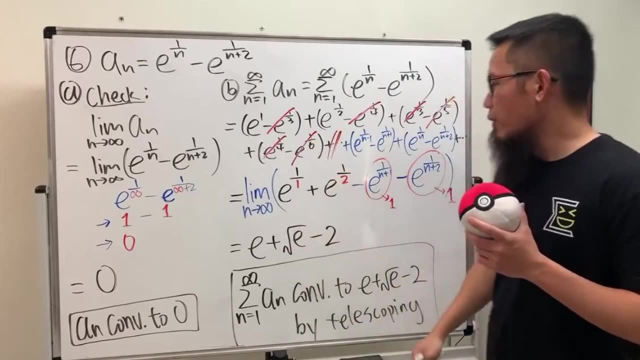 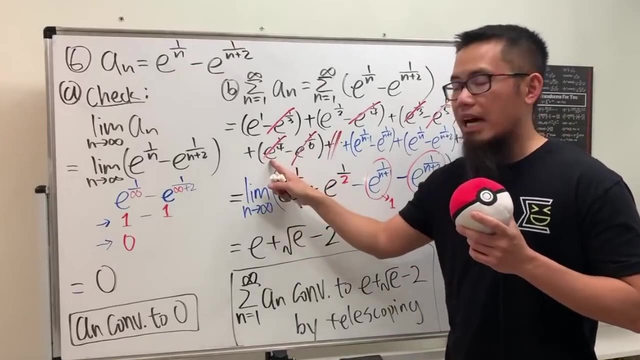 So With this they are going to get canceled out. Now notice that we have this and that survived. that's what we did, But don't forget that you also have to pay attention to the end term. right here And, as I said earlier in the parentheses, right here this guy get canceled out first. 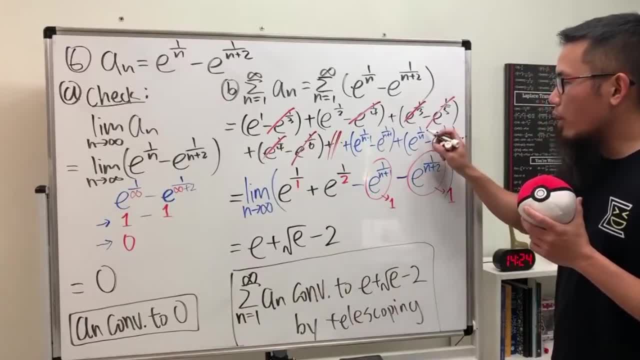 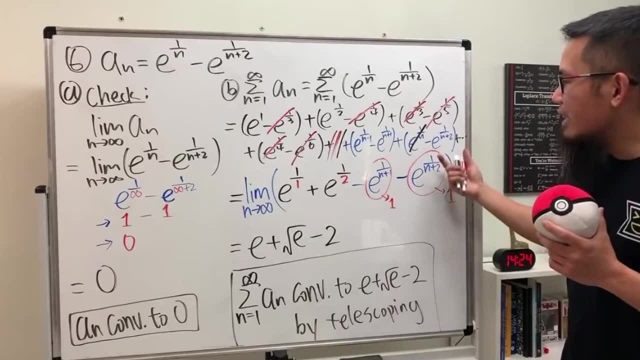 So, if you look at this well, here we have e to the 1 over n. this is going to get canceled out with some guy in the front right here, isn't it? Yes, And if you go to the previous term, this guy is going to get canceled out with some. 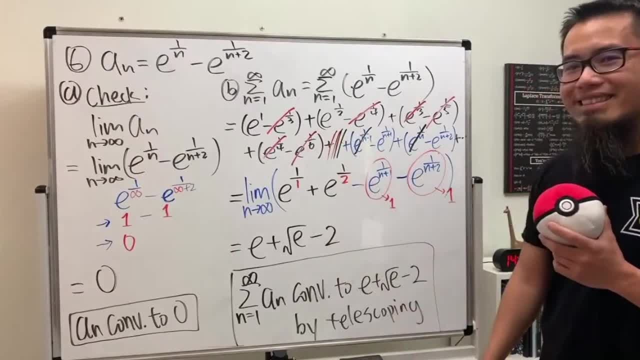 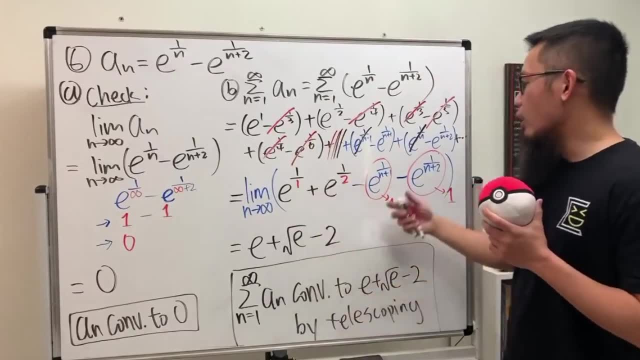 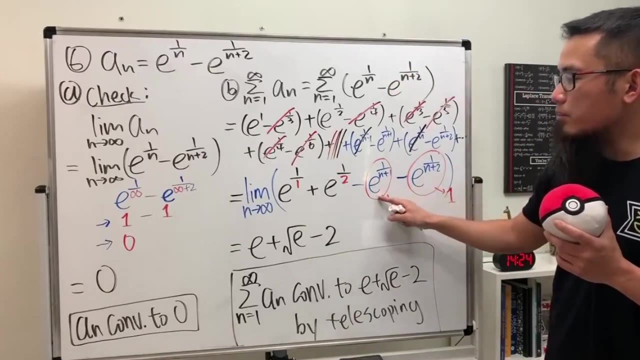 guy beforehand, isn't it? Yes, That's why, when they are off by 2, just write down the first two terms right here by doing what I told you, and then also write down the last two terms like that. Just put this down right here and then go to its previous term. that's it. 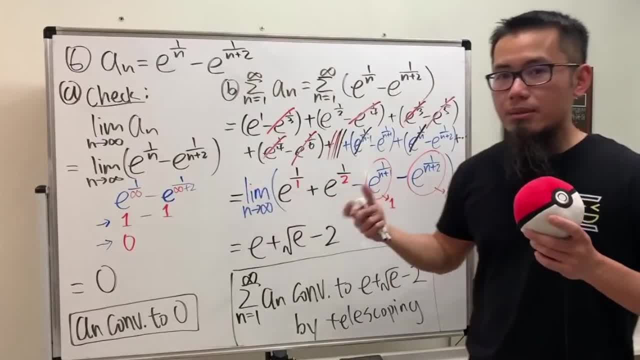 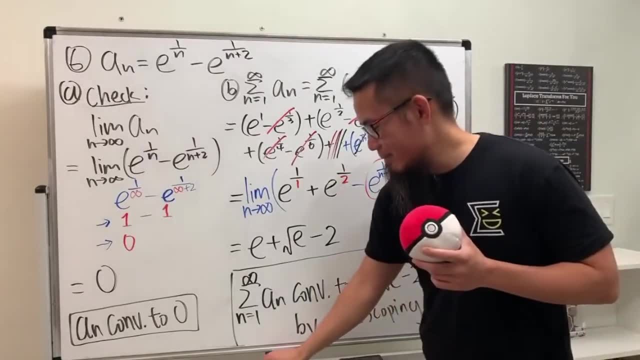 You can go from here to here in my class, but I'm not sure about your teacher. Maybe your teacher wants to see the cancellations, then in that case do that. But you can also remember the shortcut. is this all right? 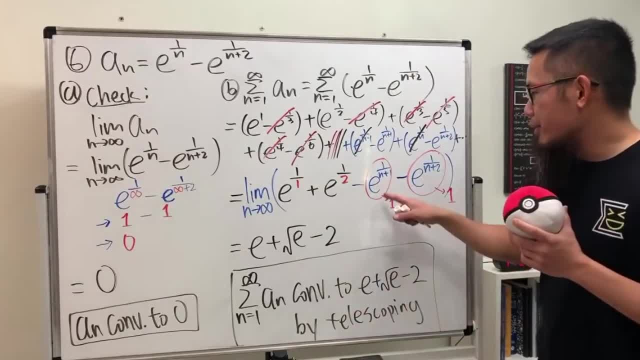 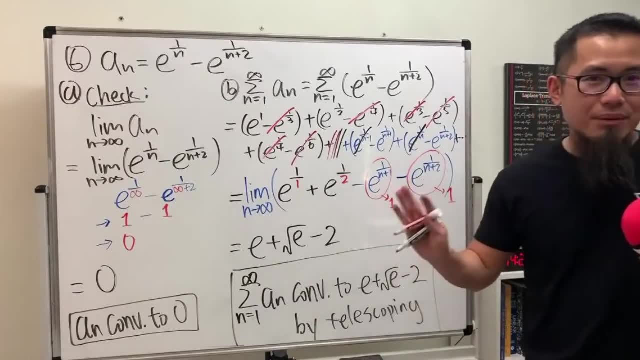 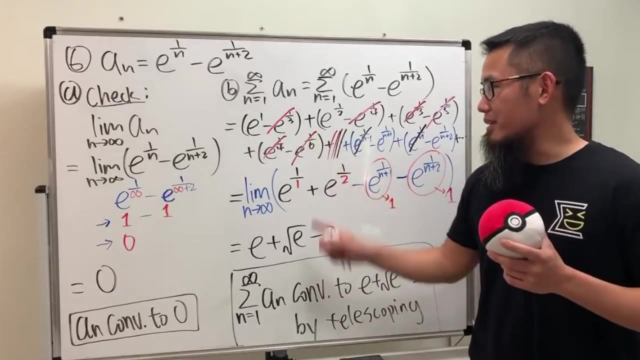 So hopefully this is okay. One thing, though: you will have to check the limit. right here. A lot of students. they tend to forget about the limits for this because they think it's always equal to zero, but that's not true Sometimes. if this right here doesn't exist, then you don't have a limit for the series. 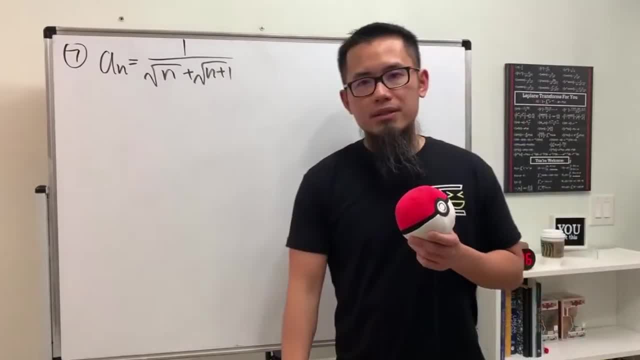 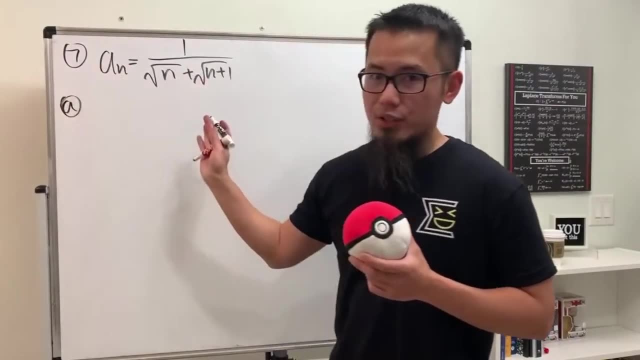 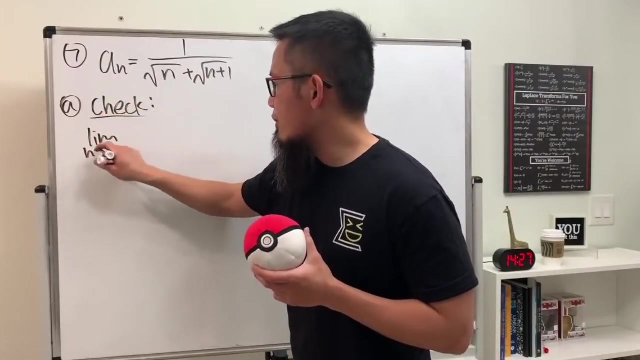 so that's bad. This right here is the limit for the series. Okay, So here it's not so bad. you'll see First check if a n converges or not. So by that we will check the limit, as n goes to infinity and a n which is just the limit. 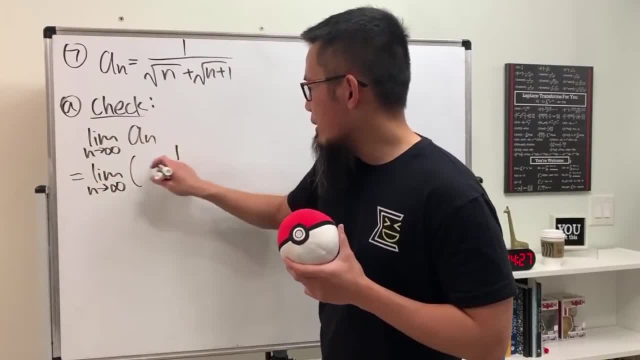 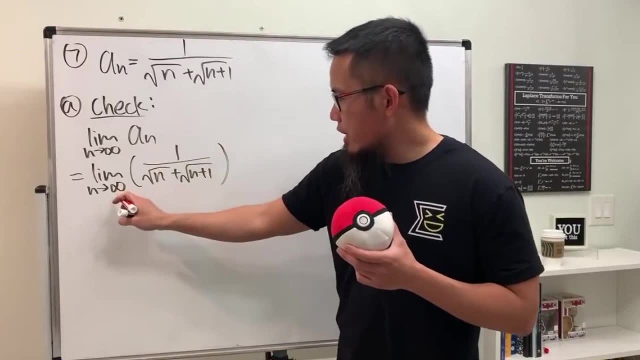 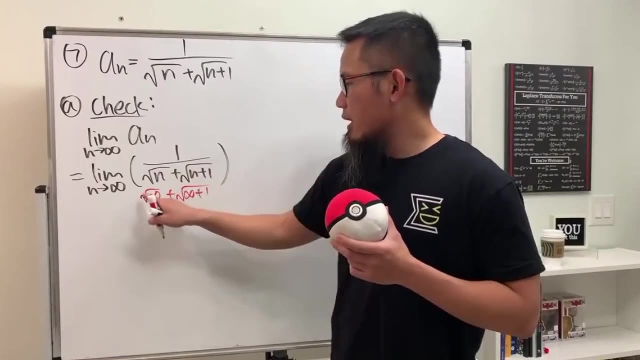 as n goes to infinity of that which is 1 over square root of n plus square root of n plus 1.. So here we can actually just put infinity to. here you get square root of infinity plus the square root of infinity plus 1.. 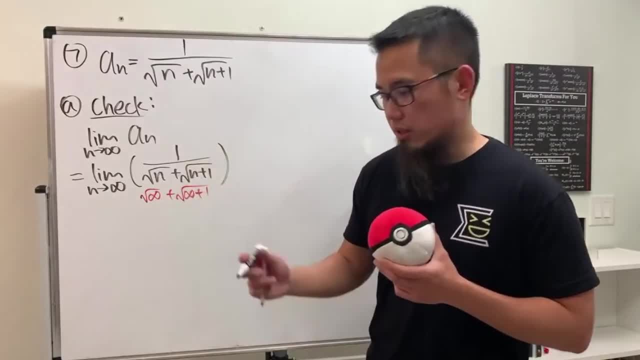 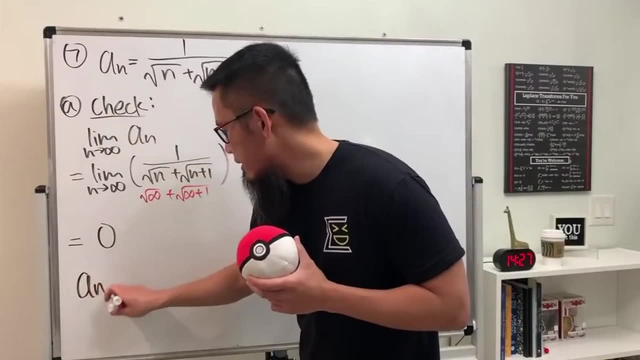 On the bottom it's just going to be infinity. 1 over infinity, you get zero. So all this is just equal to zero. Therefore, we can say: a n converges, and we know that it converges to the number zero. 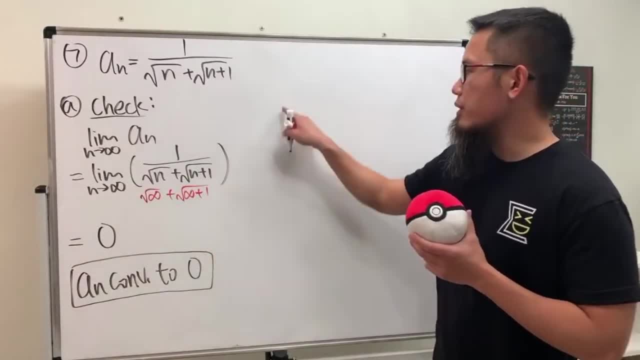 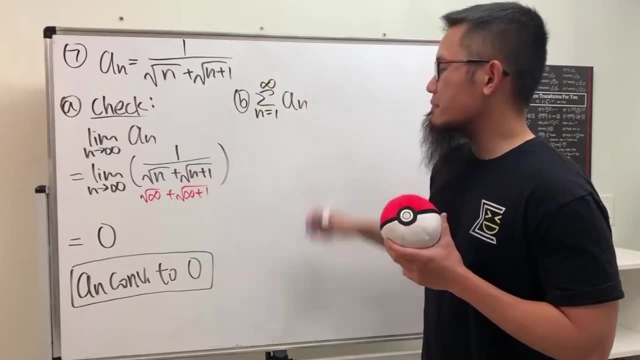 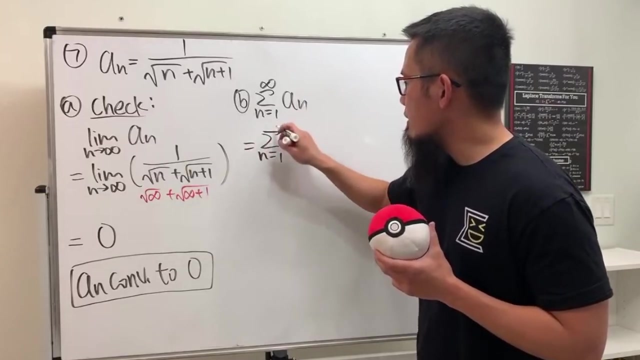 Done. This does not do us any good in terms of finding the convergence of the series as n goes from 1 to infinity of a n. We have to do more work. Yeah, Anyway, though, to check this, we are just checking the series as n goes from 1 to infinity. 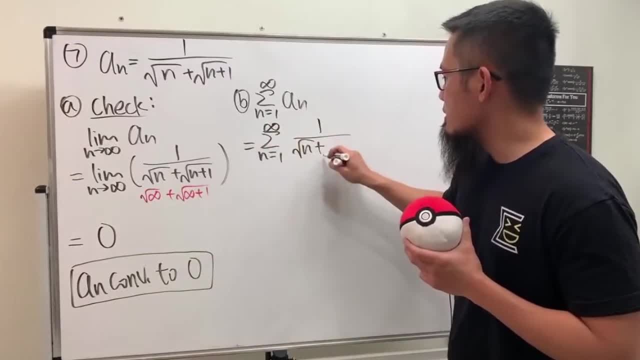 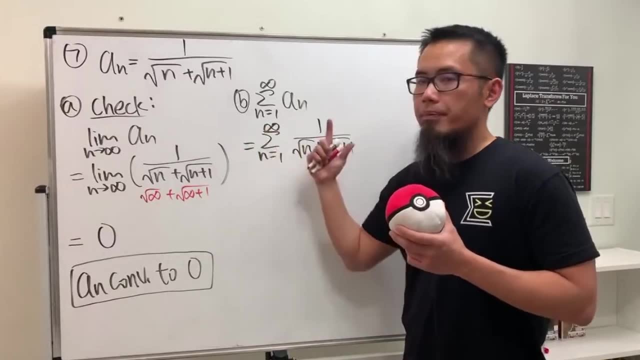 of 1 over square root of n plus square root of n plus 1.. Right Now, imagine you see this later on. Yes, You can use what we call the Compression Test To finish this Right, That's totally okay. 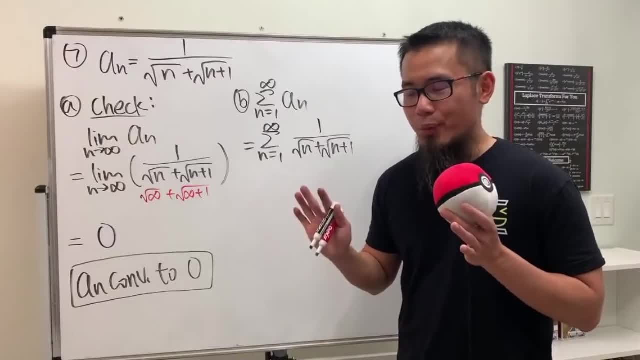 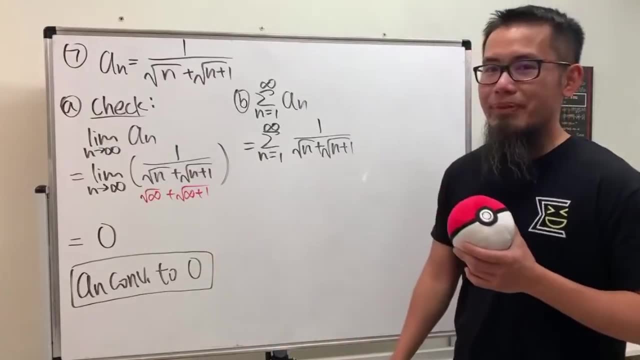 But again, this is an introduction video, so we're not there yet. Huh, That gives us zero, so we have to do more work for this. This is what we can do. We can do the conjugate. Have a look. 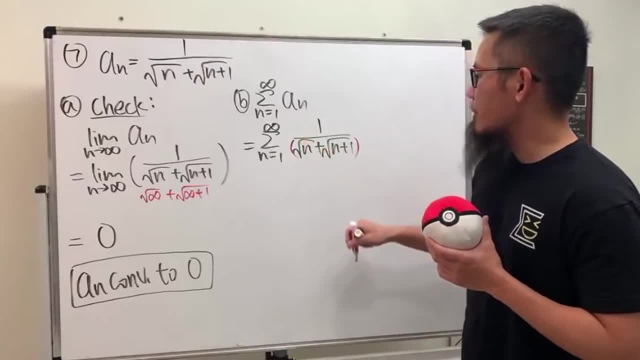 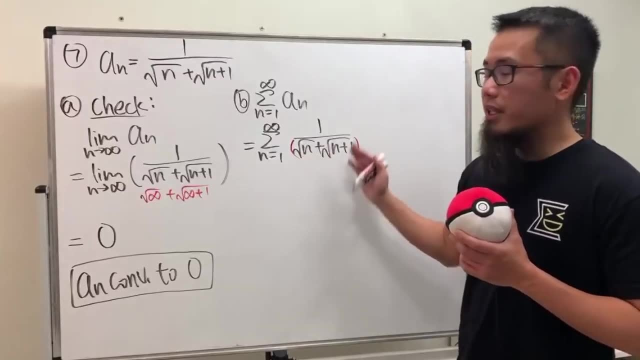 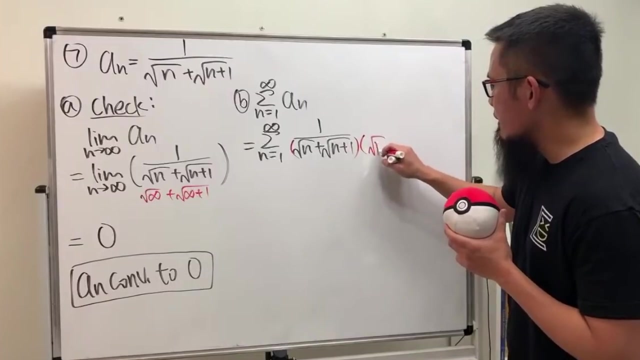 Right here I'm going to multiply the top and bottom by the conjugate of this and because- And the reason for that is because we see we have the square root in the rational expression- That's usually a good idea to go. Therefore, let me multiply the top and bottom by square root of n minus square root of n. 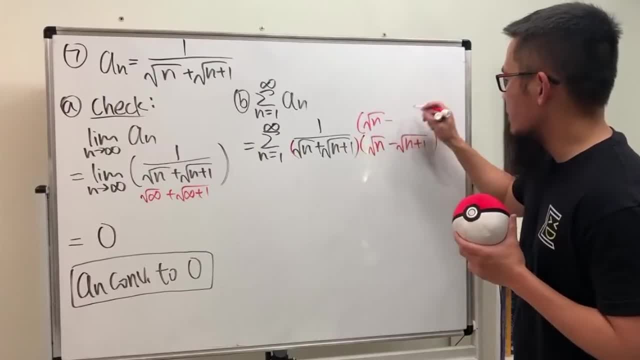 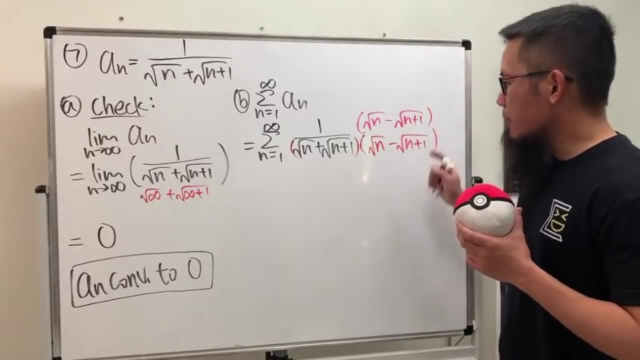 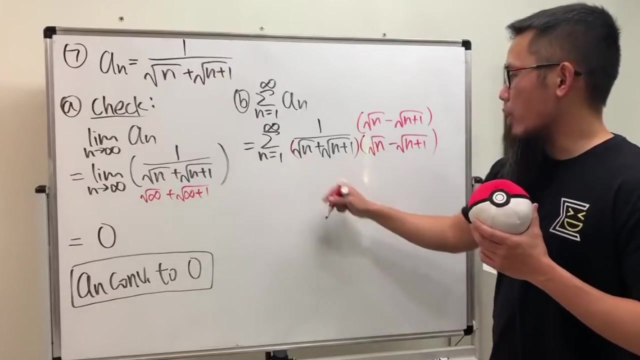 plus 1.. And then let's do the same thing on the top as well. Now check this out: When we multiply out the bottom, this right here becomes what This is just going to be, this thing squared, which is n. 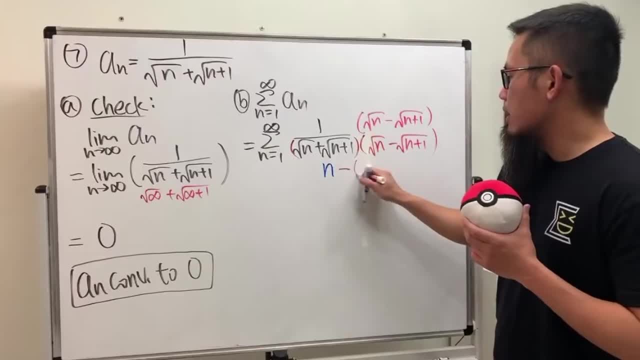 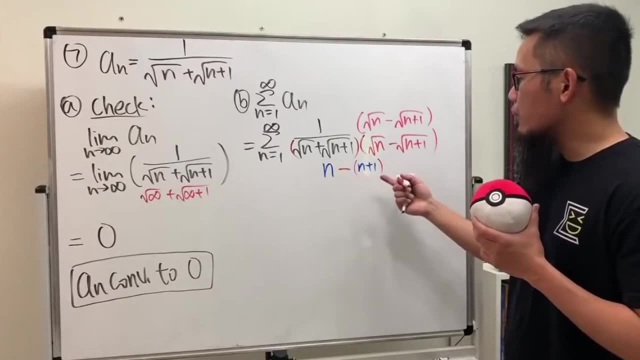 And then minus What This, This thing squared, which is n plus 1.. Right, And n minus n is just equal to zero and then minus 1.. So technically we have a minus 1 right here, All right. 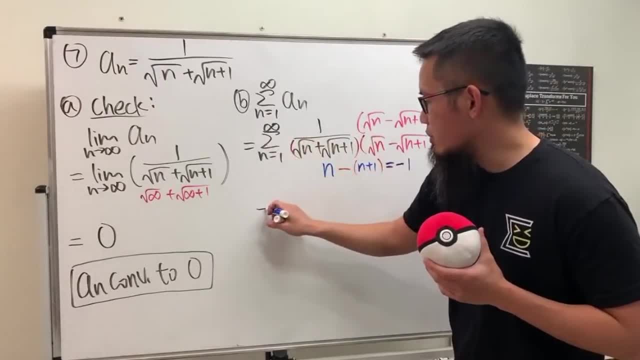 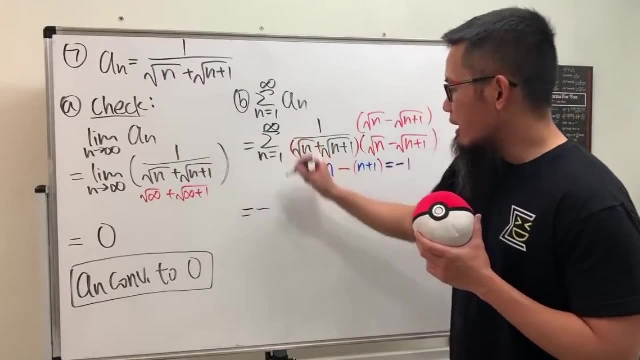 So here we have negative 1.. Let me put the negative 1 in the front of the summation, So I just want to make this slightly more clear for you guys. Right, Negative 1 in the front already. And then we have the series as n goes from 1 to infinity. 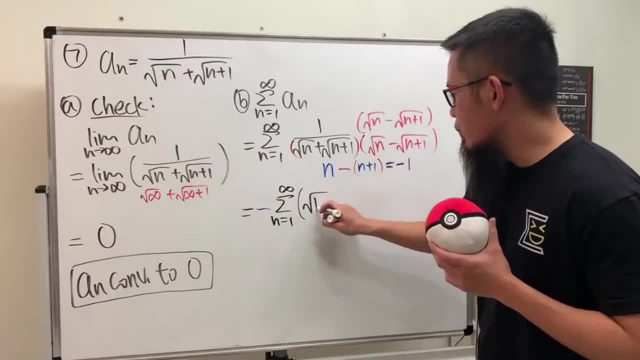 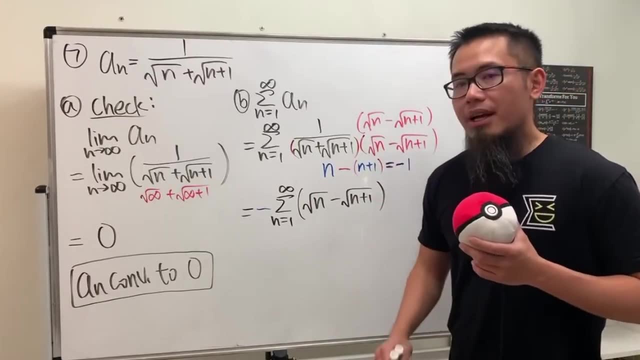 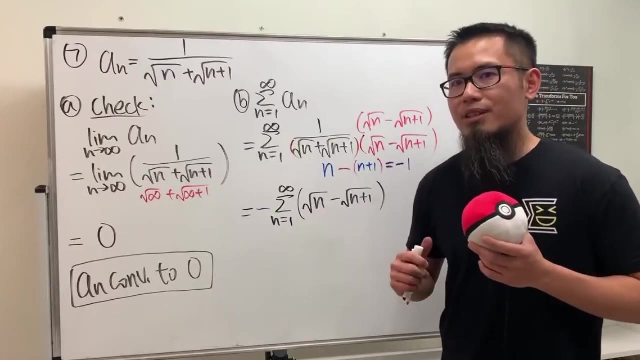 And we have just this, Namely n in the square root minus square root of n plus 1.. All right, This is the reason why I did it this way, Because you can see that, yes, this right here is a telescoping series. 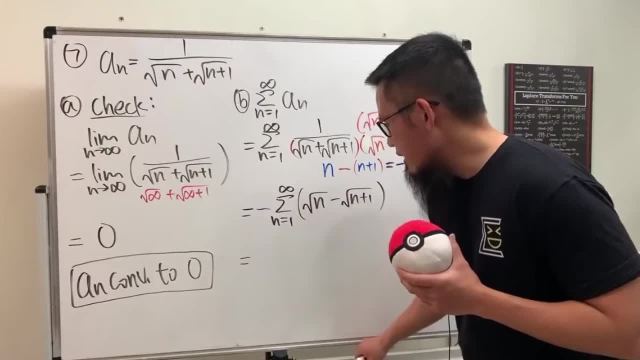 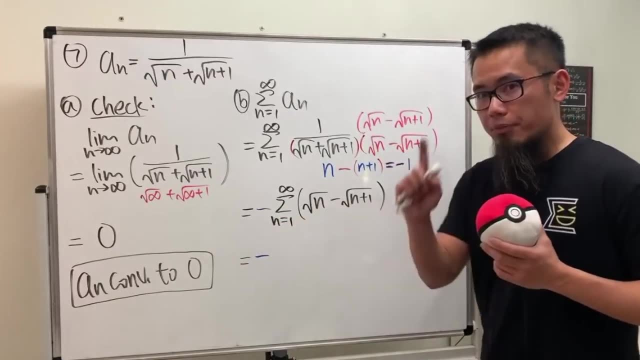 But check this out though This right here, we still have the negative all the way in the front, And that's do what we did earlier, Right This time: this, and that they are just off by 1.. So I'm just going to put the 1 in here one time. 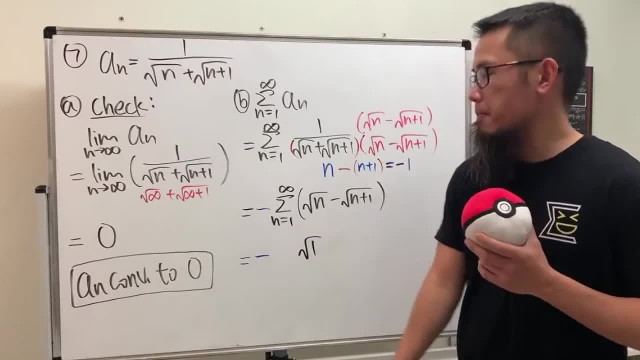 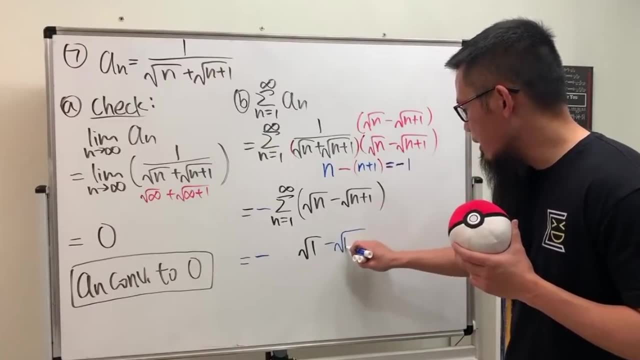 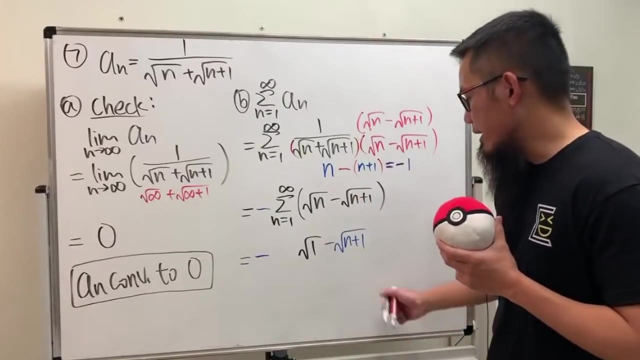 So we have square root of 1. And we are done. And then we are going to look at this and then put that down, which is negative square root of n plus 1.. Yeah, So that's what we did earlier, And don't forget that we will have to take the limit. 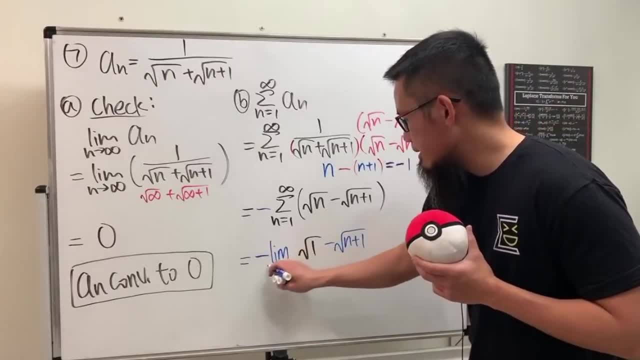 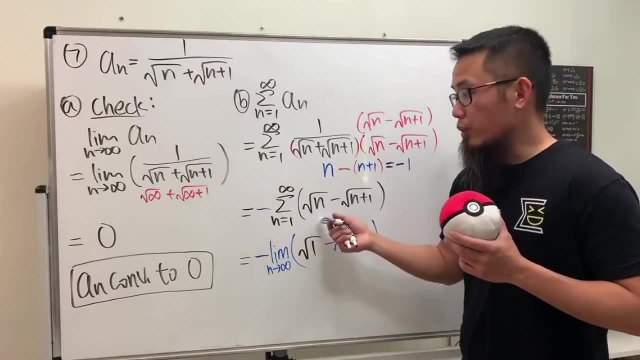 And we will have to take the limit. And we will have to take the limit As n goes to infinity. So again, we change this to limit because we are doing the telescoping thing right. So that's why this becomes a limit. 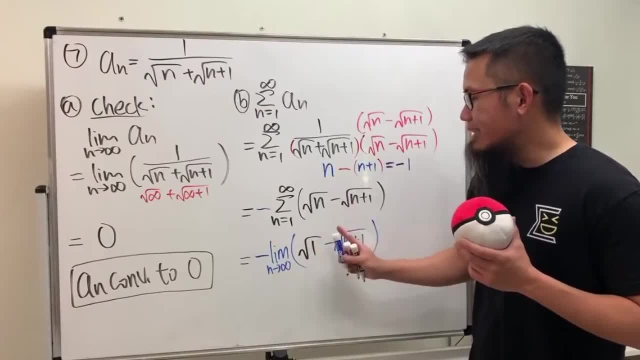 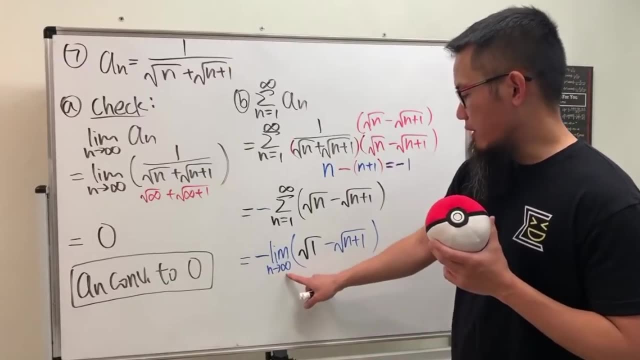 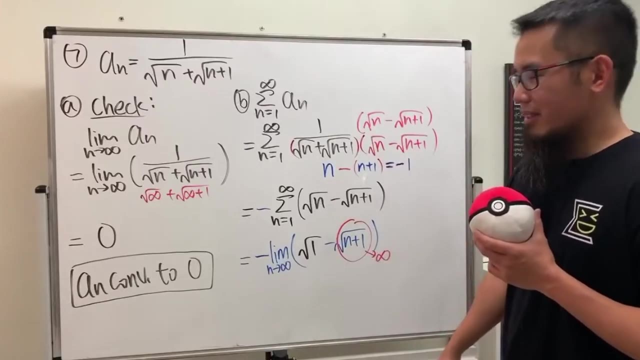 Because this right here is technically the nth partial sum for this guy already. Well, in this case you will see, as n goes to infinity, this guy goes to where Infinity. So have a look. So technically, if you would like to just do some computation, this is going to be negative. 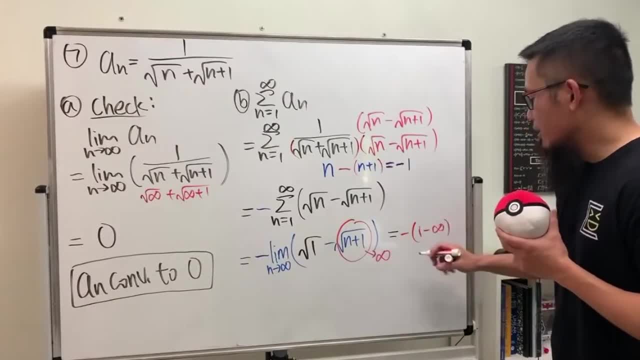 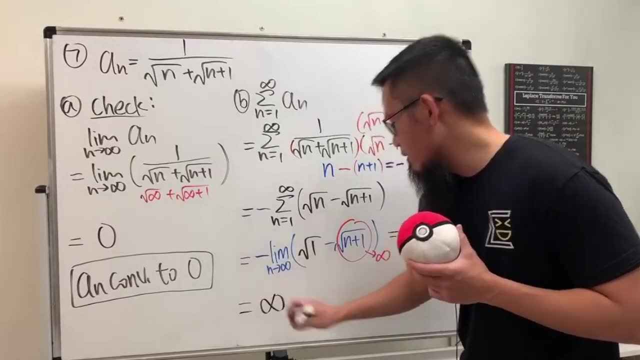 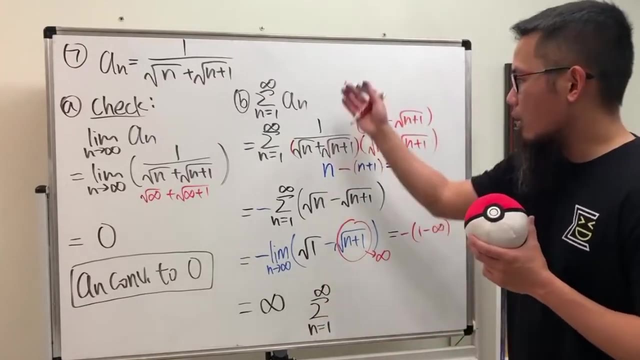 And then we have 1 minus infinity. So, all in all, this right here is actually just going to be infinity right. This right here is actually going to be infinity. So therefore, we know that this series as n goes from 1 to infinity of a n, this right. 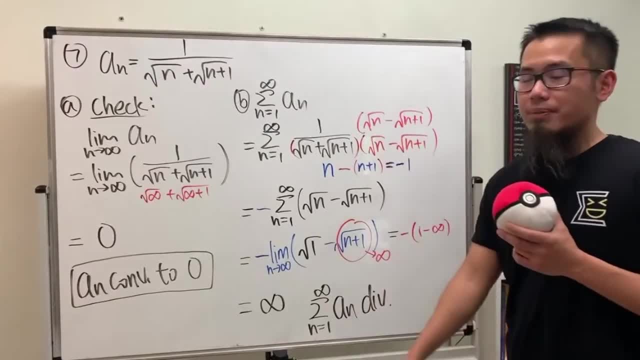 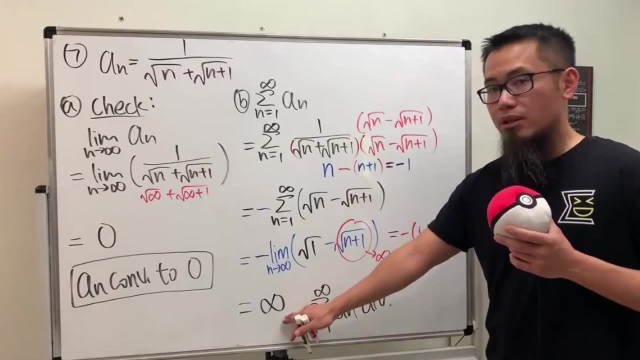 here diverges And this right here diverges Right, Right. And the reason is because we have shown that this right here is going to give you positive infinity, So it diverges to infinity. But you can also quote the reason. You can just say by the telescoping thing: 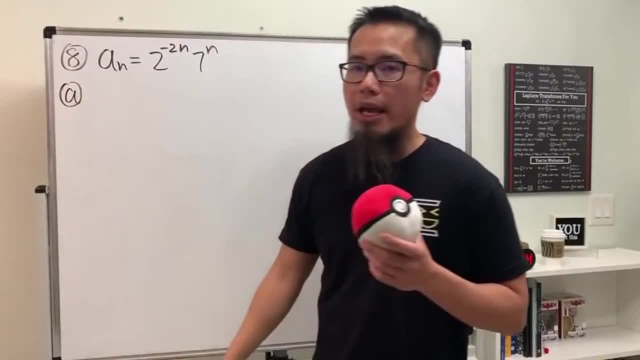 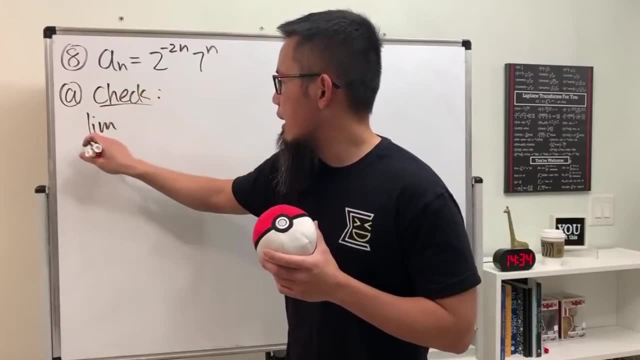 There we go. Nice Part one, Sorry, part a. Does a? n converge Again? that means we are just going to check the limit as n goes to infinity of a n. So this means the limit as n goes to infinity of a n. 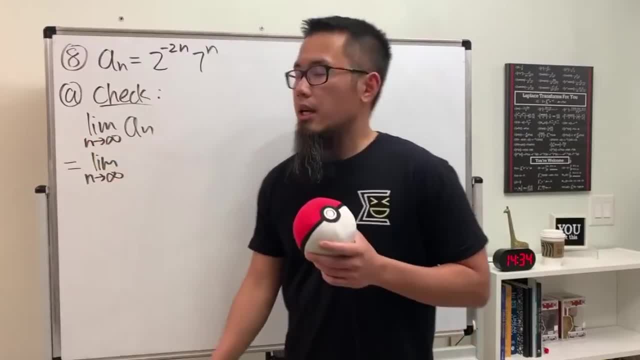 So this means the limit, as n goes to infinity of a n. So this means the limit, as n goes to infinity of a n. So we'll take 2 to the negative 2 n. So this is f of infinity a n is that? 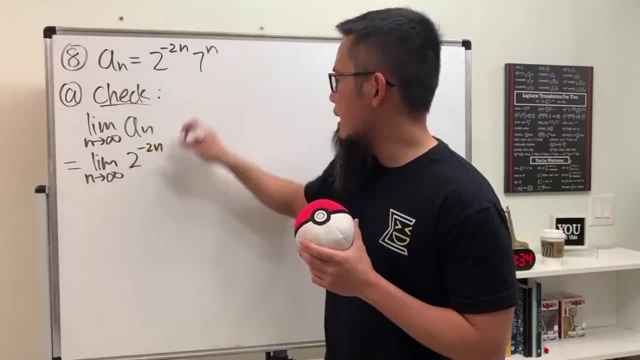 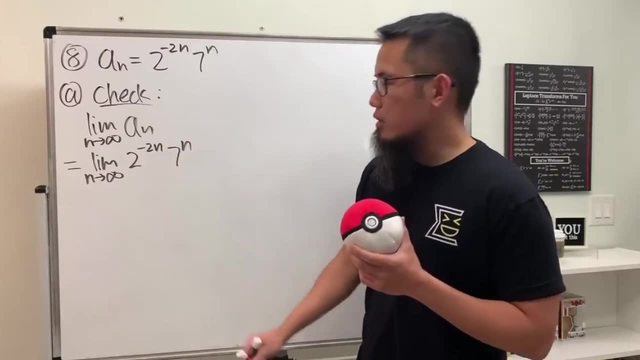 So let's write that down: 2 to the negative, 2 n and then 7n. Notice that both of them have n, so we can put the n's power on the very outside. So if you would like, you can look at this right. the limit as n goes to infinity. 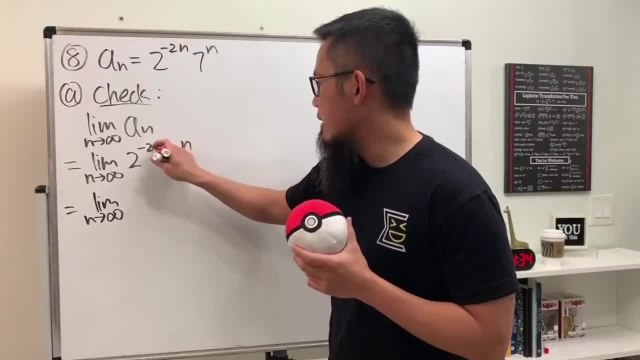 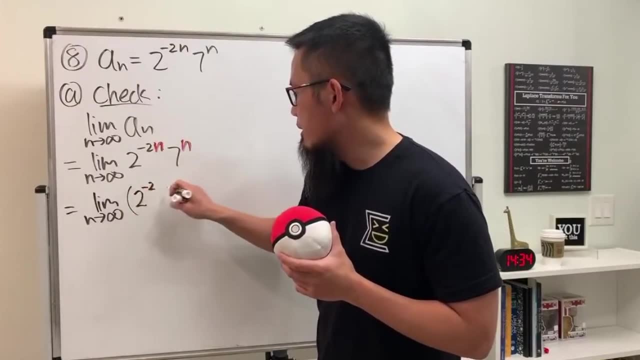 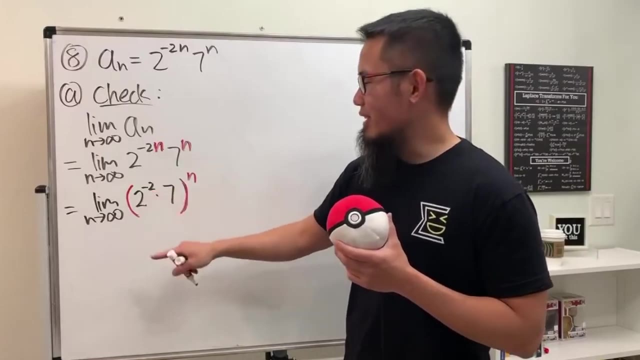 Again this n and that n. we can just put it on the outside. So here we are looking at 2 to the negative, 2 times a n, 7, and then, raised to the nth power, 2 to the negative 2 is equal to 1 over 4, so you can just write this down as 7 over 4.. 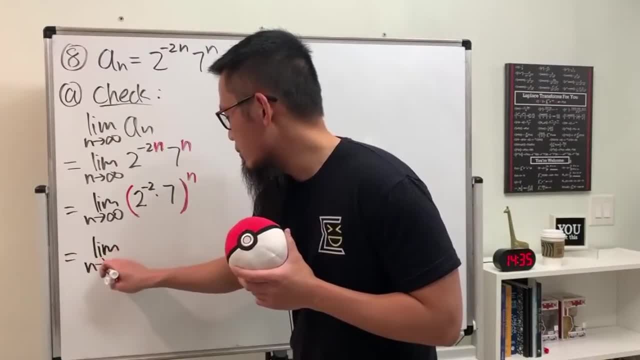 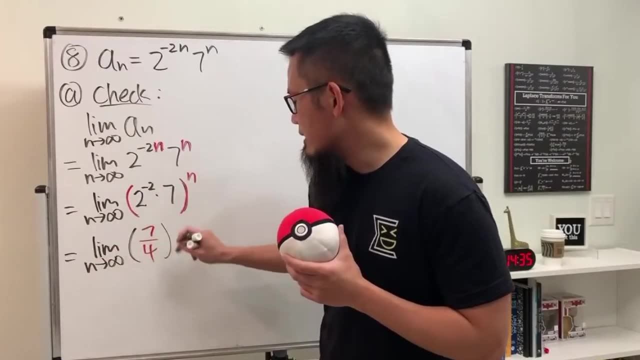 So this right here is really just the limit, as n goes to infinity, and then we will have 7 over 4 raised to the nth power. This right here is infinity right Because this number is bigger than 1 raised to the nth power. 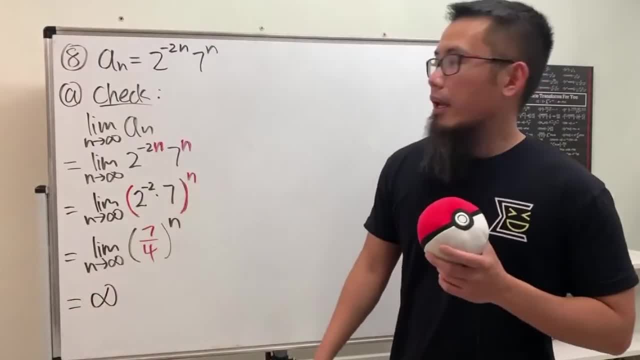 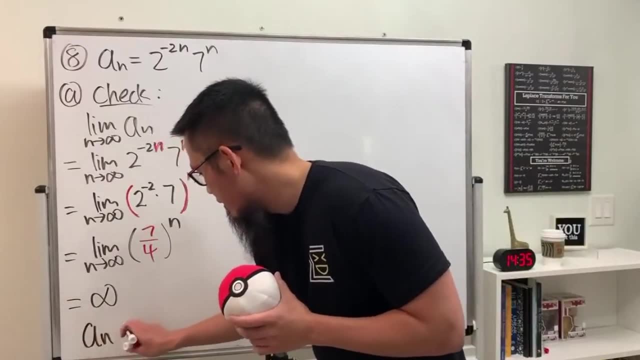 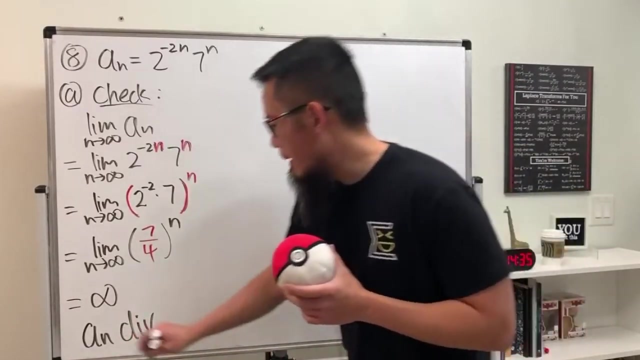 so this right here gives you infinity. And do not say a n converges to infinity, no, You just say a n diverges. You can say a n diverges to infinity, that's fine, but just leave it like this, Maybe even better: a n diverges, that's all. 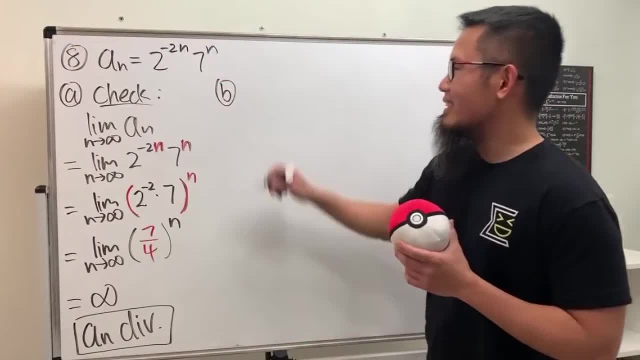 Okay, so for part b, check the series as n goes from 1 to infinity of a n. Okay, so for part b, check the series as n goes from 1 to infinity of a n. Thus, this is infinity. Thus, this is infinity. 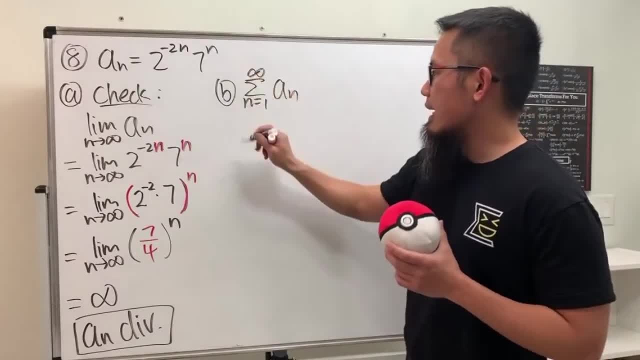 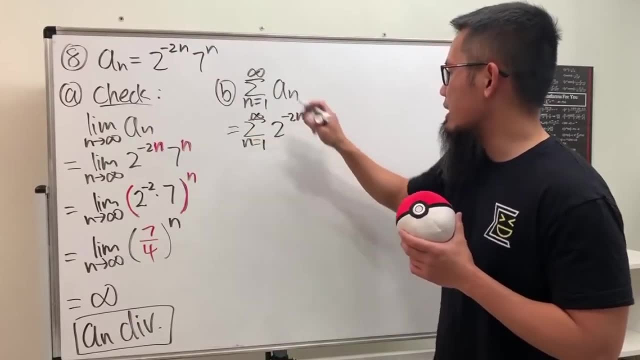 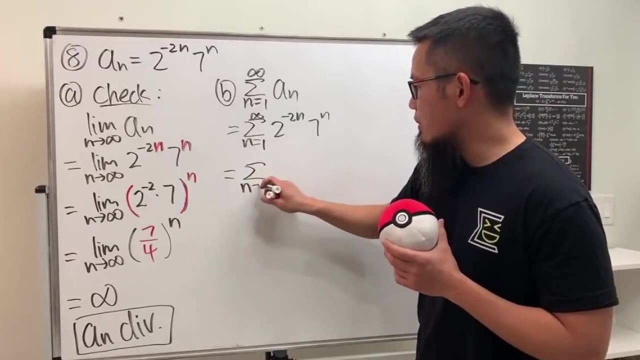 Thus this is converging, right. So a n is that? so let's write that down. We are checking the series as n goes from 1 to infinity, and let me just write it down as how it has over there, And you can write this down like that, which is the series as n goes from 1 to infinity. 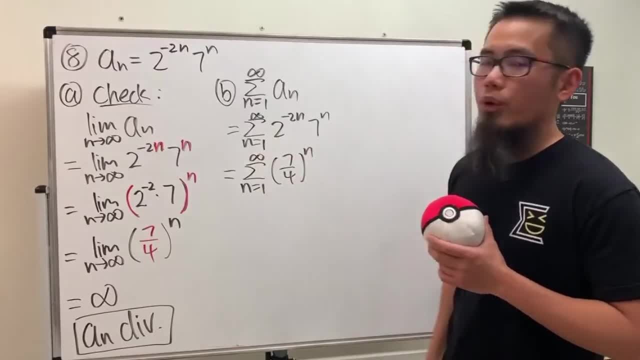 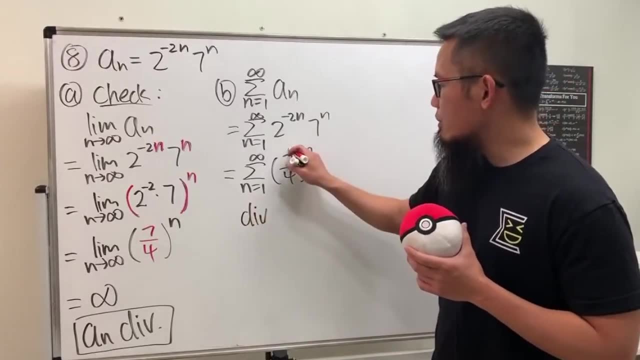 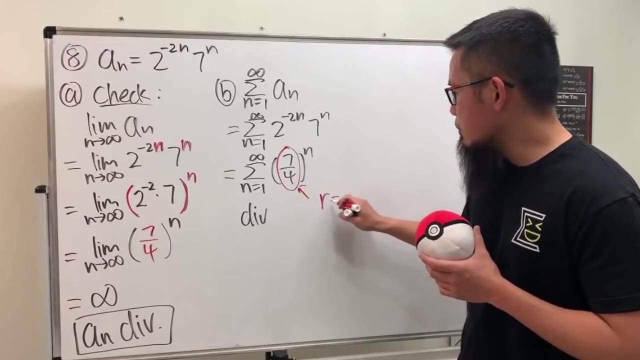 and then we have 7 over 4 raised to the nth power, And by this you can say it diverges. Why? Because you notice that This right here is a geometric series And to do so you can just say: r is equal to 7 over 4.. 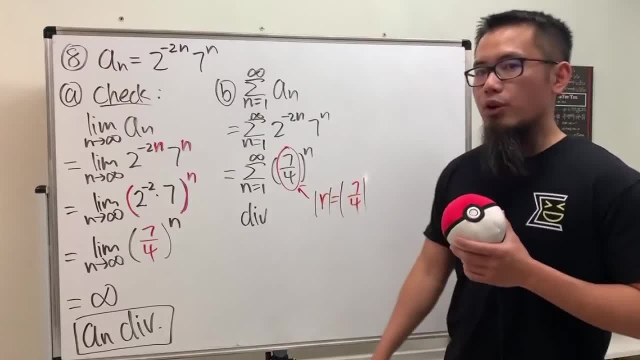 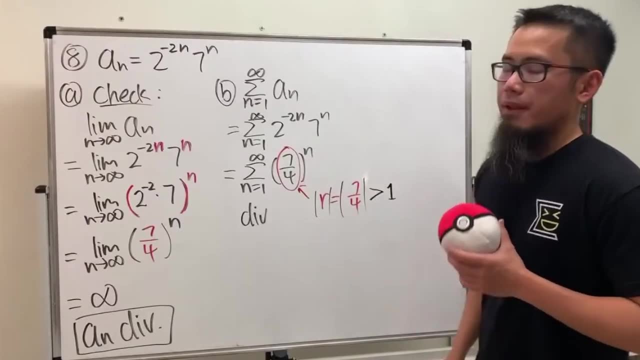 If you look at the absolute value of r, this is the absolute value of 7 over 4.. But don't just tell me that. You have to tell me that this is greater than 1.. And I insist, you guys to write this down. 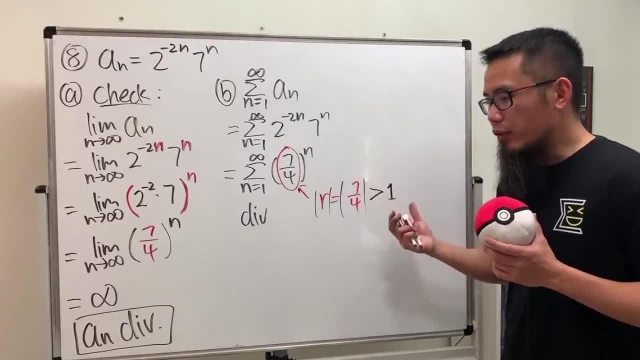 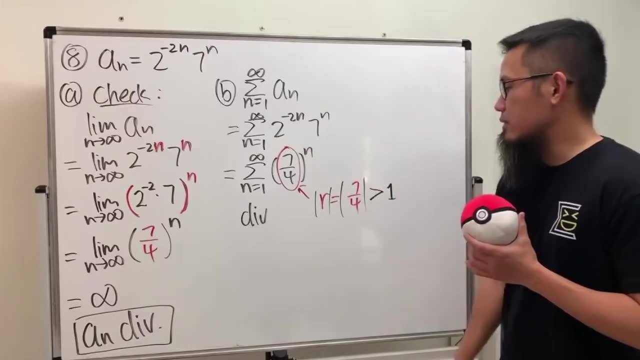 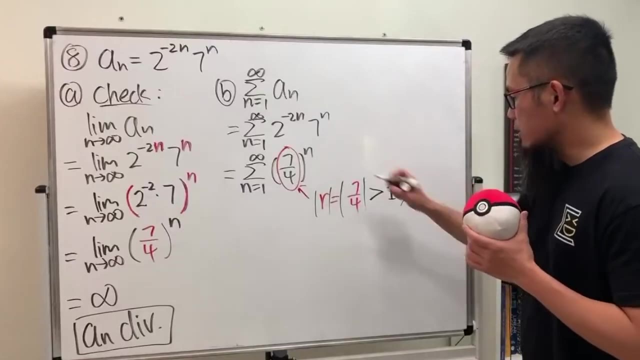 because later on we'll be using different numbers in different tests to tell us if the series converges or not. So get used to this kind of things. So, because this right here is greater than 1, therefore the series diverges. 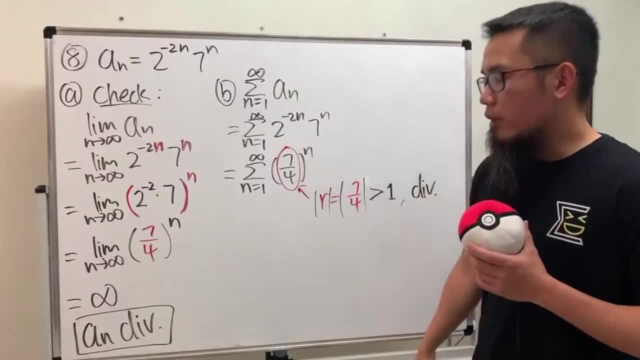 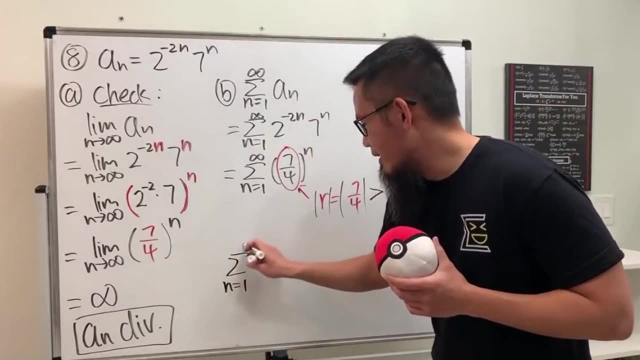 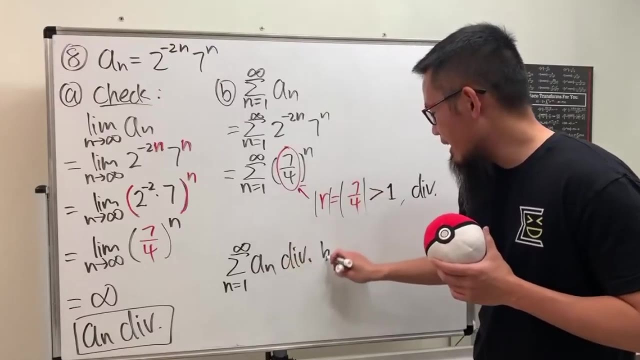 you can write it down like this, no problem at all. Or you could also have said: let me put down two of them. You can say this right here: Okay, Diverges By geometric series test because the absolute value of r is bigger than 1.. 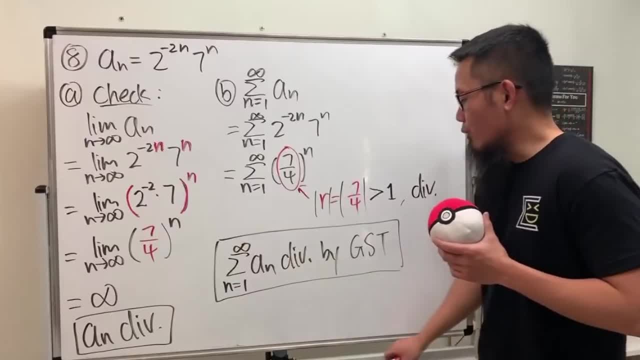 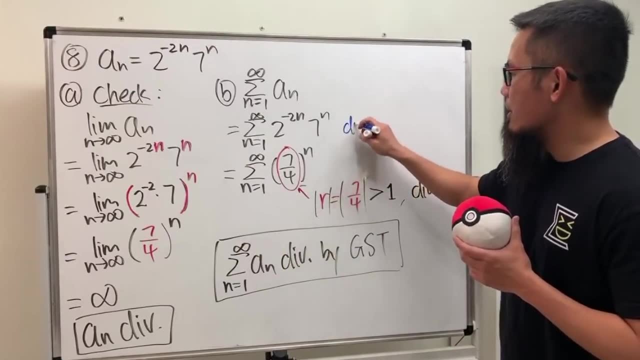 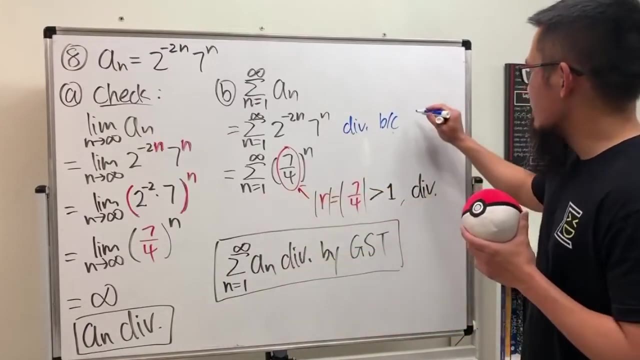 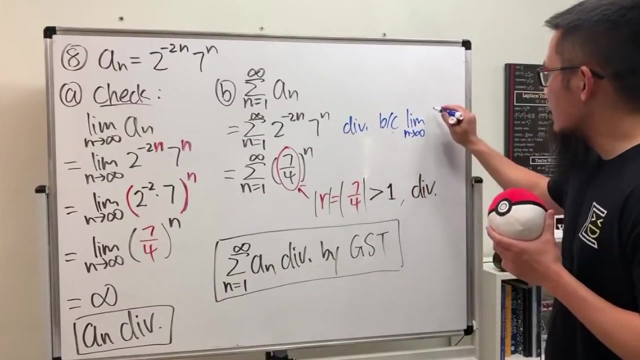 So you can put it down like this, So no problem at all. Or you can also say this right here: diverges because the limit of that- so I'll just say the limit as n goes to infinity, of the 7 over 4 to the n. 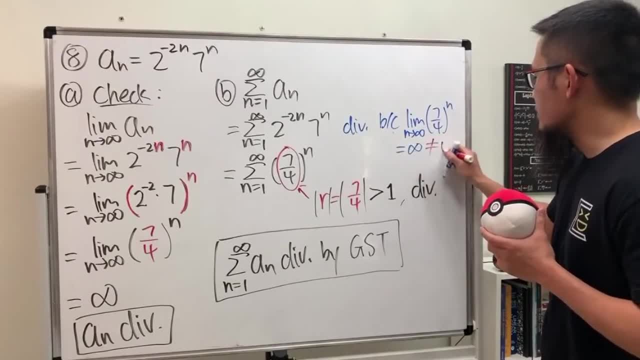 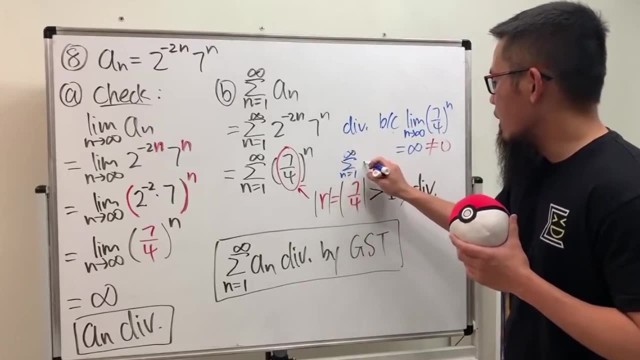 this right here, is equal to infinity, which is not equal to 0.. If you put this down right here, though, then you would just say: the series, as n goes from 1 to infinity of a, n diverges. If you use this. 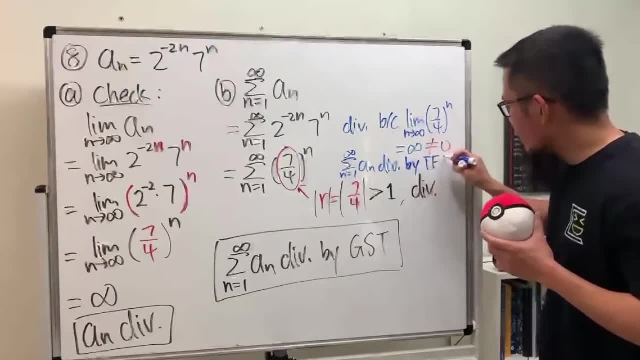 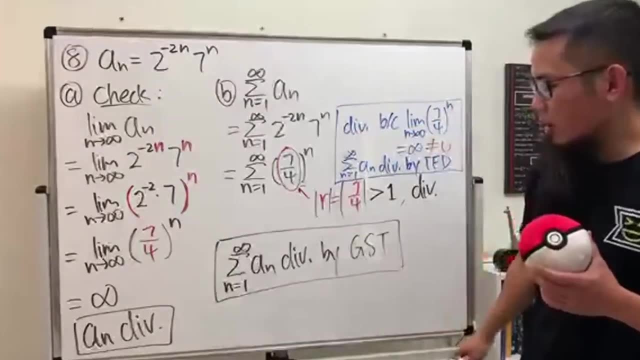 you will have to crawl by test for divergence. Alright, So it depends on which route that you want to take. Yeah, so both are okay. Perhaps this one is better, because we are talking about the geometric series already: 1.6..